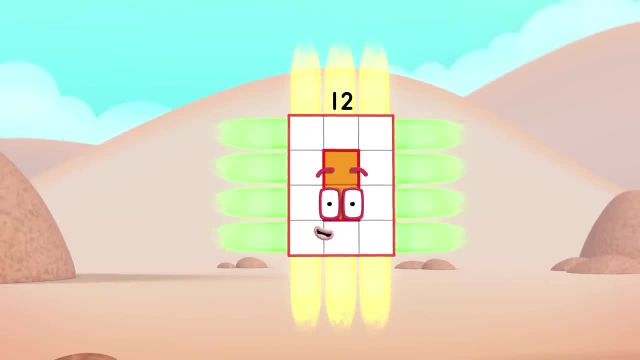 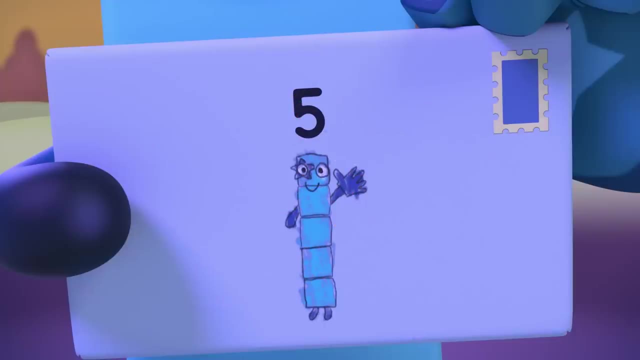 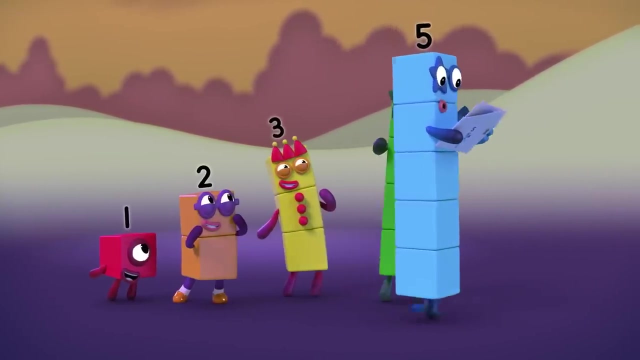 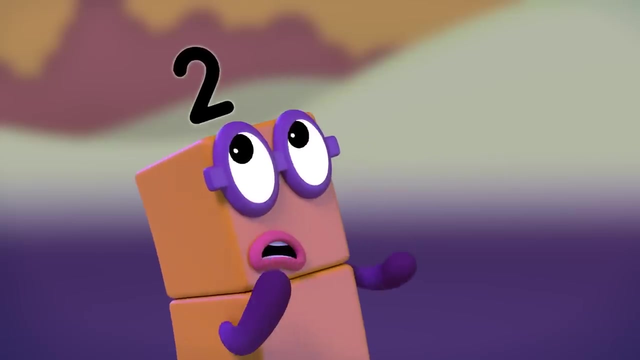 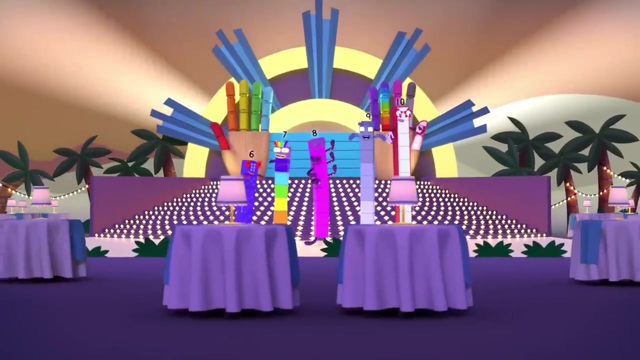 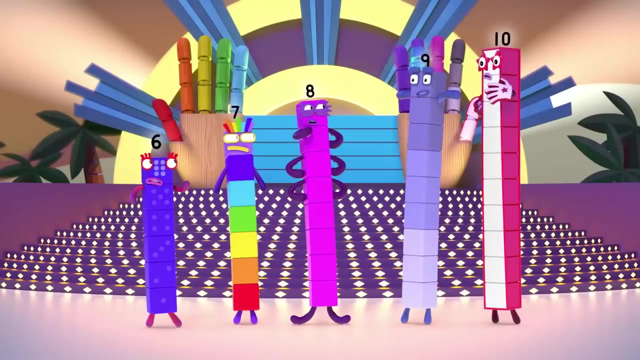 I am a super rectangle. Now, what could this be? Five and friends are invited to a five-star ball at the Two Palms dance floor. I can wear my sparkly headband: The Two Palms. Where's that? Um, Oh Don, Where's five? 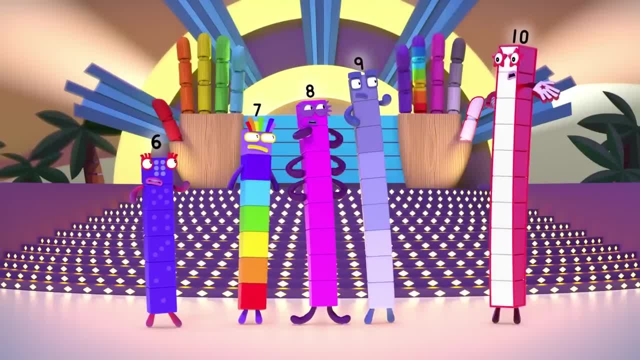 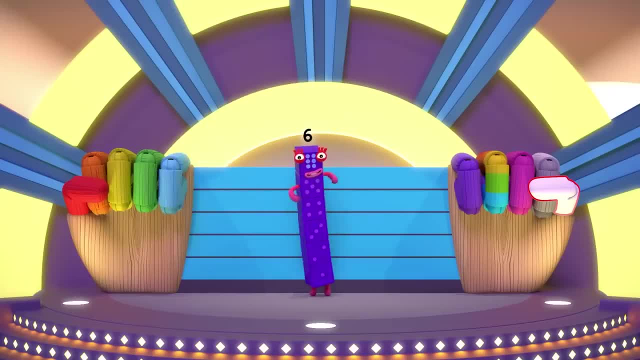 We can't start a five and friends dance without five. Why wait? Just look and you will see that five is here as part of me. Ready, I'm six, I'm five and one, Five and one. I've got a five in me too. 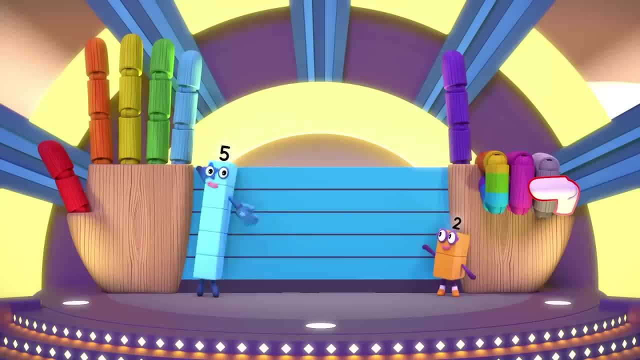 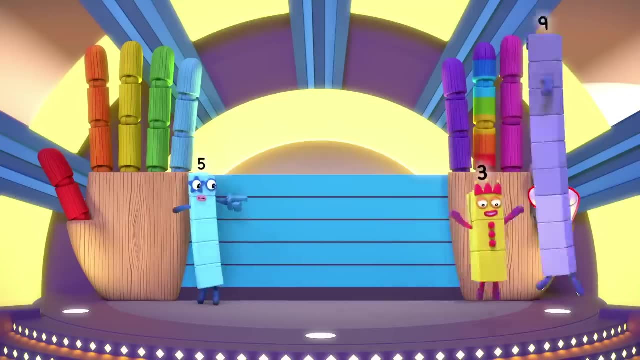 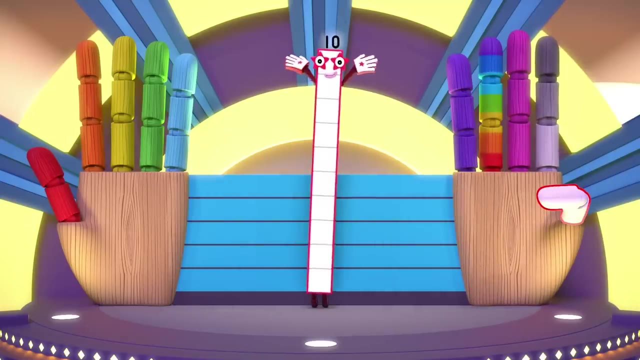 I'm seven, I'm five and two, Five and two, I'm eight, I'm five and three, Five and three, I'm nine, I'm five and four, Five and four And I'm ten. I'm five and another five. 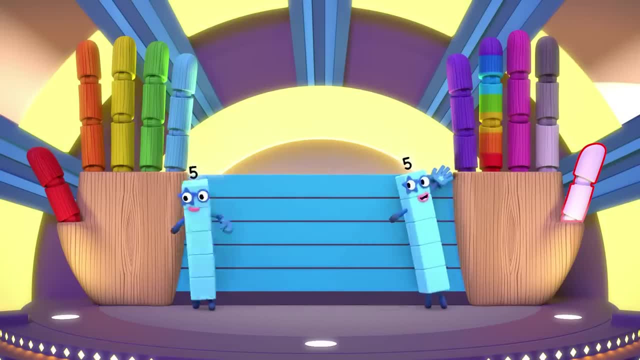 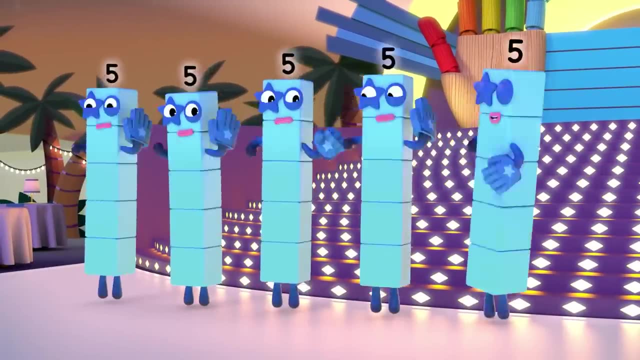 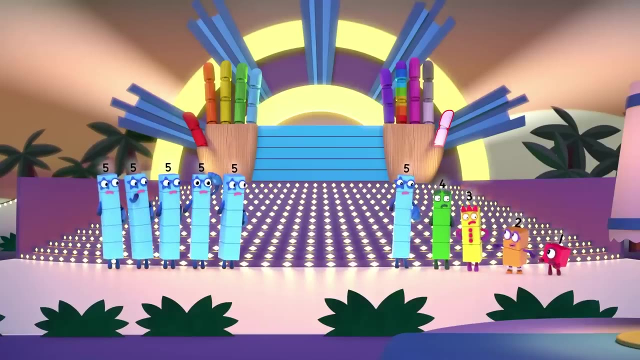 High fives, Five and five. Hey look, five, fives, High five. Ooh, To the side up above, don't know too slow. Yay, Hey, wait. there are loads of fives here now, but we're a six, seven, eight, nine and ten. 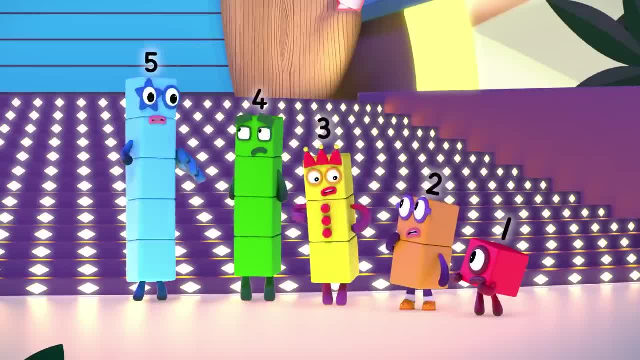 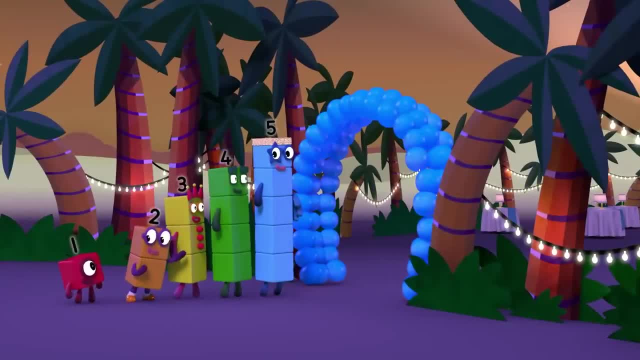 We can't start the dance until all my friends are here. Let's go and find them. Ooh, Wow, This must be the Two Palms. Ooh, Ooh, Wow, And look, five, fives, Ooh. 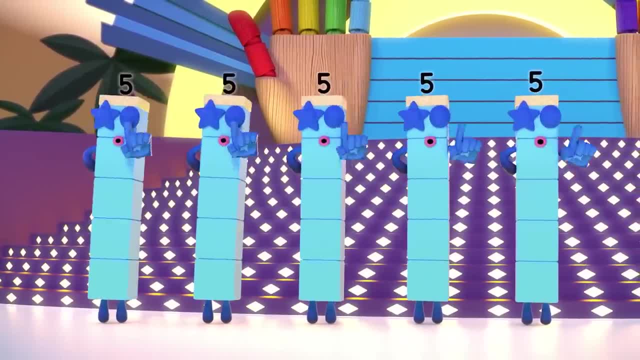 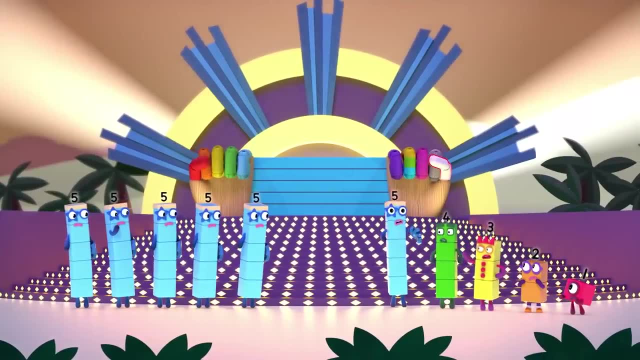 High fives, High fives. Ooh To the side up above, don't know too slow. Wait, wait, wait. Where are six, seven, eight, nine and ten? We can't start until all my friends are here. 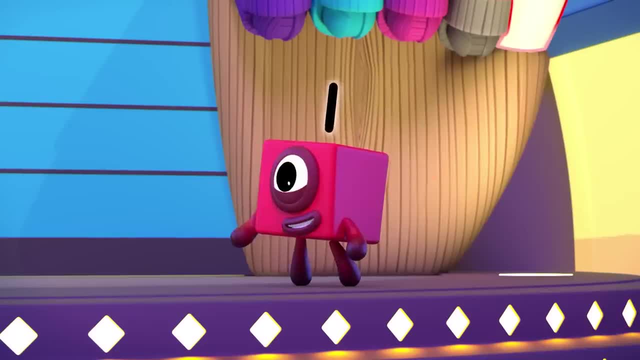 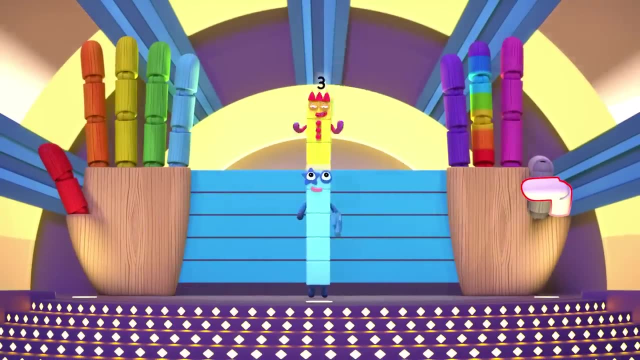 Hey, We can make friends Ready. Five and one is six. Five and two is seven. Five and three is eight. Five and four is nine. High five. Five on another five is ten. Now let's get this party started. 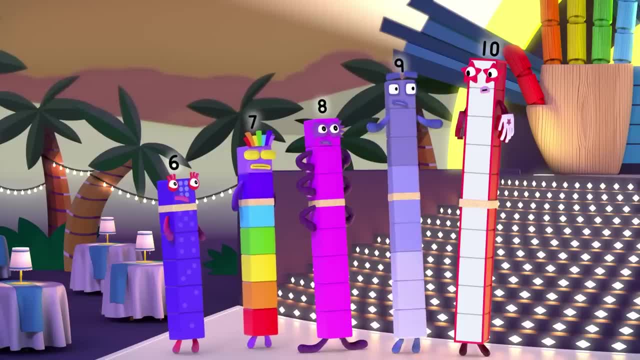 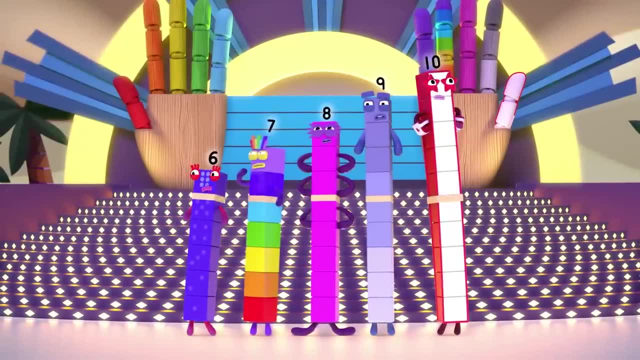 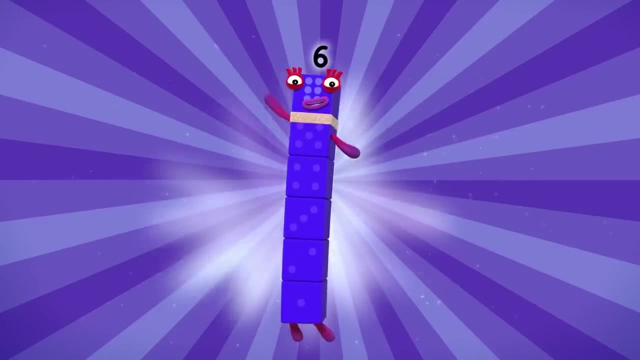 Hold on. We're a one, two, three, four and five. Where are they? Look here, above the sparkly line. Do you see who I see? Ready. I'm six, I'm five, I'm one, I'm seven. 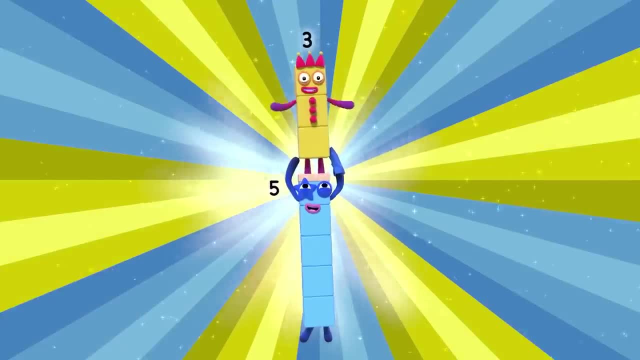 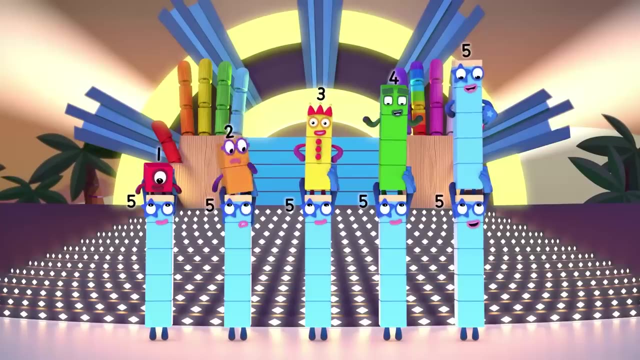 I'm five, I'm two, I'm eight, I'm five, I'm three, I'm nine, I'm five and four, I'm ten, I'm five, on another five, High five. Hey, wait, Where are six, seven, eight, nine and ten? 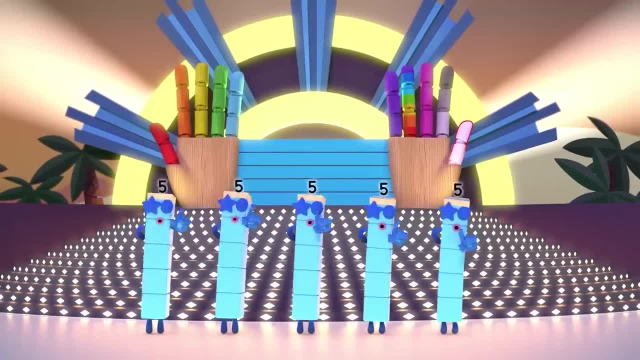 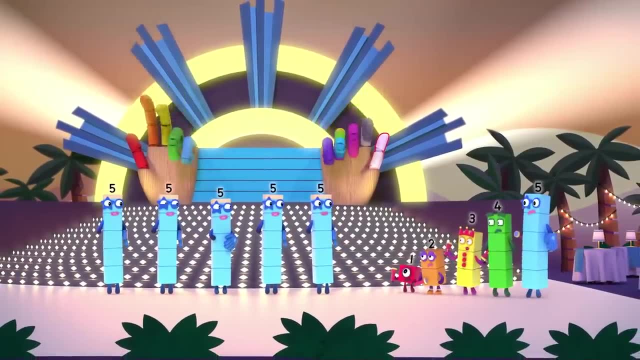 Let's go and find them. High five: Ooh To the side. Oh, don't go too slow. Oh here, Where are six to ten? Jump up here, You'll see them then. Ready Five and one is six. 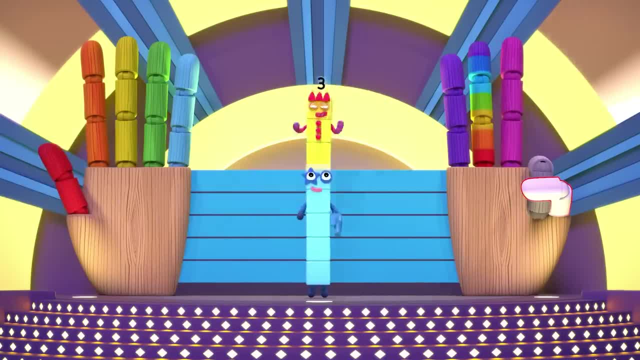 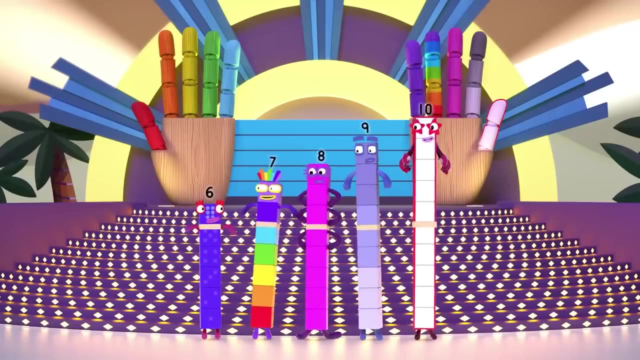 Five and two is seven. Five and three is eight. Five and four is nine. High five, Five and another five is ten. Now let's get this party started. Hold on, Where are one to five? One, two, three, four? 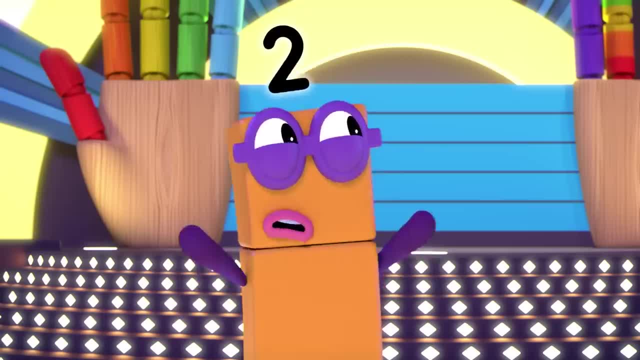 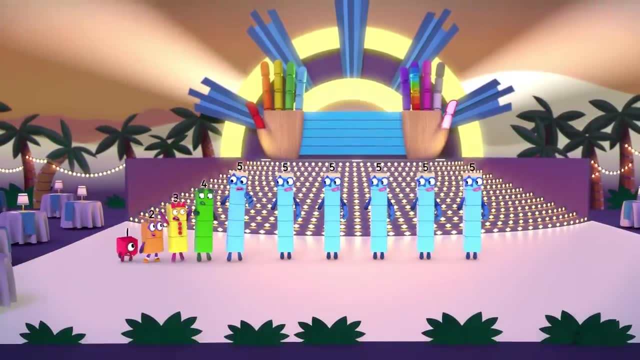 Five and another five. High five. Hey wait, Where are six to ten? Let's go look for them again. High five. Ooh, Where are? where are six to ten? Why don't you jump up again? Six, seven, eight, nine. 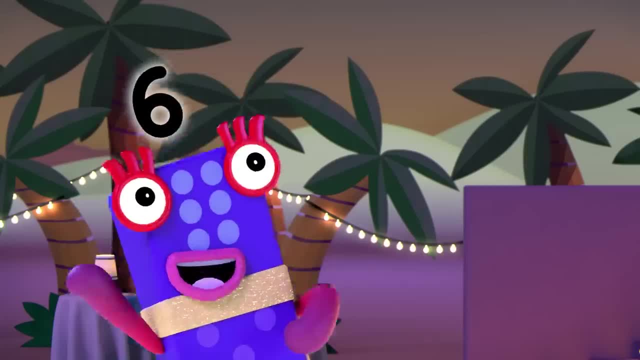 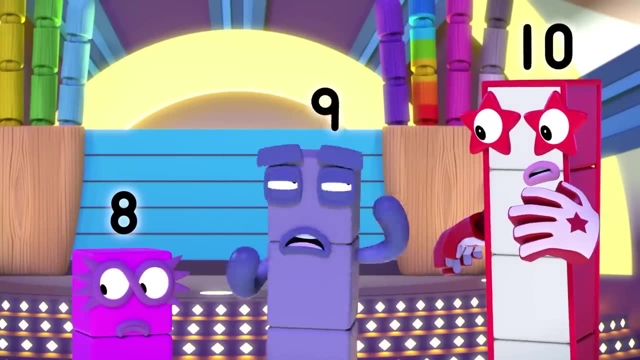 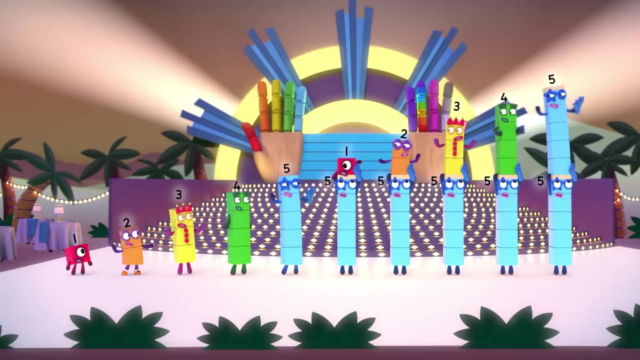 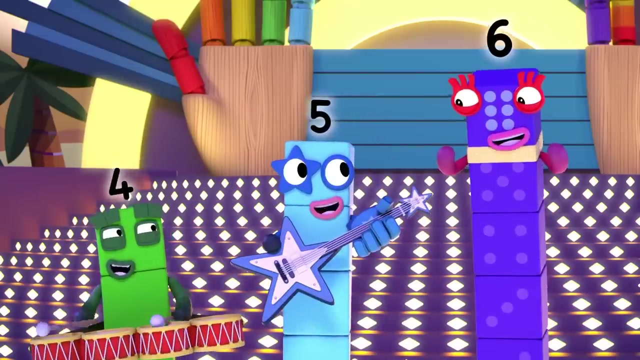 Five and another five is ten. Let's get this party started. Hold on, Where are one to five? There we are. Well, where are? where are six to ten? Here we are. My friends are all here. Let's Get this party started. 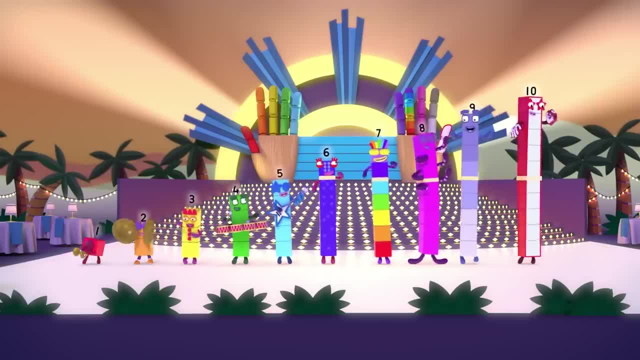 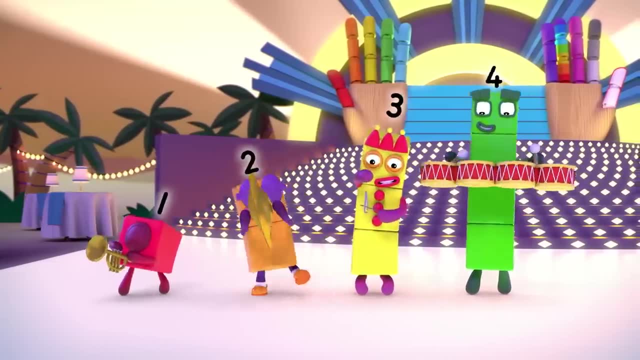 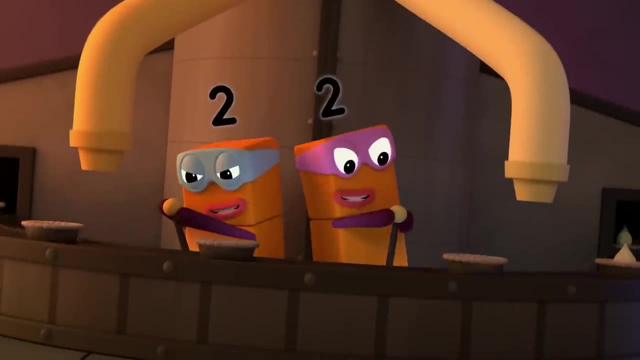 Let's get this party started. Let's get this party started. High five, Ooh. To the side Up above. Don't low Too slow. High five Ooh. Surprise, surprise, Custard pies Ooh. 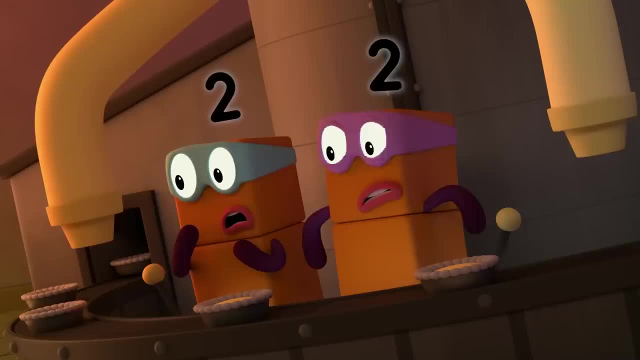 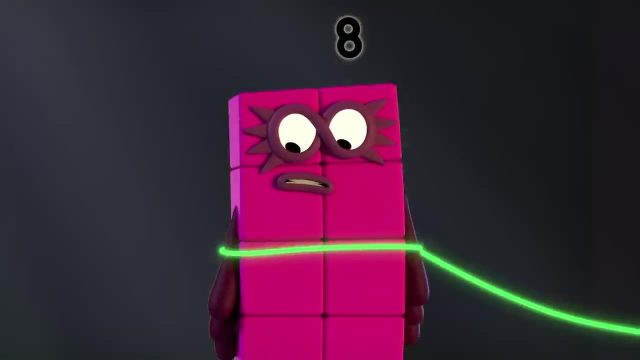 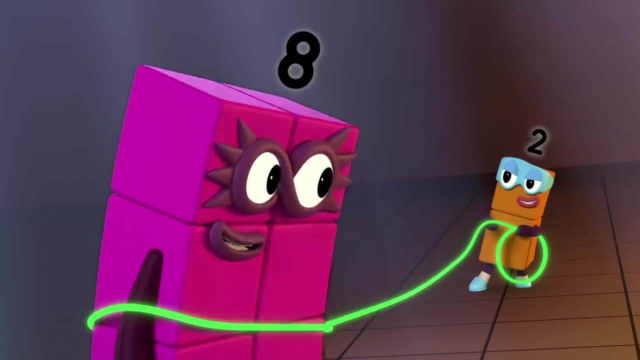 Your days of naughtiness are numbered terrible. twos, One, two, three Got you Octoblock Break Rope. That rope is made from pure octonite. Your powers are useless? Maybe so, but I can still do this. 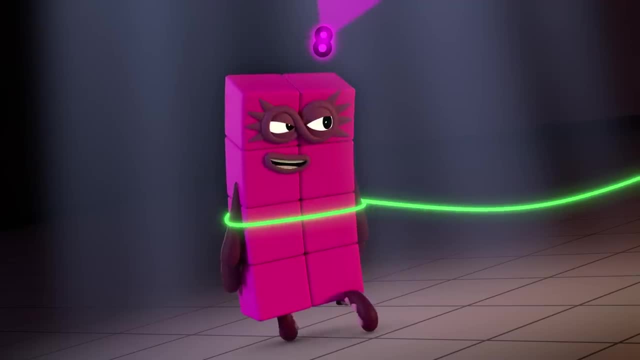 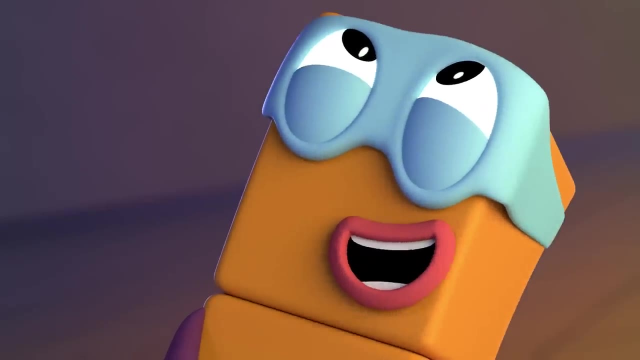 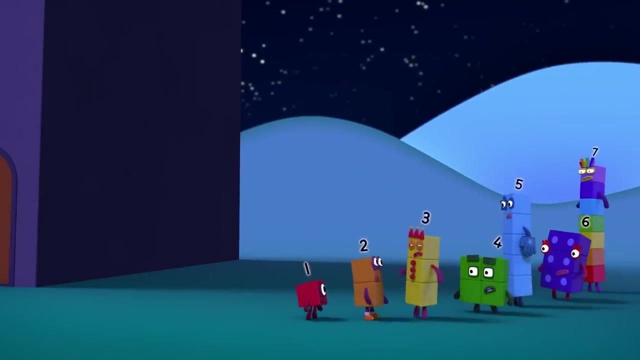 The Octo-Signal. My friends will be here any moment And they will fall straight into our troublesome traps. Mwa-ha-ha-ha-ha-ha, Don't be so sure. Octoblock leads us Splitter. 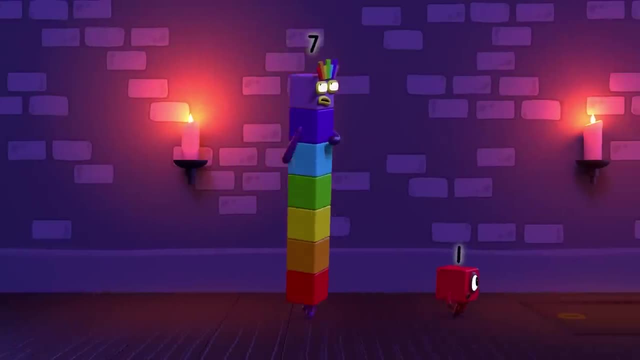 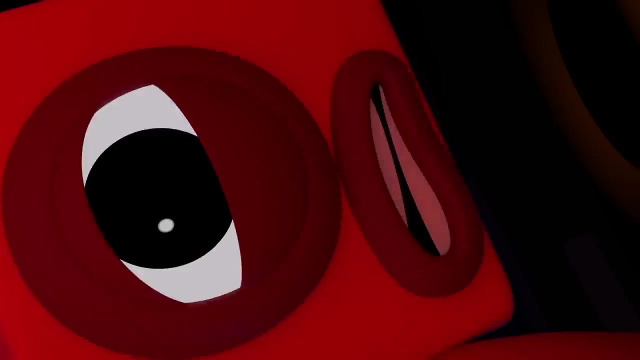 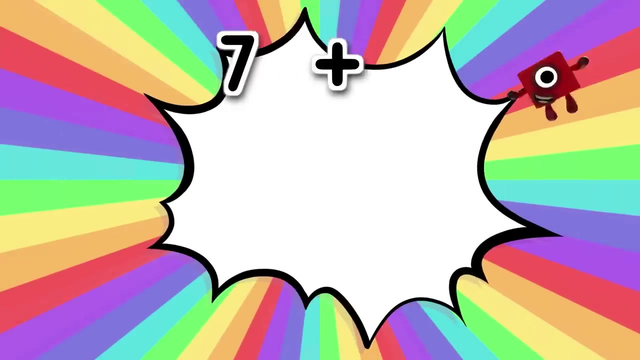 In here: Whoa Ow, Oh, Oh. Oh, That wasn't very lucky, Ah, But that was Seven. One Equals Eight. Octoblock leap: One, two, three, four, five, six, seven, eight. 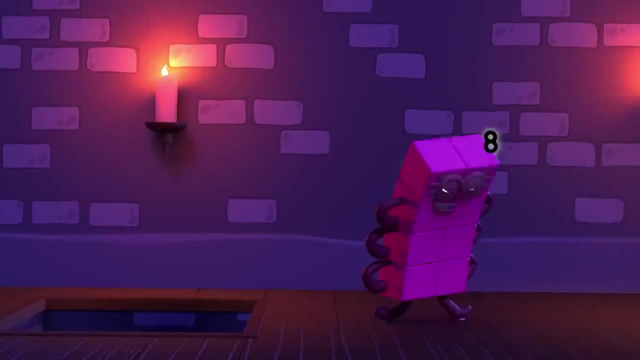 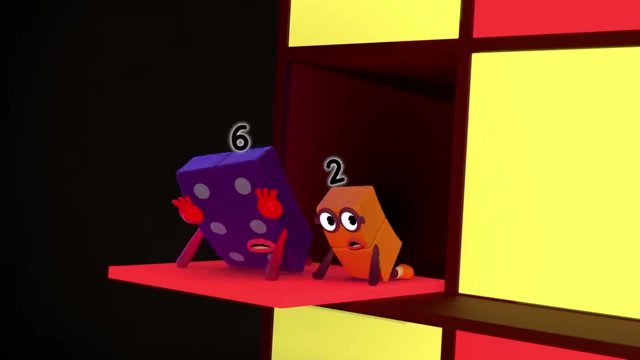 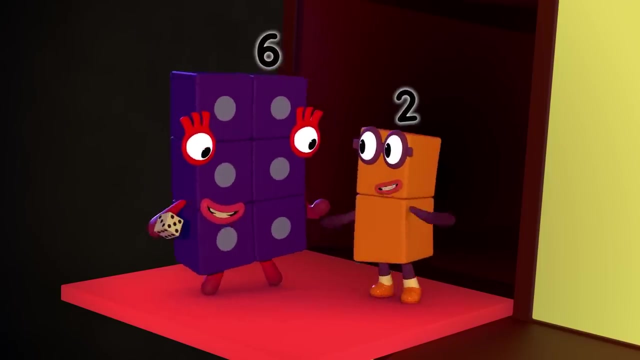 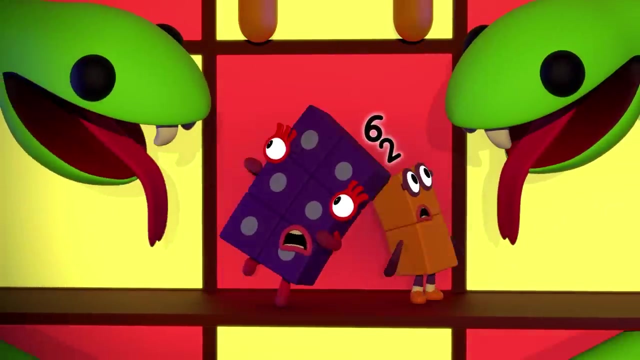 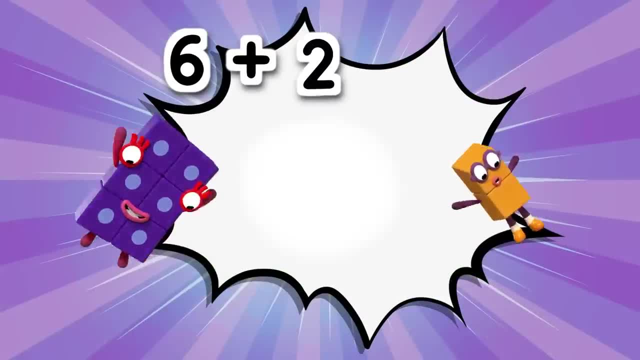 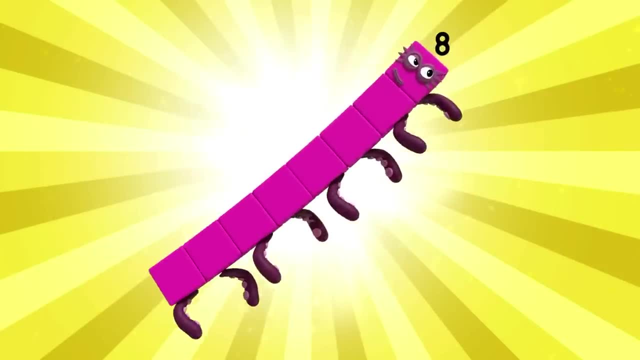 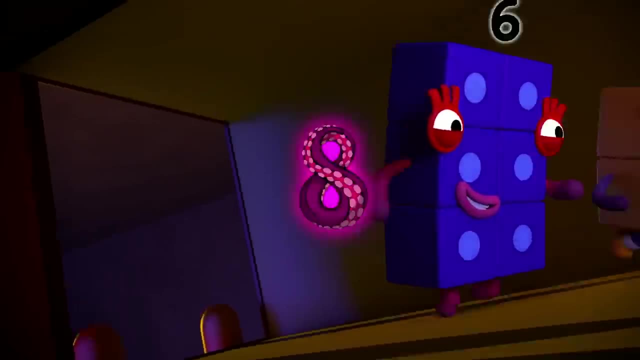 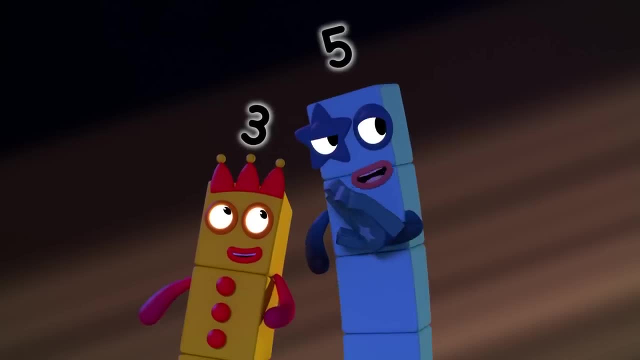 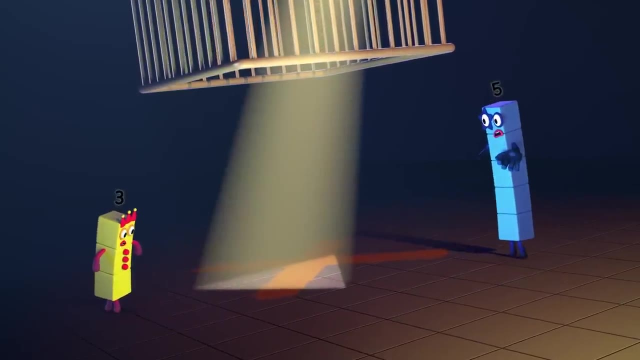 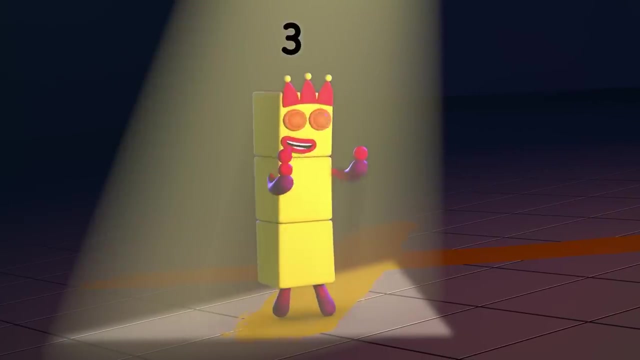 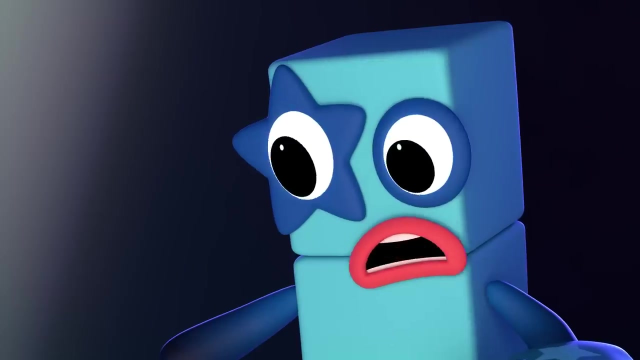 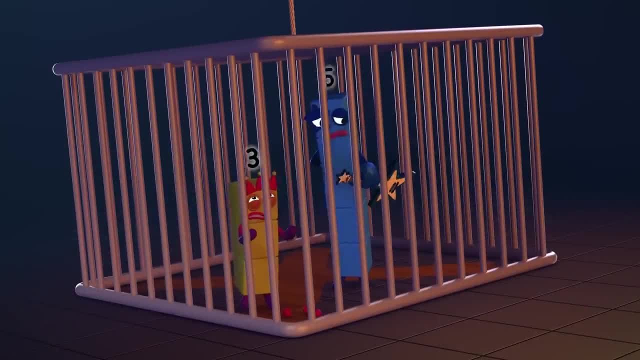 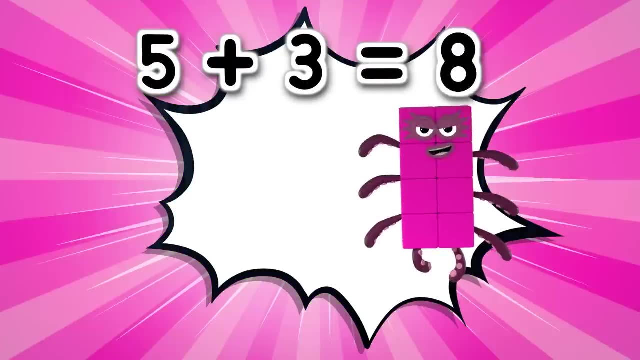 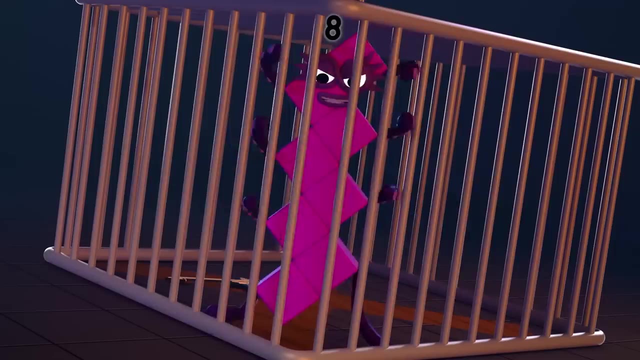 Ah, Ah, Hey, I wasn't finished. Grand finale: Five plus three equals Eight. Huh, Octoblock ten. One, two, three, four, five, six, seven, eight Burn, Ah, Ah. 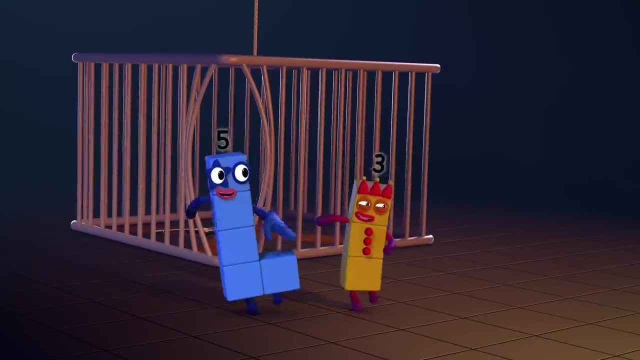 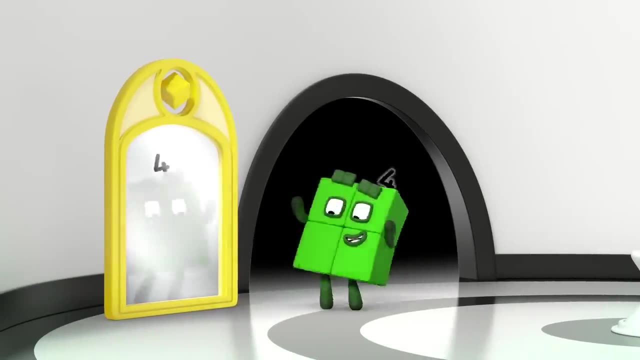 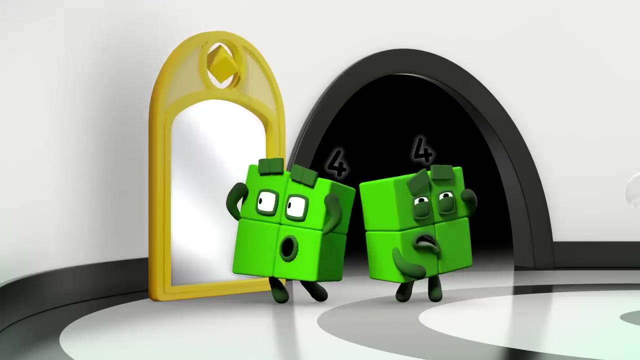 Ah, Ah, Ah, Oh, Oh, Oh, Oh, Hello, Hello, Ooh, Round things, It's got us. Ah, Four plus four equals Eight. Four plus four equals Eight. Four plus four equals Eight. 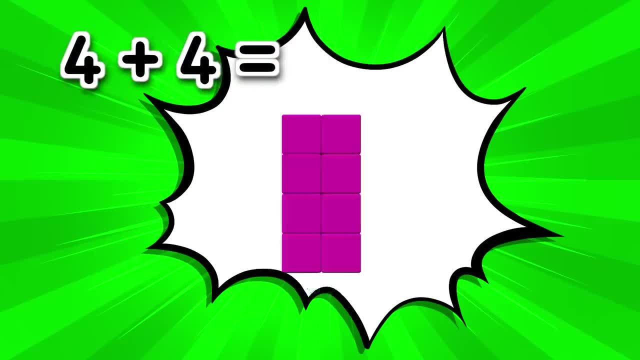 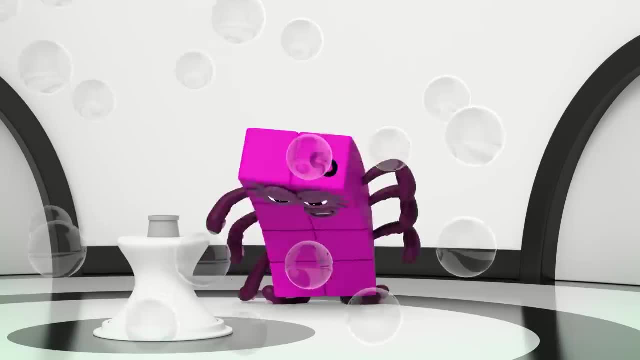 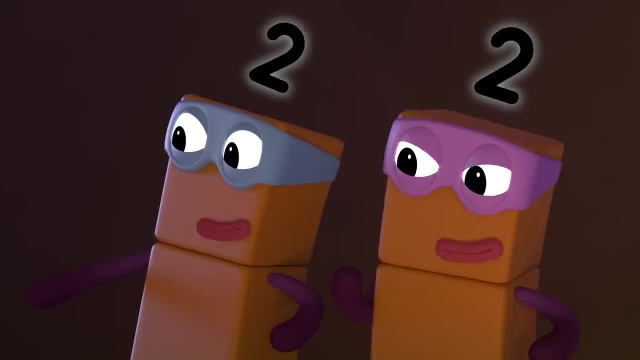 Eight, Four, Four, Four, Eight. Octoblock pop One, two, three, four, five, six, seven, eight Pop. Huh, Prepare to be pied Spiderblock. Ha-ha, Stop right there. 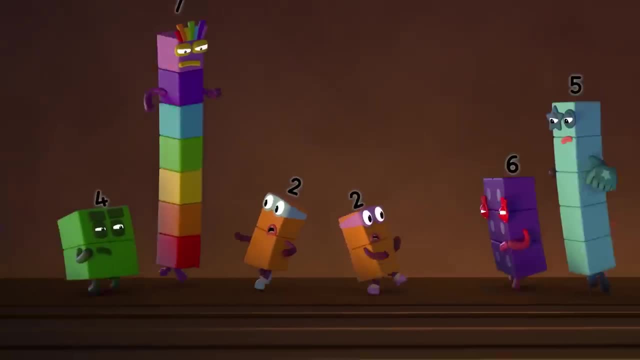 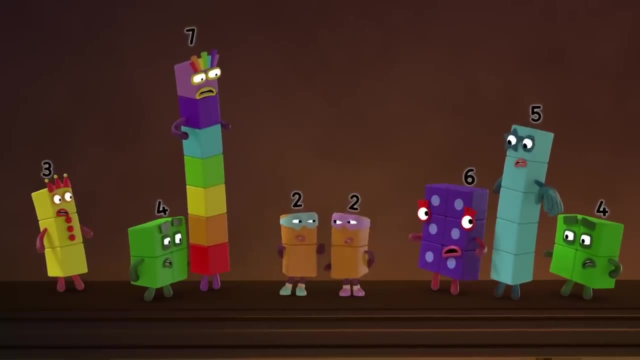 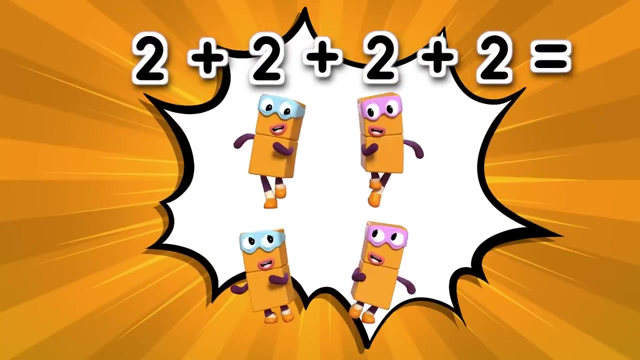 We have you outnumbered? Ooh, Ah-ah, Ha-ha, Ha-ha. Maybe so, But we've still got a trick or two up our sleeves. Two plus two plus two plus two equals eight. Oh, four terrible twos make one Octonauty. 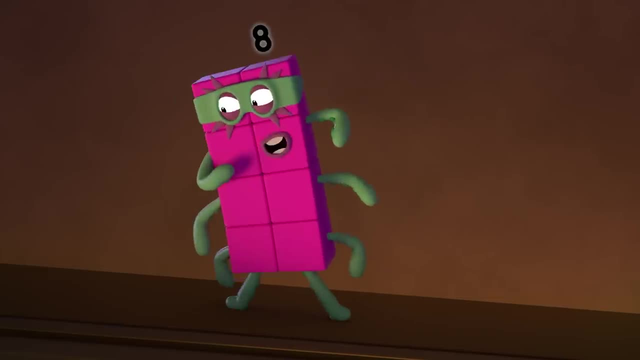 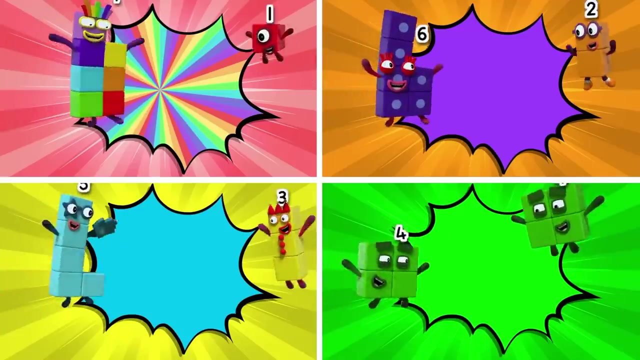 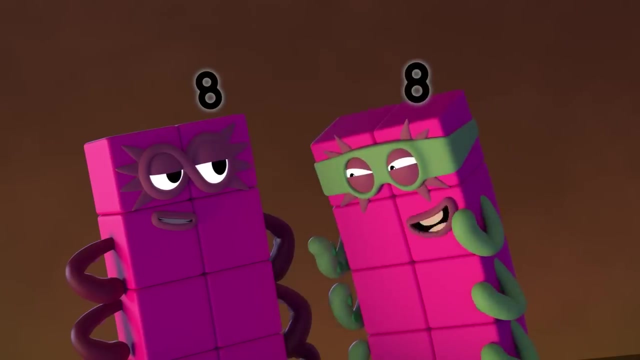 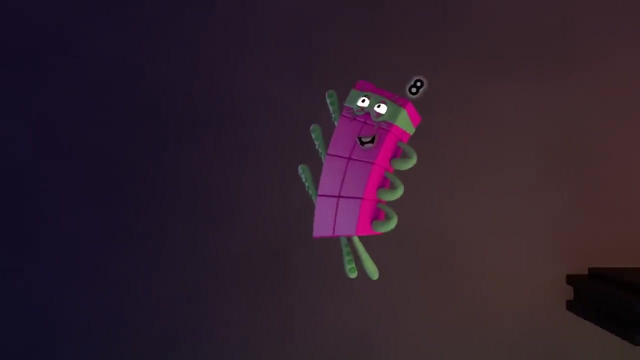 You've met your match, Octoblock, Don't count on it. Octoblocks assemble. Your number is up. You'll have to catch me first. Octonauty escape. Eight, seven, six, five, four, three, two, one escape. 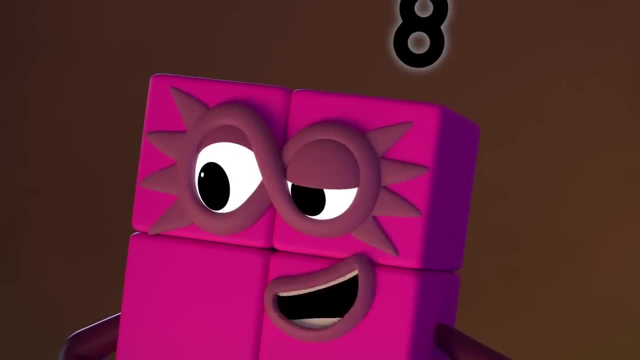 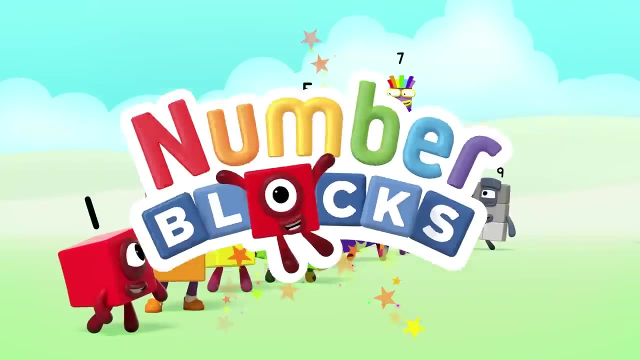 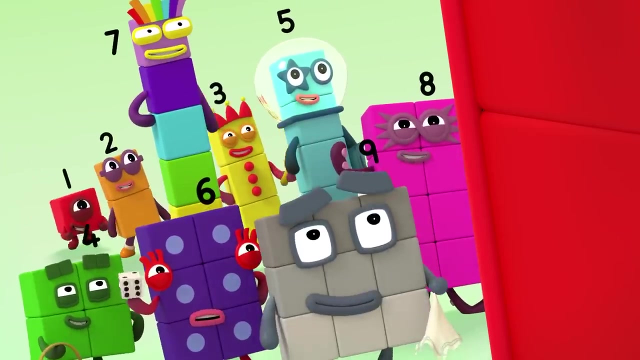 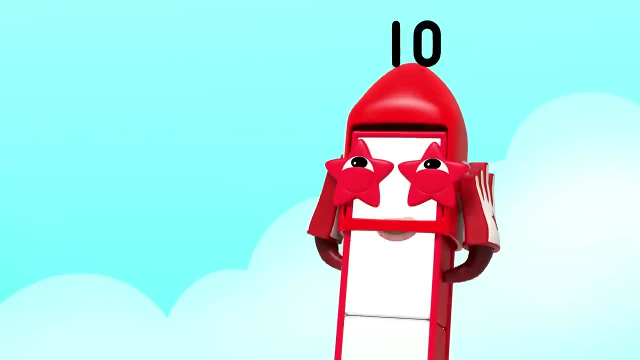 Uh-oh, I spy with my little pie. a very naughty number block Ha-ha-ha. What shall we do today? What shall we do today? I say please, please, Oh, OK, Let's do everything, Everything. 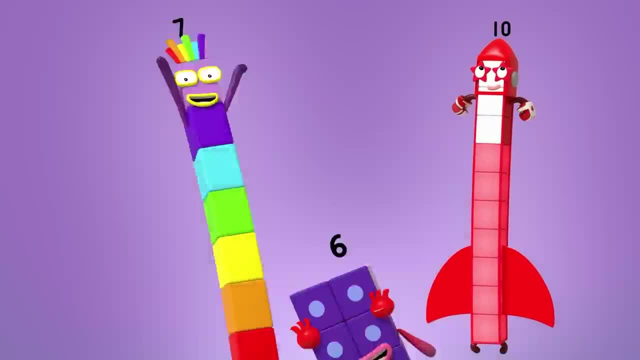 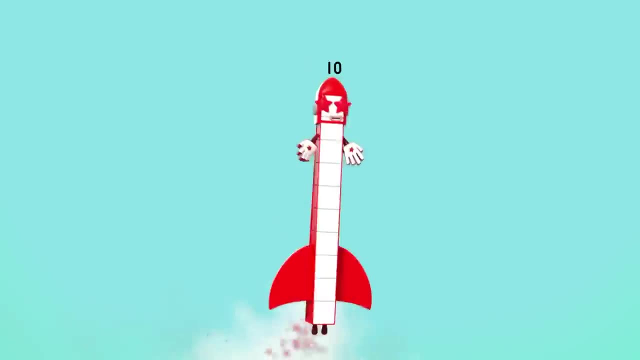 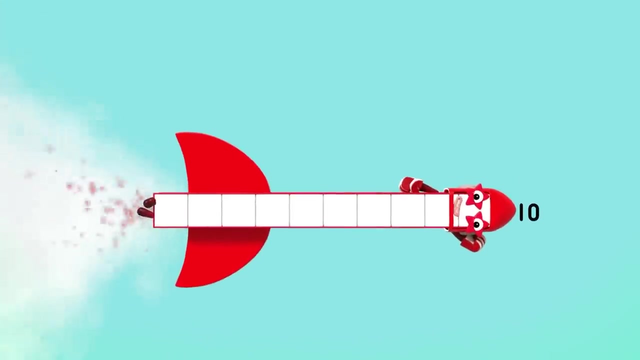 Yes, Ready. Ten, nine, eight, seven, six, five, four, three, two, one Blast off. I'm ten, ten, ten, and I'm flying through the sky. I'm ten, ten, ten. you can break me up any way you like. 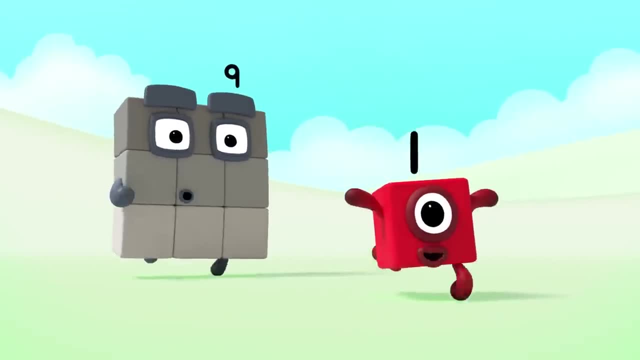 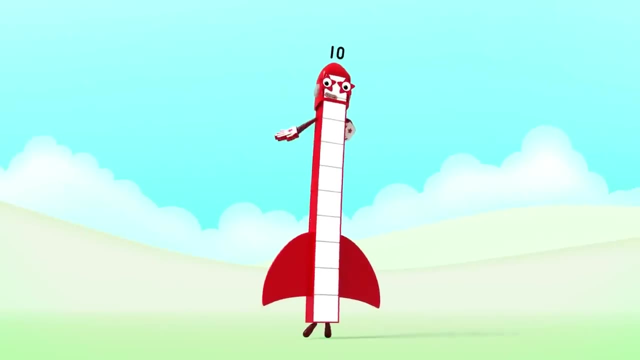 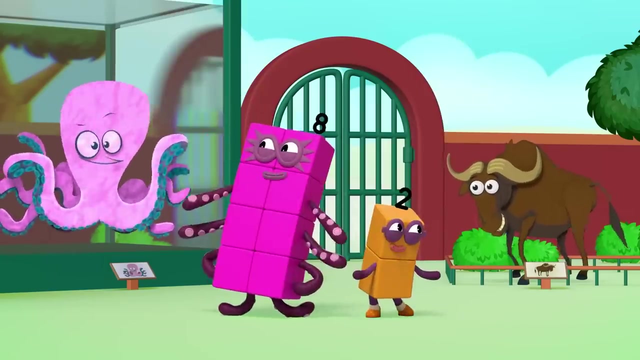 I can be Nine plus one going for a run, trying not to sneeze And having lots of fun. And then I'm ten, ten, ten again. I can be Eight plus two visiting the zoo, Talking to the octopus. 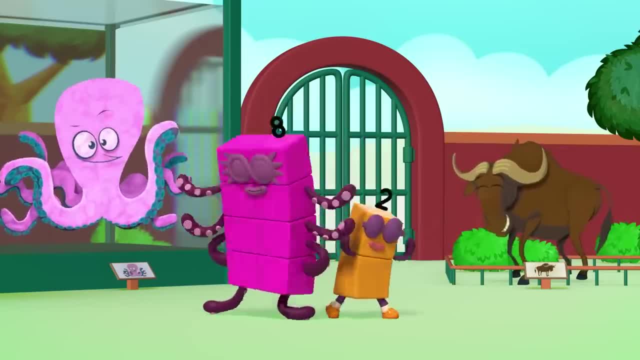 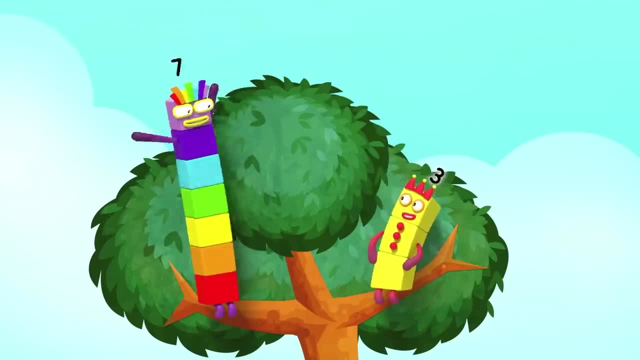 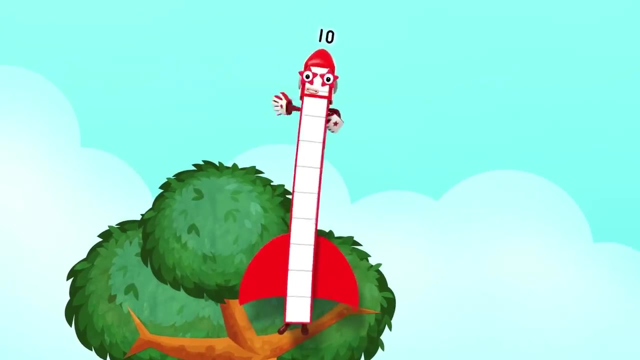 And dancing with a canoe. And then I'm ten, ten, ten again. I can be Seven plus three sitting in a tree Making rainbows And looking at me. And then I'm ten, ten, ten again. 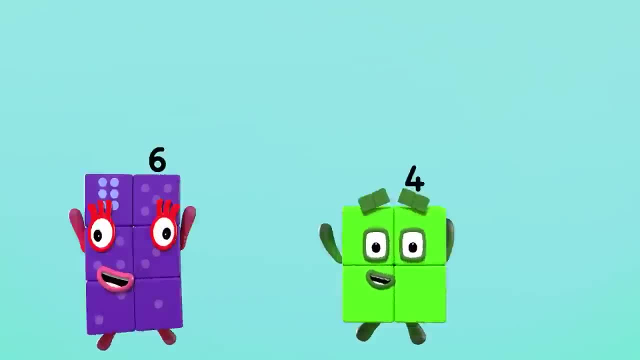 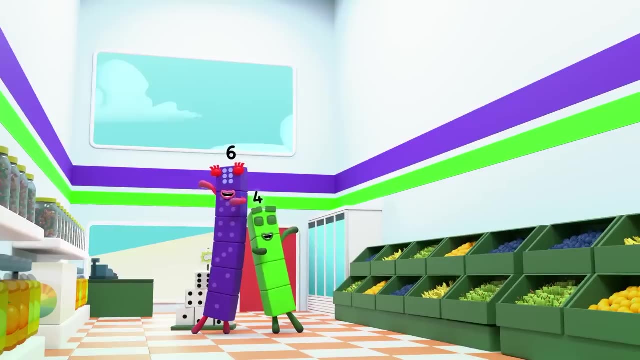 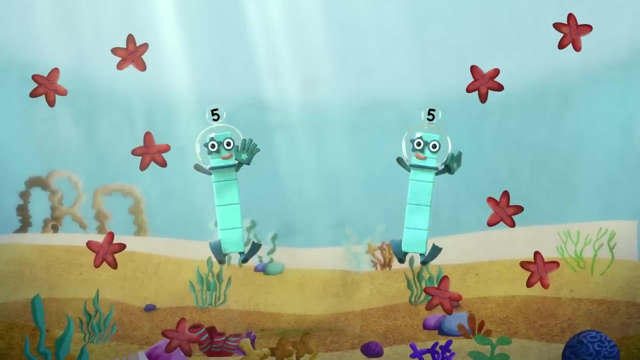 I can be Six plus four shopping at the store, Playing with a dice On a square tile floor, And then I'm ten, ten, ten again. I can be Five plus five on the skua dive, Swimming with a starfish and doing a jive. 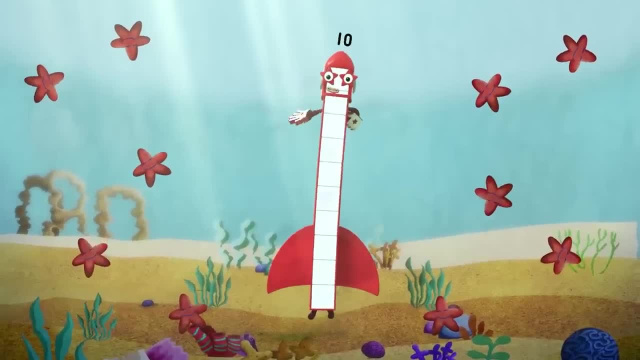 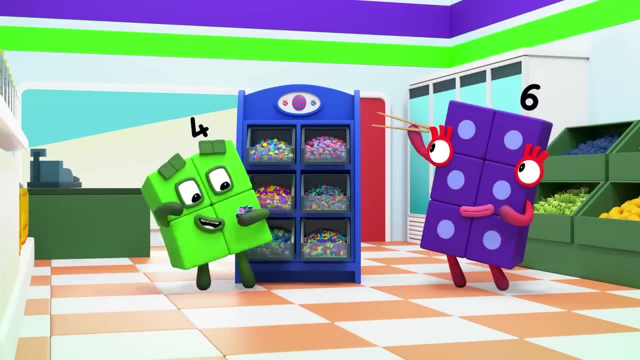 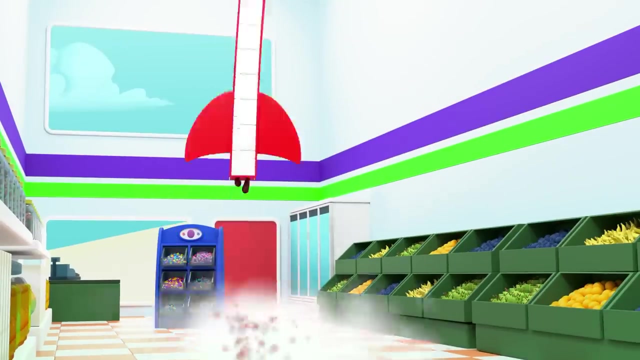 And then I'm ten, ten, ten again. I can be Four plus six, buying pick and mix, Picking out the square ones And using chopsticks. And then I'm ten, ten, ten again I can be. 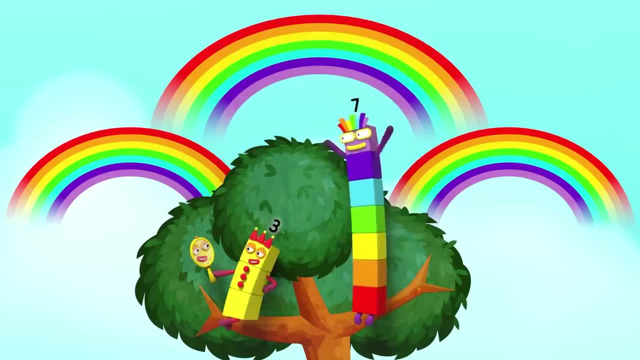 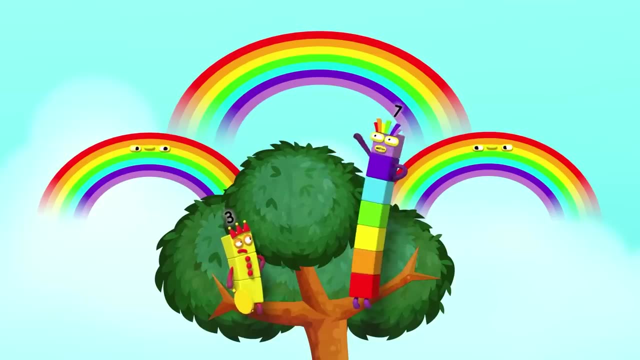 Three plus seven, gazing up to heaven- No, looking at me- And a rainbow called Kevin. Kevin, And all my rainbows have names: Kevin, Rainbow, Dina, and that's Big Bob, Hello. And then I'm ten, ten, ten again. 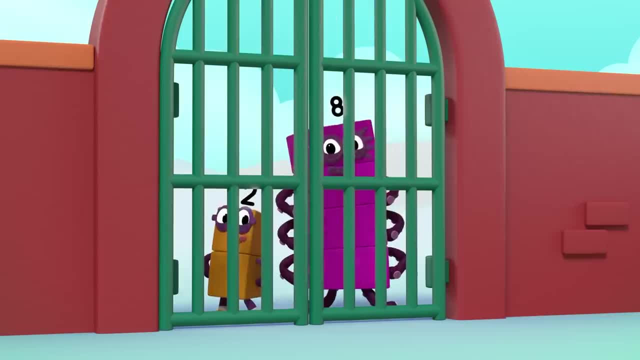 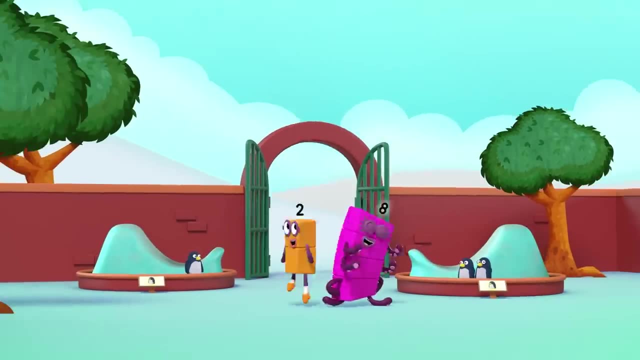 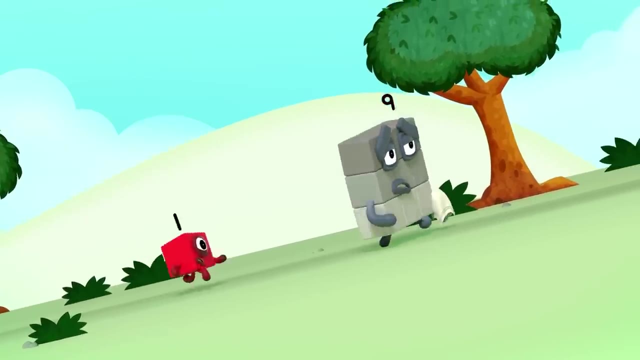 I can be Two plus eight, opening a gate, Dancing with a penguin Lifting heavy weights, And then I'm ten, ten, ten again. I can be One plus nine, starting on a climb, Getting out of breath now. 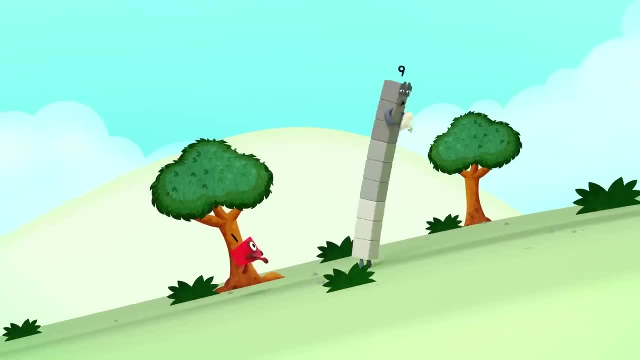 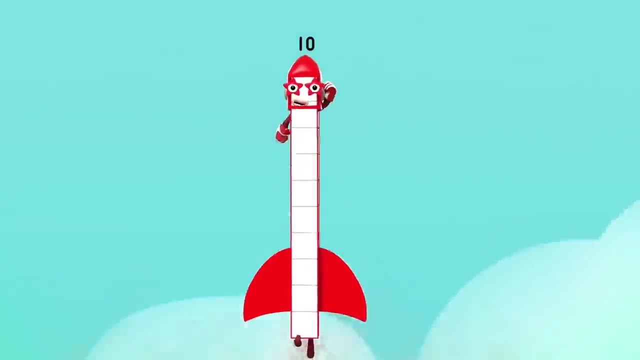 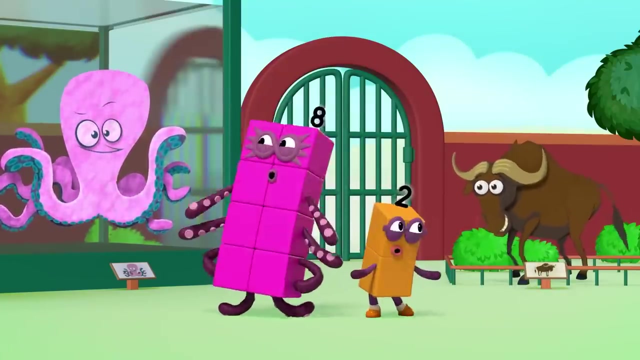 Sneezing all the time. And then I'm ten, ten, ten again, Ten, ten, ten again Again. Nine plus one going for a run, Eight plus two visiting the zoo, Seven plus three sitting in a tree. 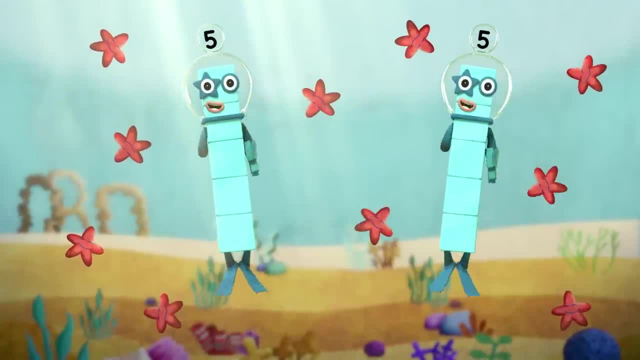 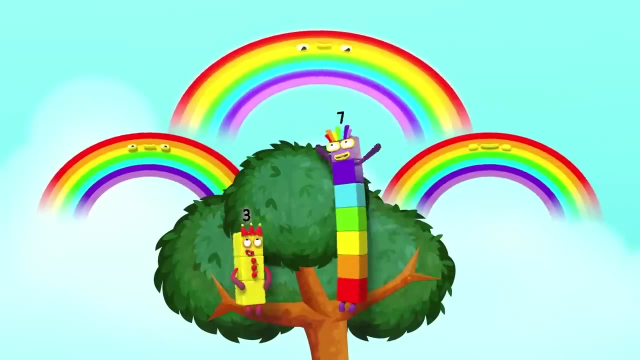 Six plus four shopping at the store. Five plus five on a scuba dive. Four plus six buying bigger mix. Three plus seven gazing up to heaven. Two plus eight opening a gate. One plus nine starting on a climb. 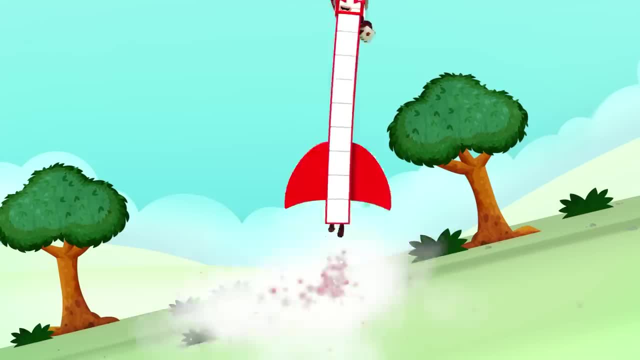 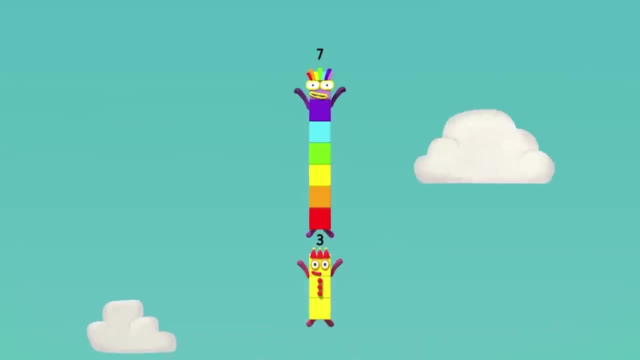 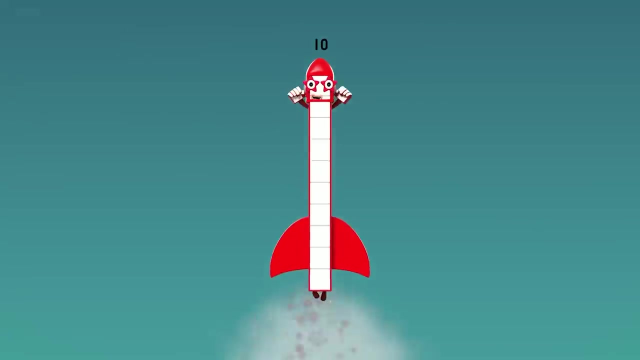 And then I'm ten, ten, ten again Again. Nine plus one, ten again, Eight plus two, ten again Seven plus three, ten again, Six plus four, ten again, Five plus five, ten again Four plus six, ten again. 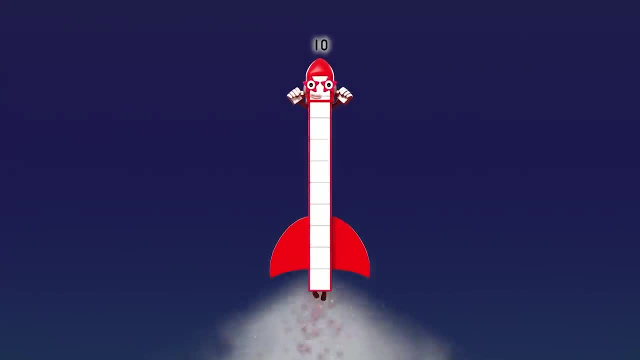 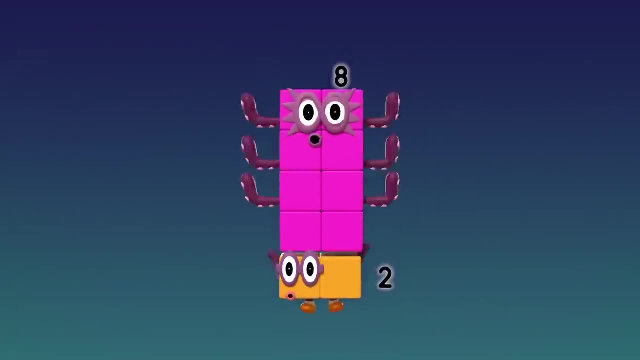 Three plus seven, ten again Two plus eight, ten again One plus nine, ten again Ten, when ten again Nine plus one, ten again Eight plus two, ten again Seven plus three, ten again Six plus four, ten again. 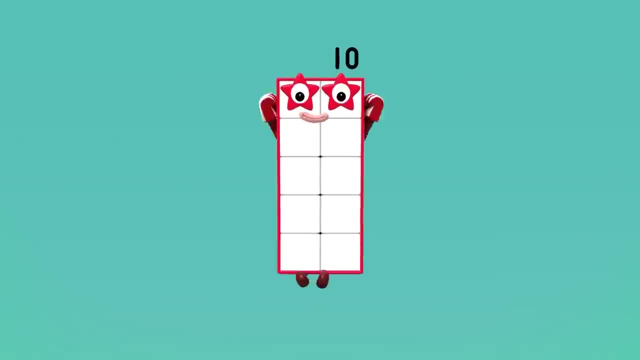 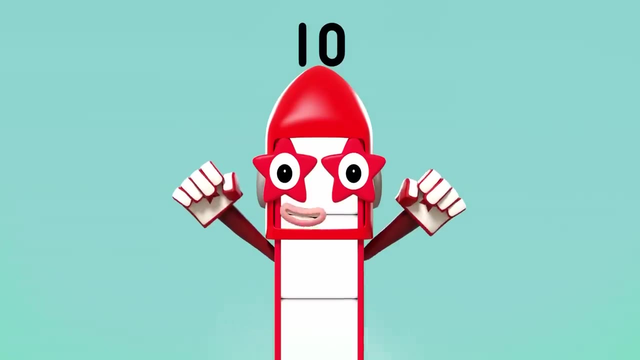 Five plus five, ten again Four plus six, ten again Three plus seven, ten again Two plus eight, ten again One plus nine, ten again Ten, ten, ten again Again Nine plus one, or one plus nine. 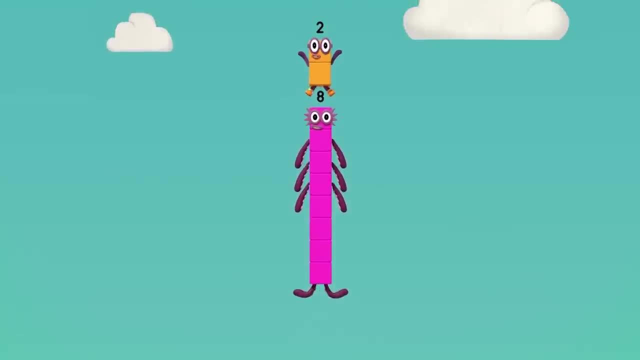 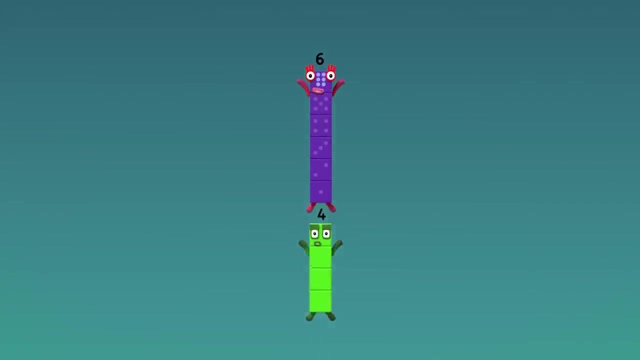 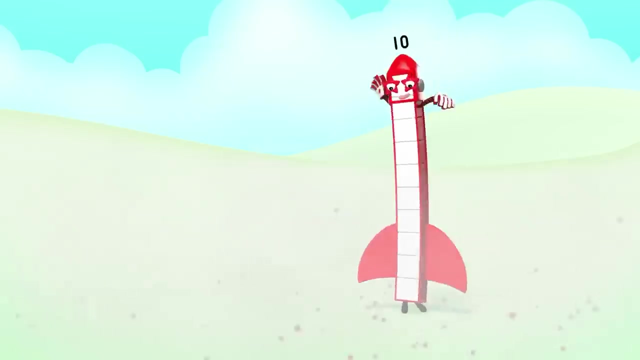 Ten Eight plus two or two plus eight, Ten, Seven plus three or three plus seven, Ten, Six plus four or four plus six, Ten, Five plus five or five plus five, Ten, Ten, ten, ten again. 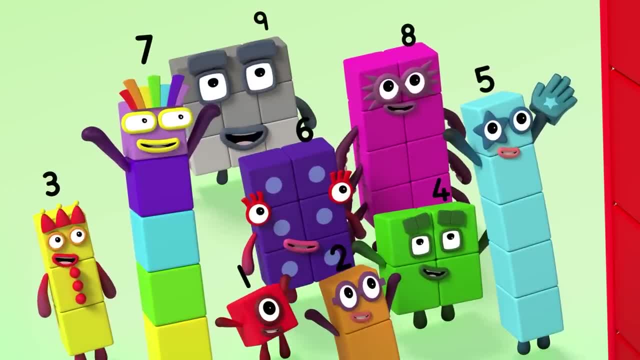 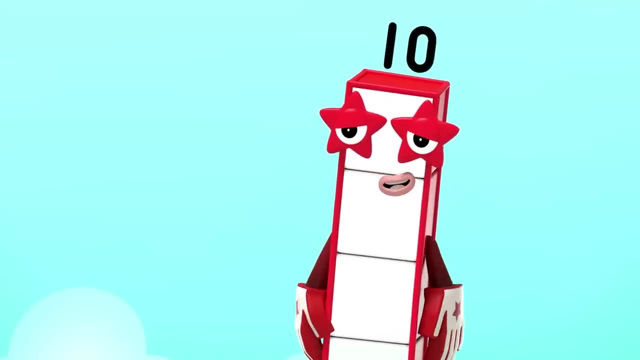 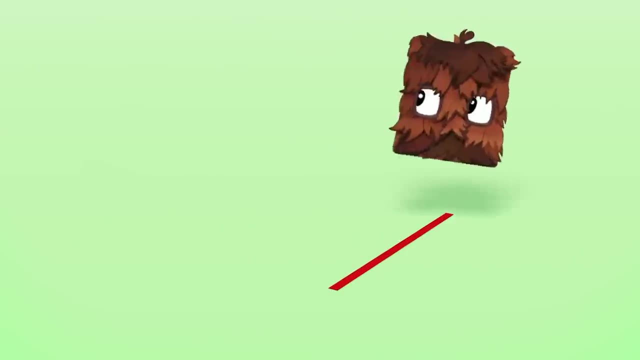 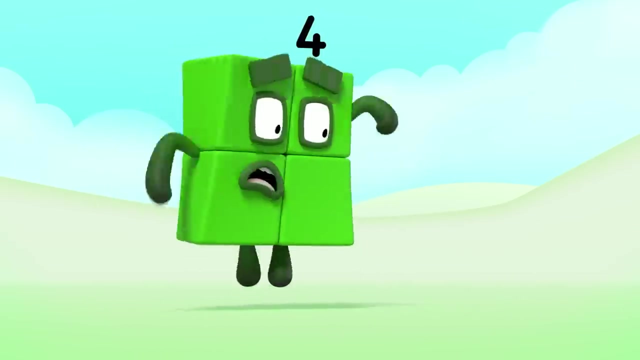 Ten, ten, ten again, Ten, ten, ten again. And what do you want to do today? Ten, I need a nap. What is it Squeary? Ooh, a stick Fetch. Hey, wait for me. 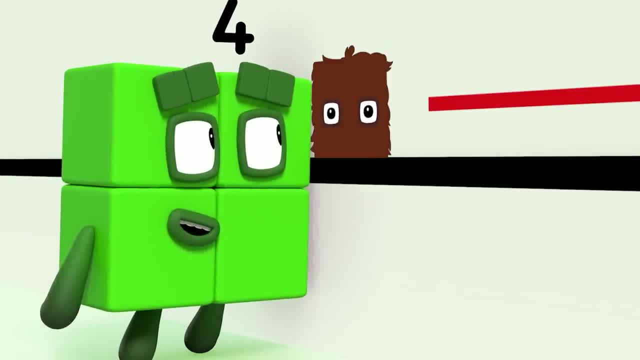 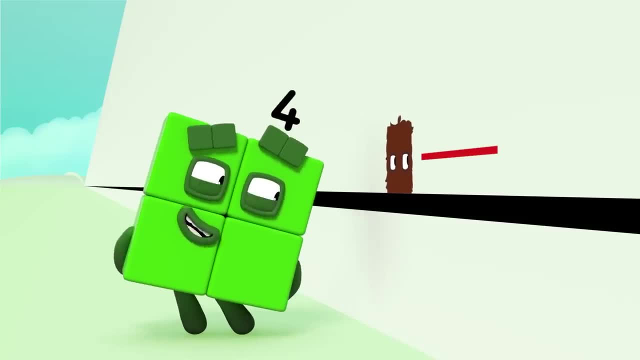 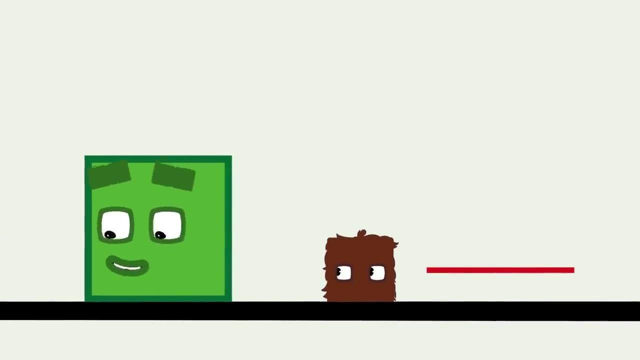 Squeary. Oh, you've gone all flat. Ooh, that looks like fun. Hey, I'm all flat too. I'm a square, A real square. Ooh, Squeary, I've a feeling we're not in Numberland anymore. 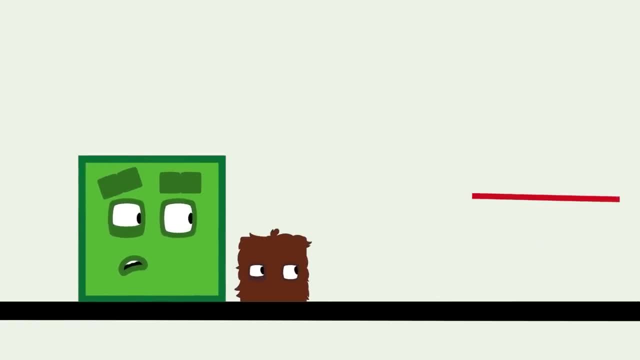 Welcome to Flatland, where all the flat shapes live. I am a line, One straight line, Two straight lines, And when three lines join together, we make Bum, bum, bum, A triangle. I've got one, two, three. 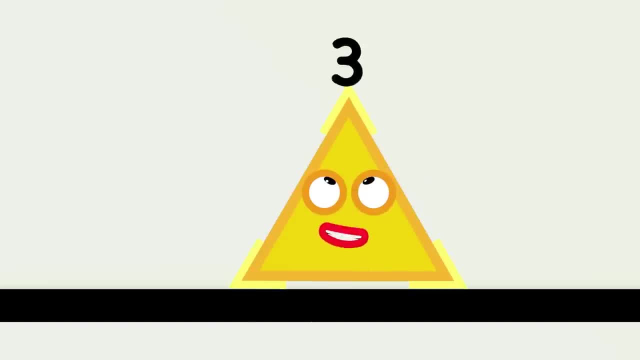 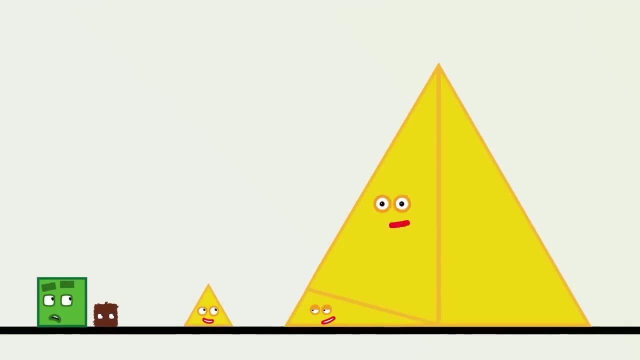 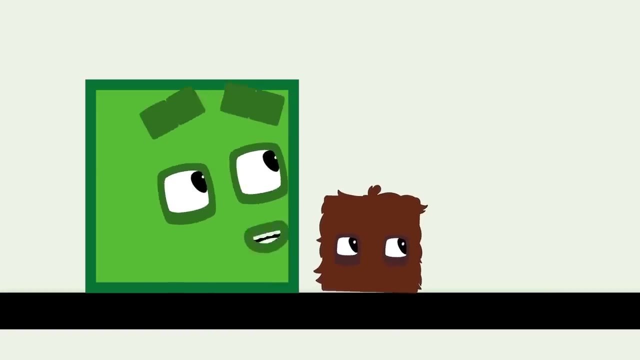 Three sides And one, two, three, Three corners. Look at me, Ooh And me, And me And me. We're all triangles, Wow, But you're all so different. Ooh, Squeary, come back. 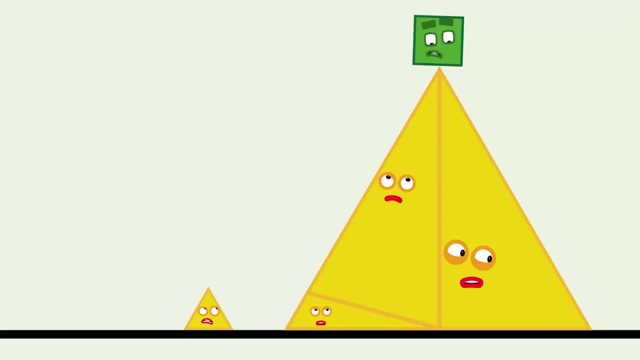 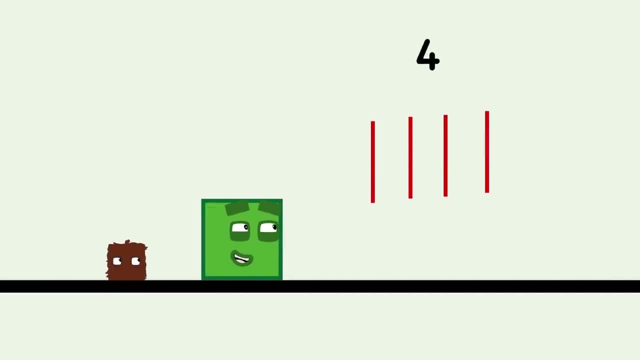 Ooh, ooh, ooh, Sorry, sorry, sorry, Really sorry, sorry. Ooh. One, two, three, four, Four lines: Hello, square. Huh, Wait, you're not a square, No, I'm a rectangle. 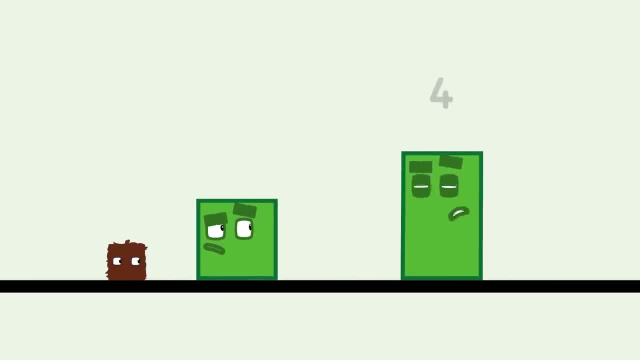 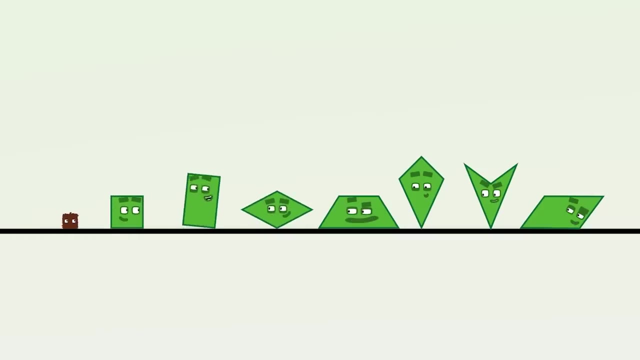 Like you, I have four sides and four corners, But your sides are all the same and mine are not. If I'm a surprise, wait until you meet the others. Hello, Four-sided shapes, introduce yourselves. Rectangle Rhombus. 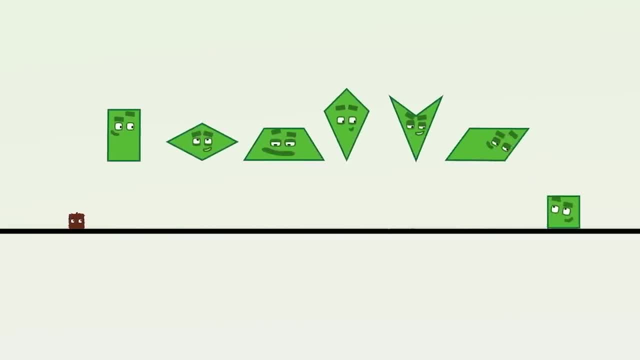 Trapezium, Kite, Dart, Parallelogram Square. Ooh, what wonderful names And what wonderful shapes: Rectangle, Rhombus, Trapezium, Kite, Dart, Parallelogram Square, Ooh. 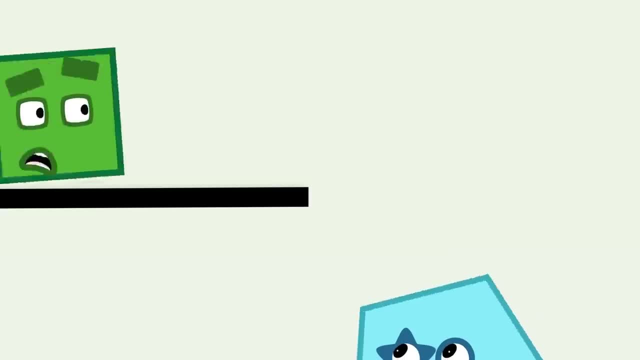 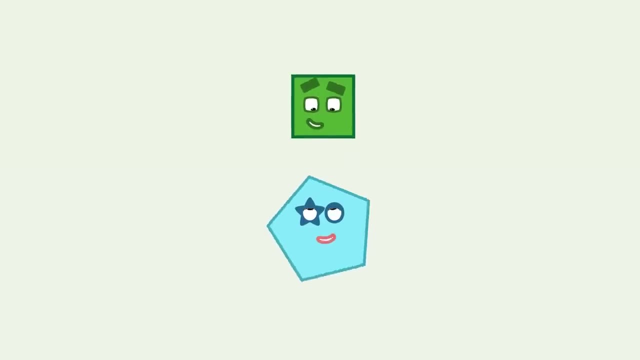 Squeary come back. Ooh, ooh, ooh, Oh. hello, who are you? I'm a pentagon with five sides, High five. Oh Ooh, Let's have a hexagon in the mix. 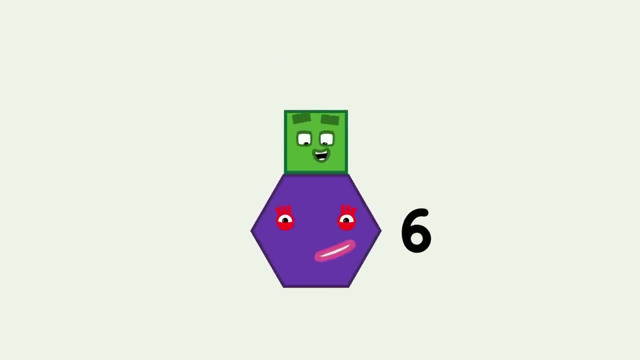 Count my sides and you'll find six. Huh, Ooh, And lucky me, I've got seven sides. I'm a heptagon. A heptagon, Ooh, Ooh, Ooh. One, two, three, four, five sides. pentagon. 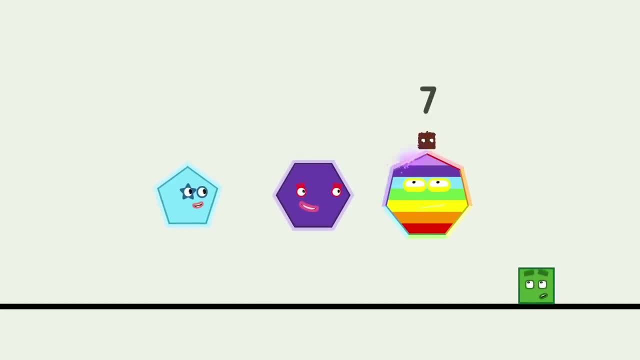 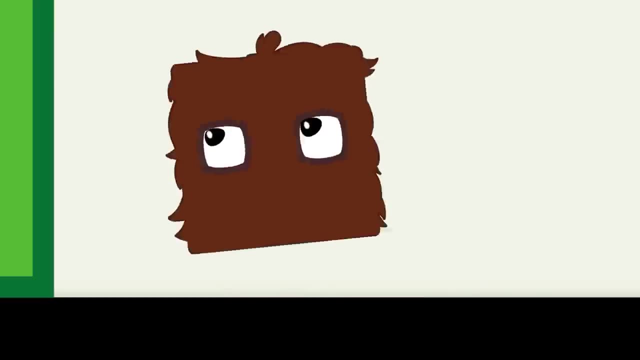 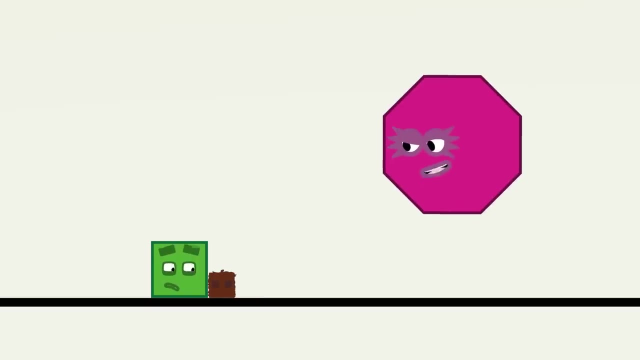 Six sides hexagon, Seven sides heptagon. Ooh, what wonderful names And what wonderful shapes. What's that Squeary? You're ready to go home? Hey, have no fear, Octagon is here. 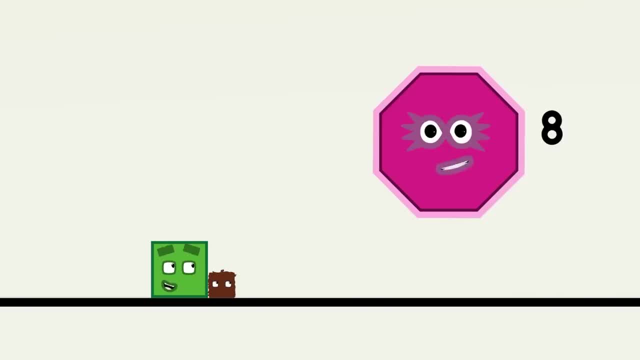 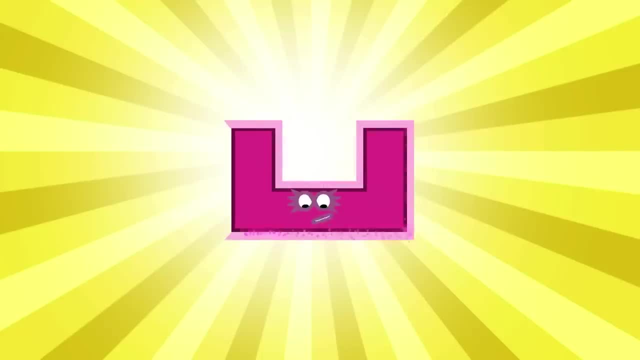 One, two, three, four, five, six, seven, eight, Eight sides. I will get you home, Octagon, make an eight-sided flying basket. One, two, three, four, five, six, seven, eight. 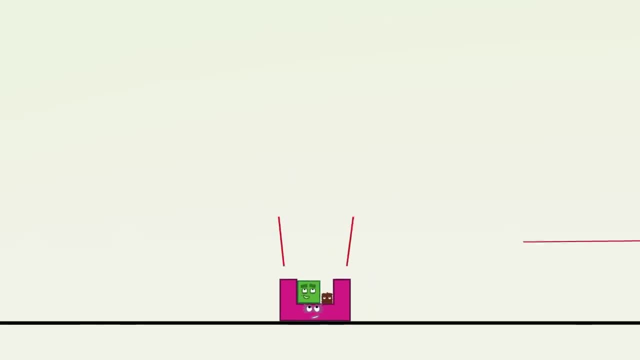 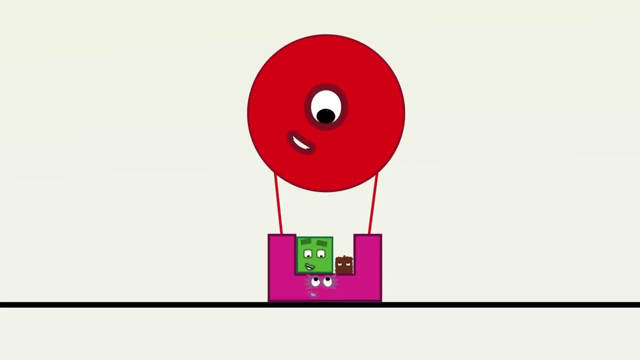 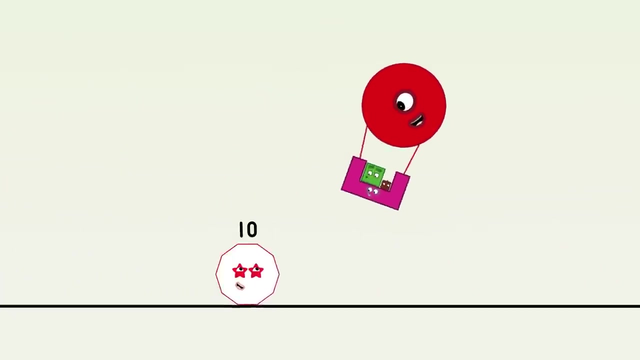 Basket. I'm a circle. I have just one curved edge. Hold tight folks. Here we go. Ooh Hey, Ooh, Wow, Ooh Ooh. Good-bye new friends. Ooh, Ooh. 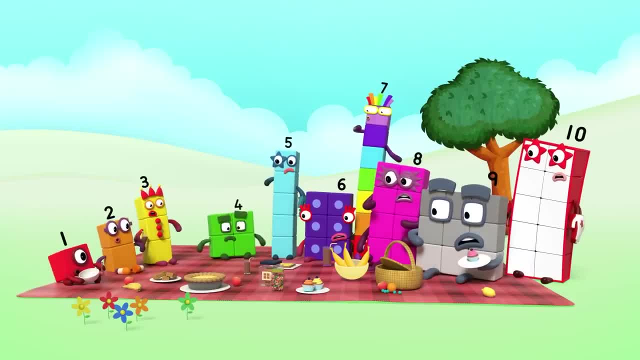 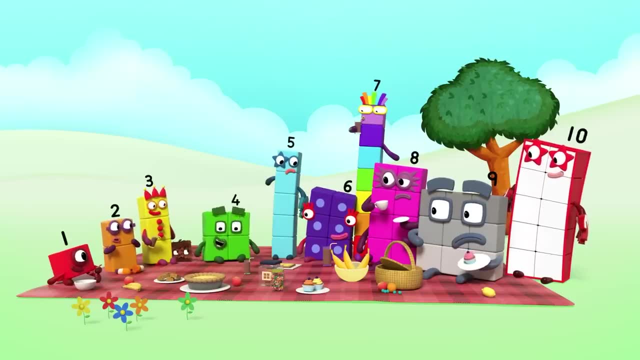 Ooh, Ooh, Ooh, Ooh, Ooh, I'm me again and you're you, Yep, yep. We went to Flatland and triangles were there and a rectangle and a pentagon and I was a real square. 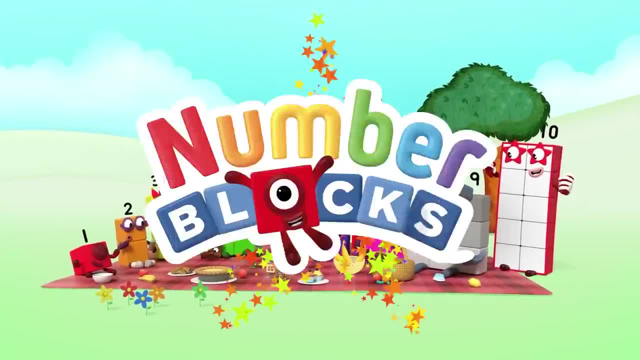 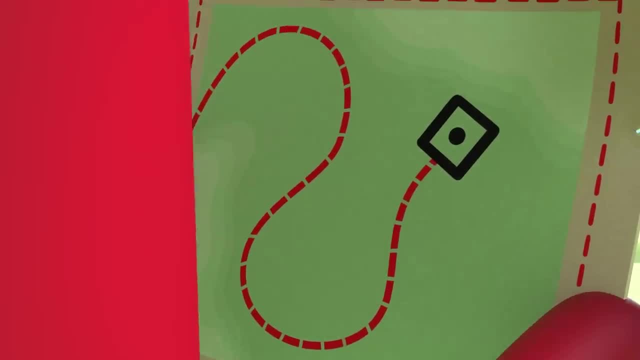 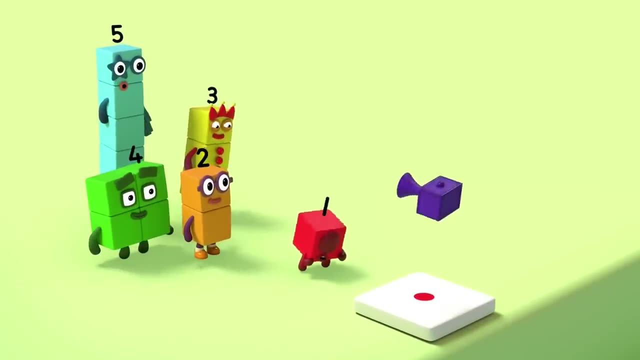 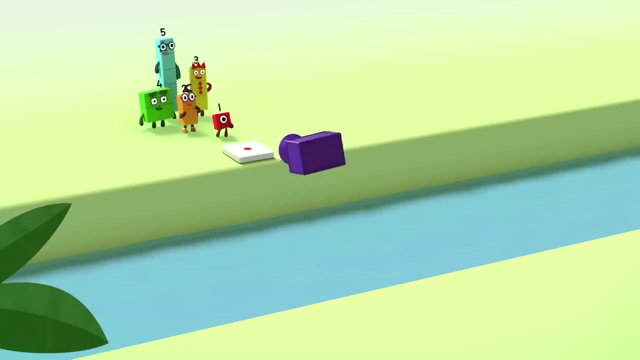 Yay, Woo-hoo, Yay, Yeah, Oh. Um, if the map is right, the Pattern Palace should be right here. Oh, Welcome to the Pattern Palace, where you can play all day, But first you must cross the Pattern Paths. 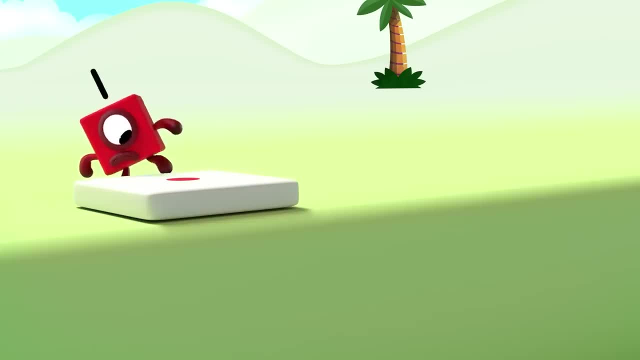 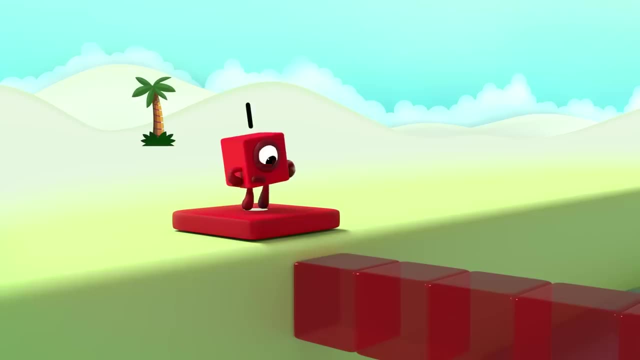 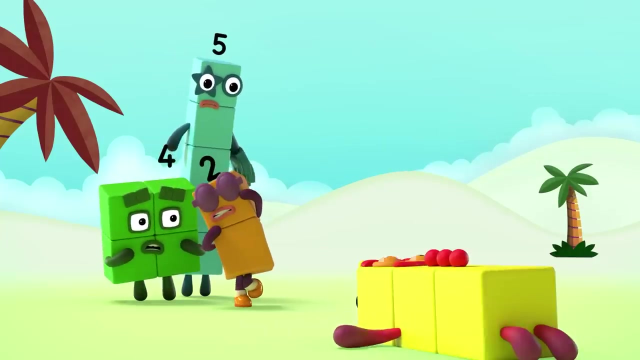 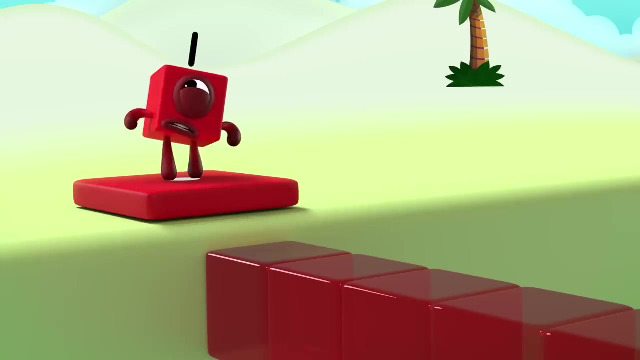 Be brave and skip this way. Ha Ooh, Follow the Pattern. Ooh, here I come. Whoa Ooh, Ooh, Ooh, Ooh, Ooh. What happened there? Uh, The blocks are red, like me, so maybe I should go first. 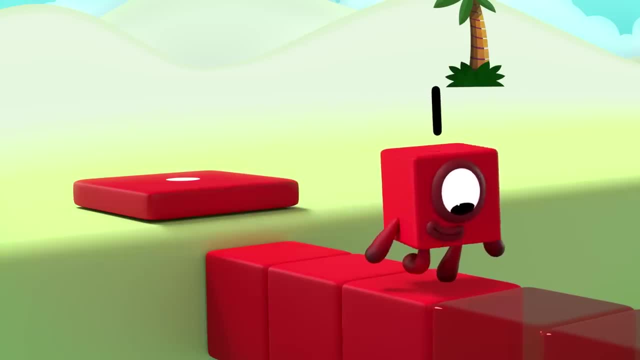 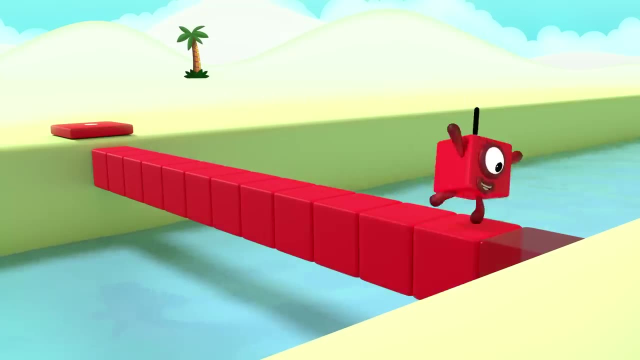 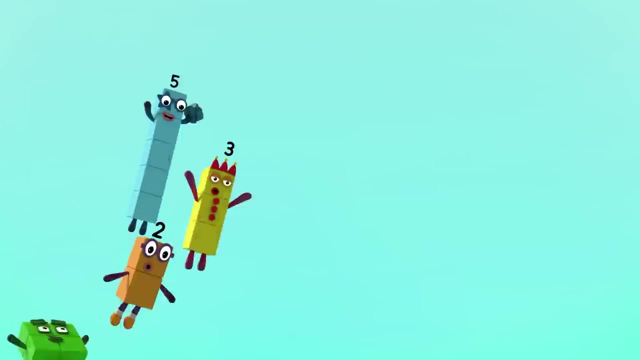 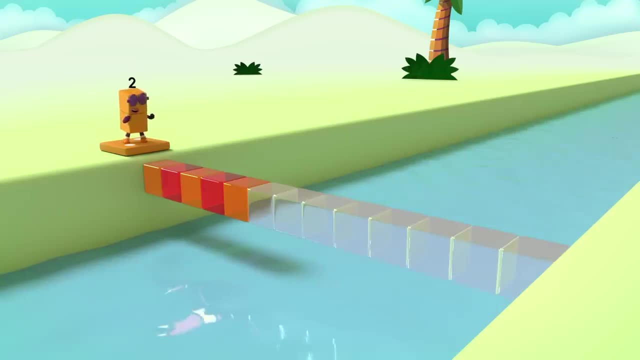 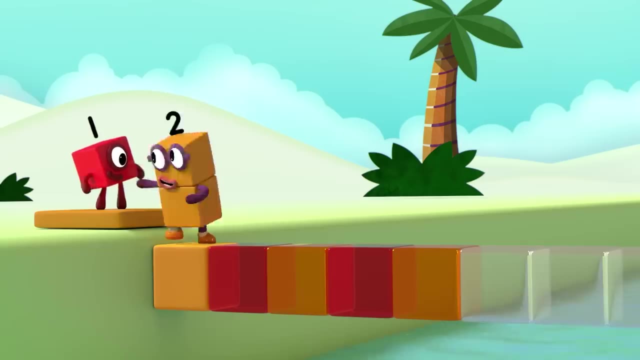 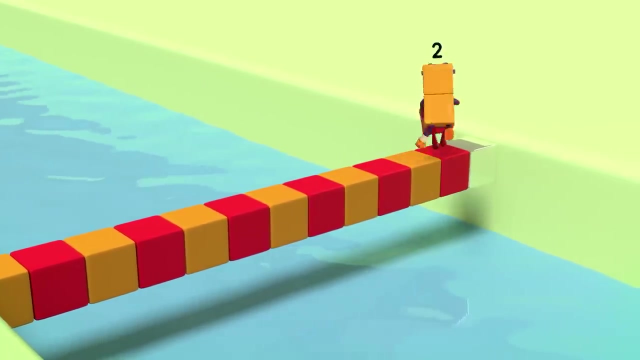 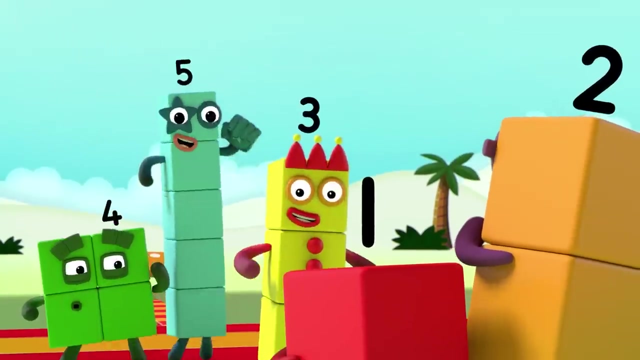 Ooh, My turn Orange, Uh-oh, The second one's red One. Red Orange, Red Orange. Ooh. Continue the pattern. Ooh Oh, Red Orange, Red Orange, Unlock Ooh. 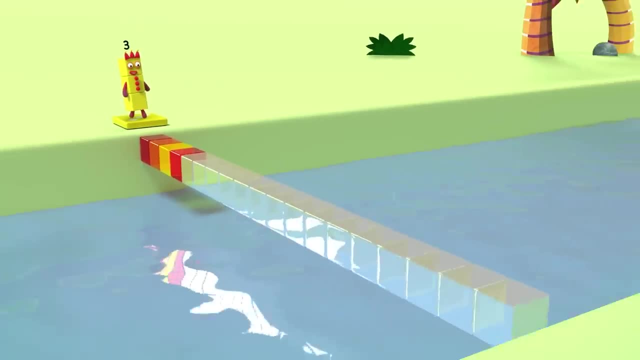 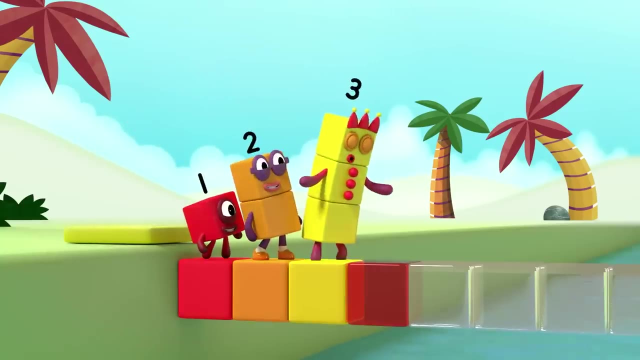 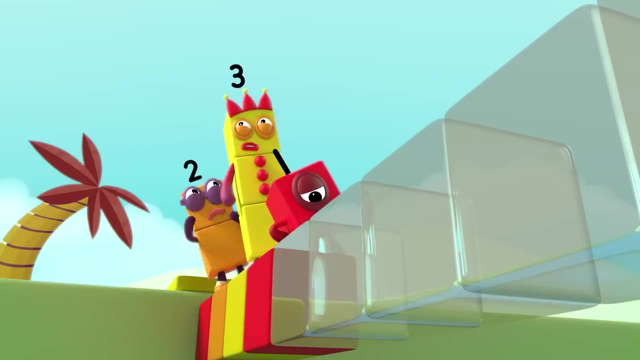 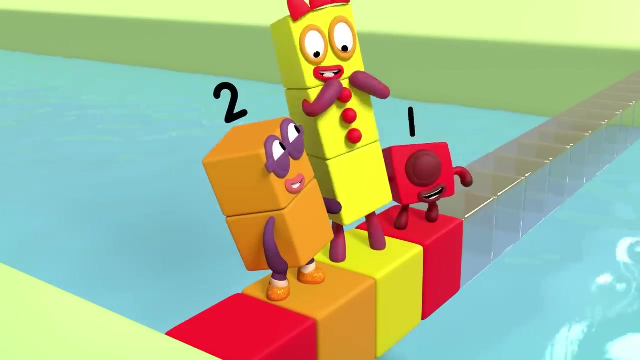 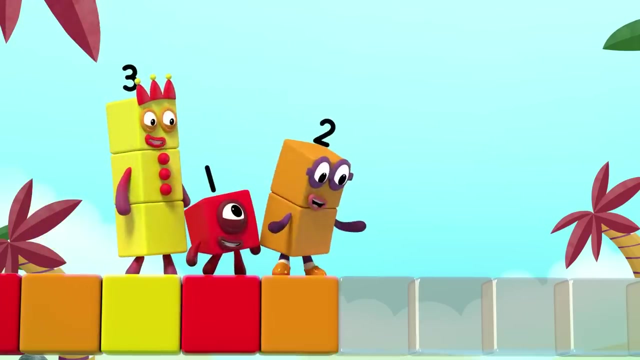 At last Me, me, me, Yellow. No, it's not Red Orange, Yellow, Red. Stop, Who's next? Hmm, Ah, Um, It goes. red orange, yellow, Red Orange, Yellow. 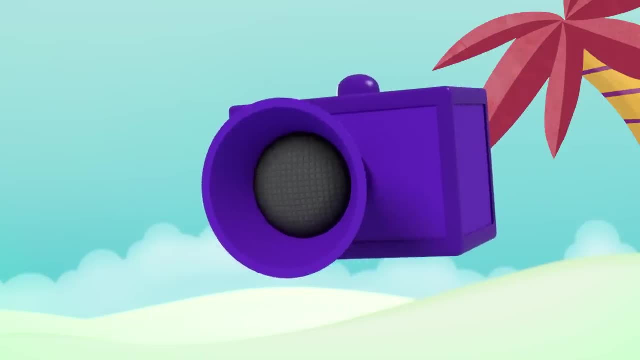 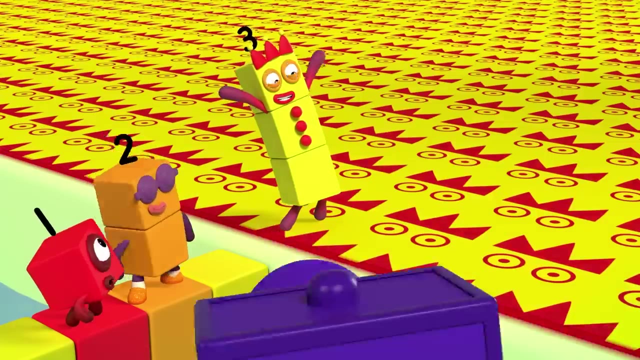 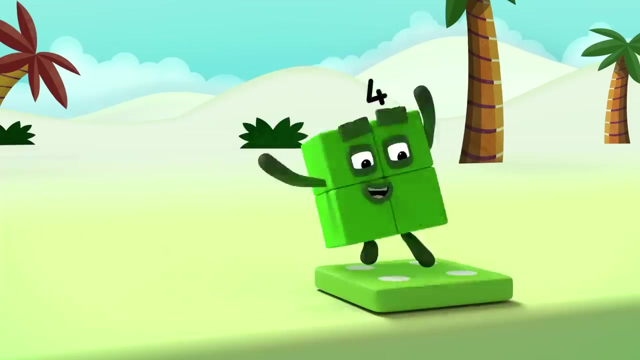 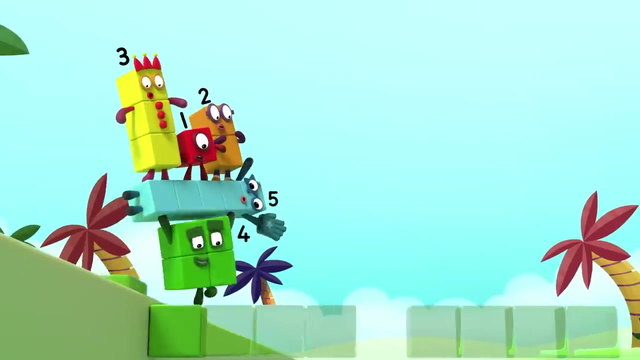 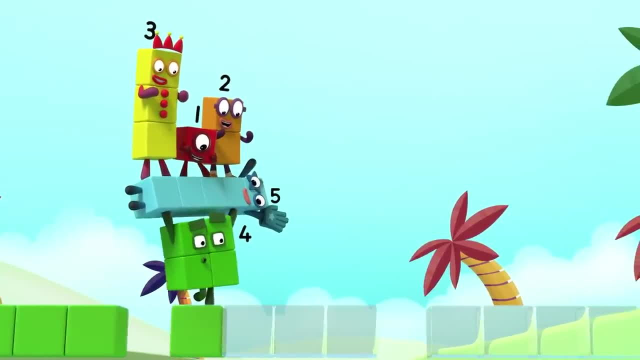 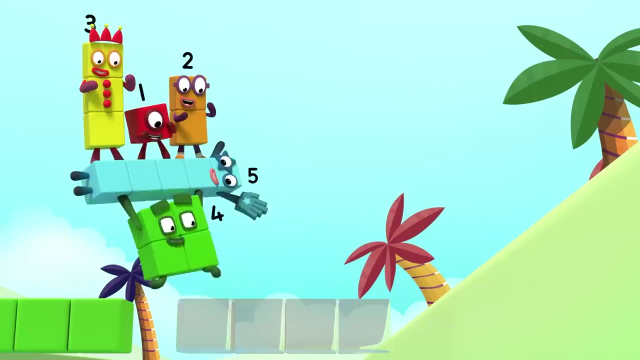 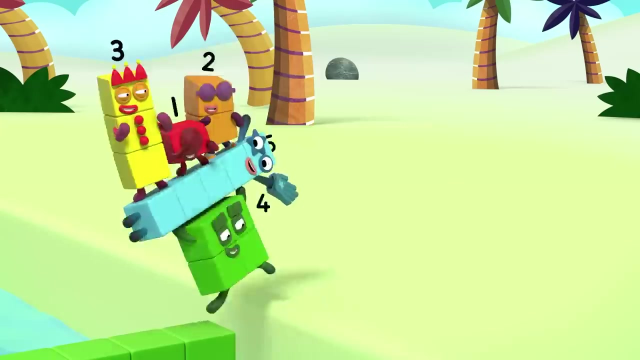 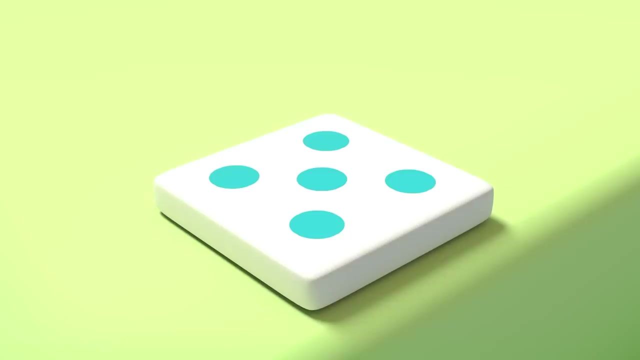 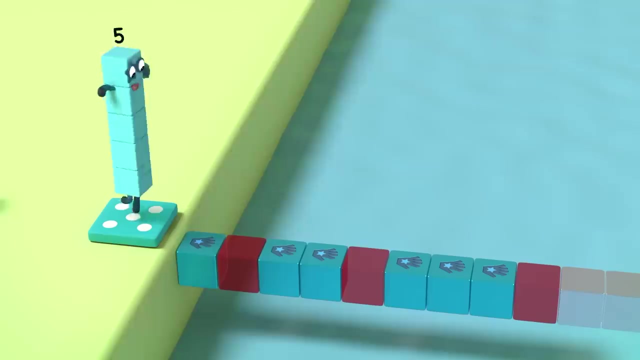 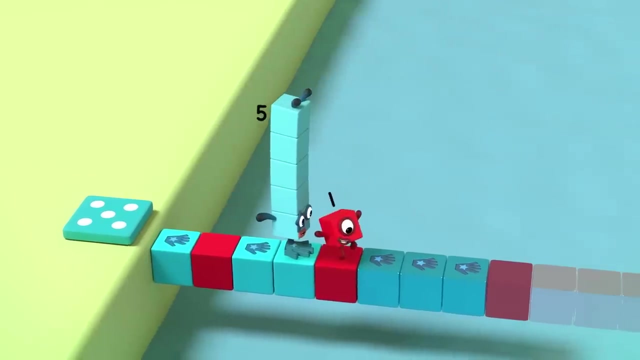 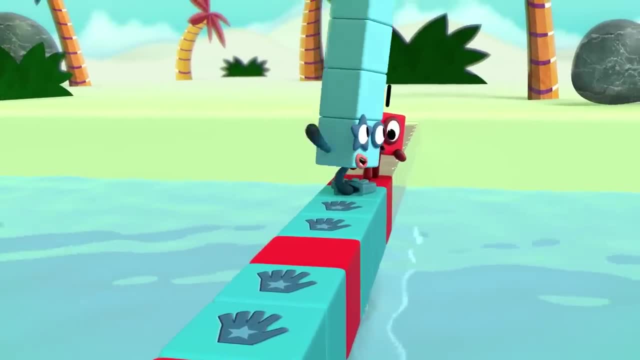 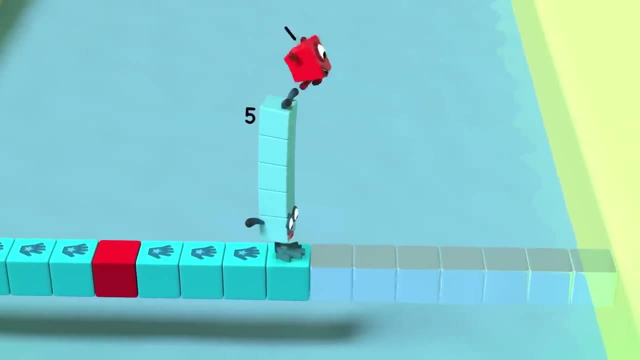 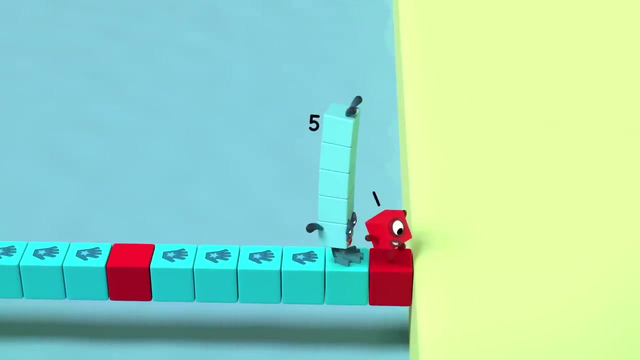 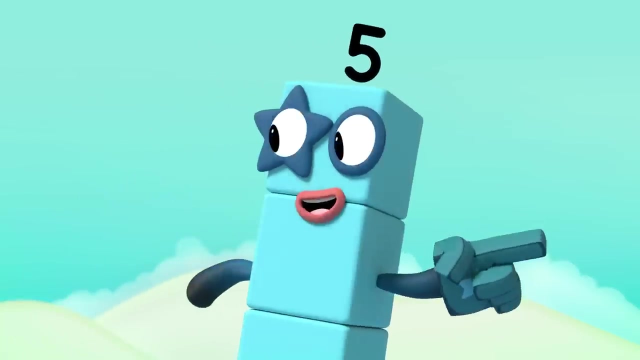 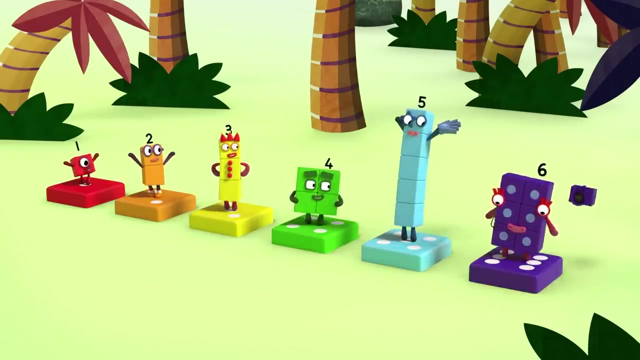 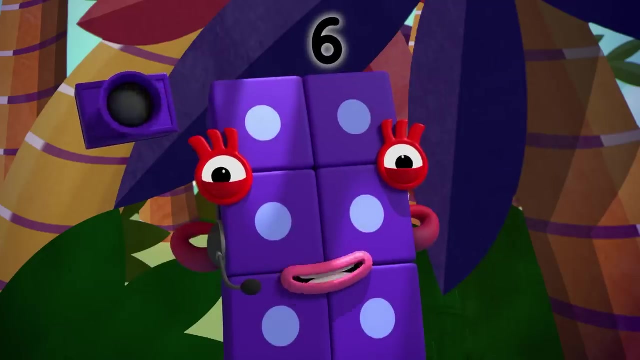 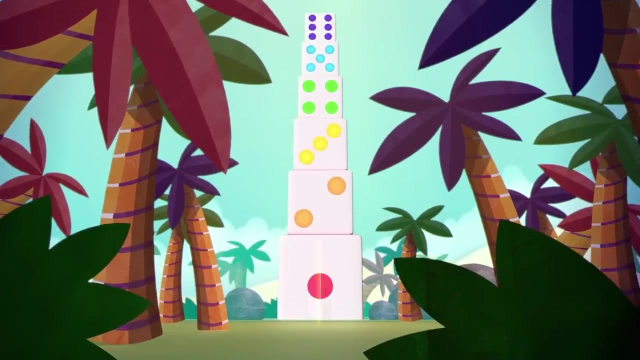 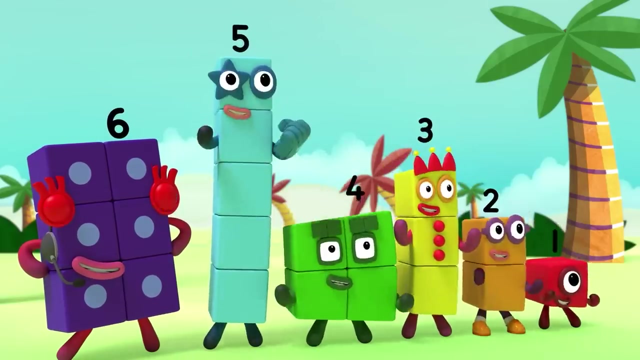 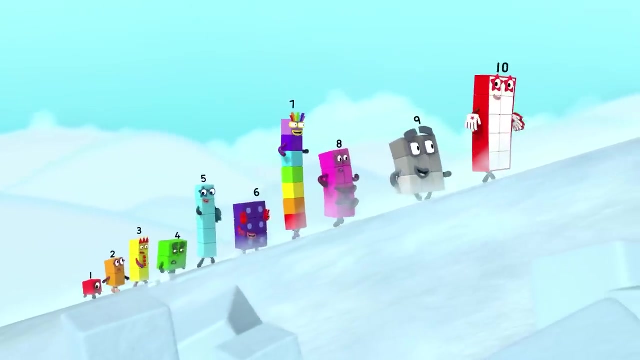 One hand, two hands, three hands got it. next comes four hands: hand One more time. each time We're at the center. Three, four, five, six. You've got across my pattern paths. well done everyone. now step into my pattern palace. Phew, it's cold up here. keep going, everybody. We're near the top of lucky mountain. 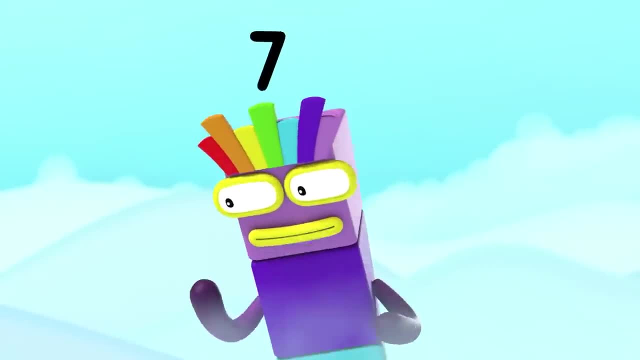 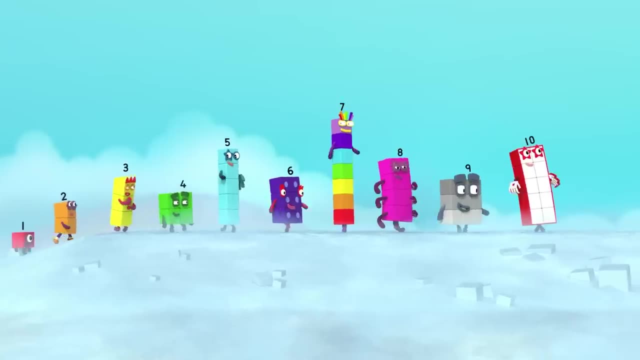 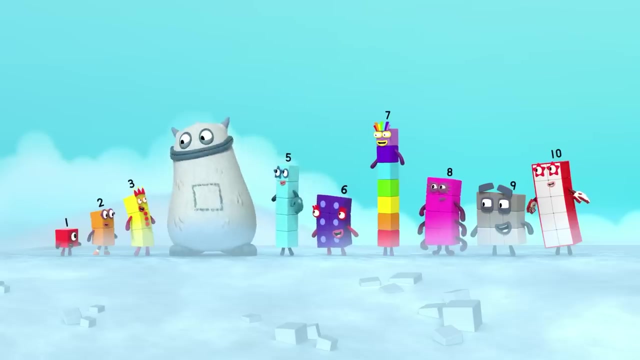 If we're really lucky, we might spot the legendary big tum, A big hairy monster with a big hairy tummy who loves puzzles. Don't be silly. seven Yum, Yum, Yum, Yum. Who's in my tum? Who's in wait? is one of us missing? 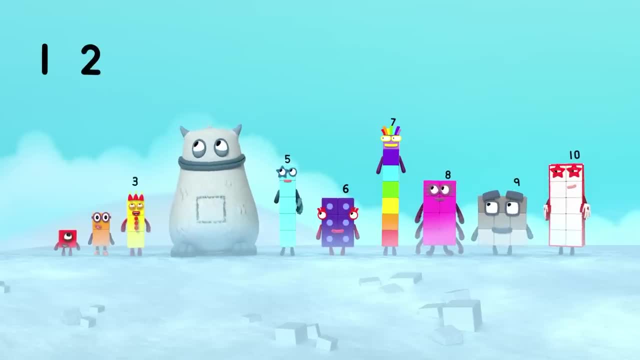 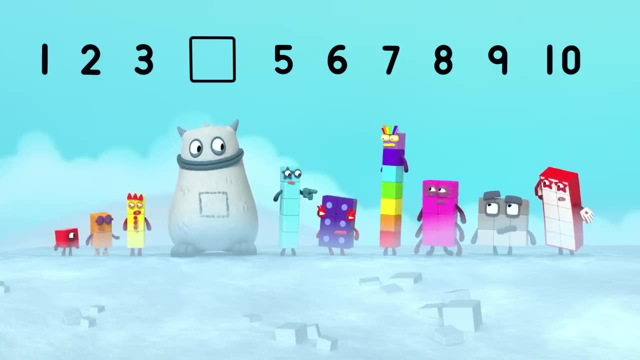 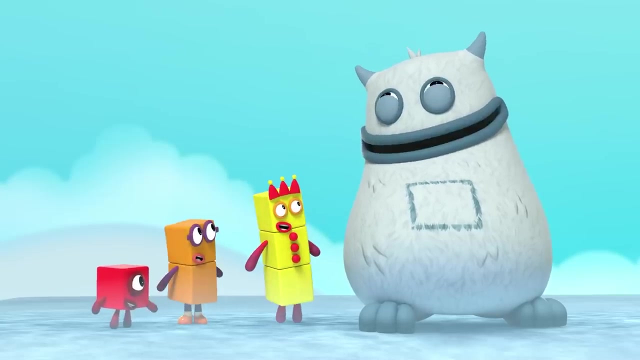 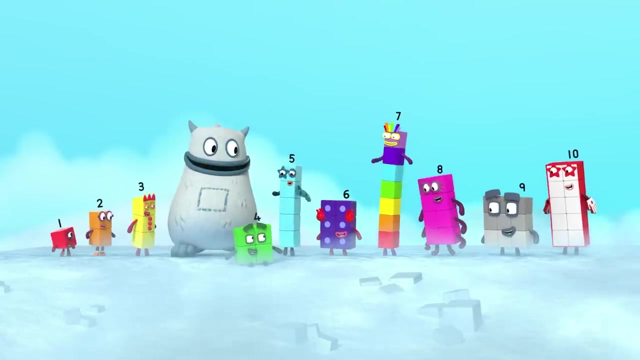 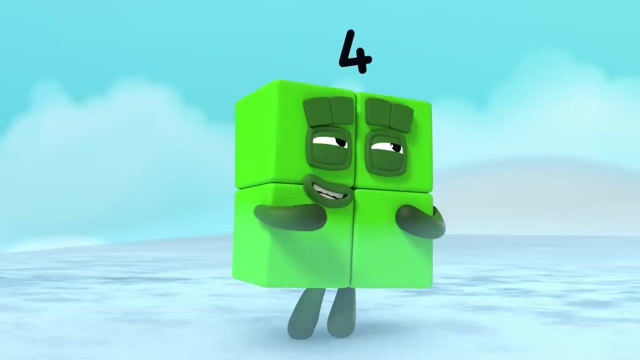 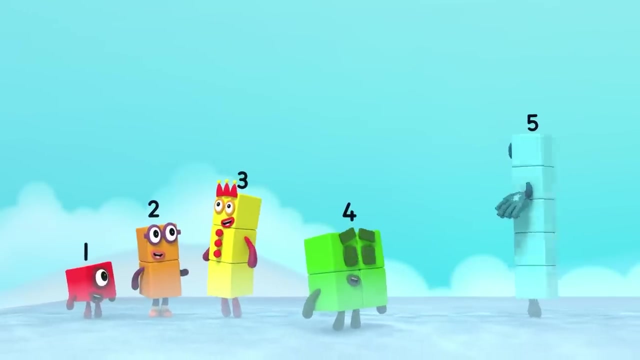 Everyone call out your number one, two, three, five, six, seven, eight, nine, ten. Where's four, fours missing, fours in your tum? Yum, well done. Are you feeling okay? four who I find? thank you, it was warm and snugly and bitum's dumb Game on coming ready or not. 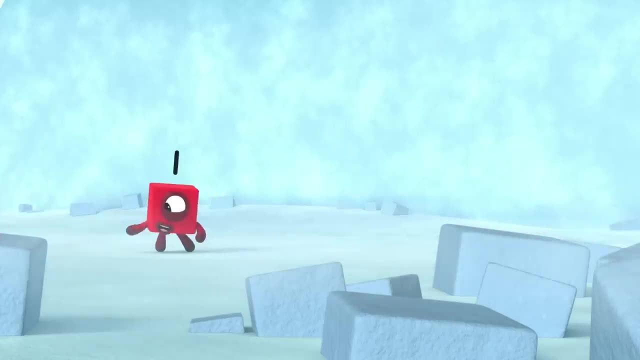 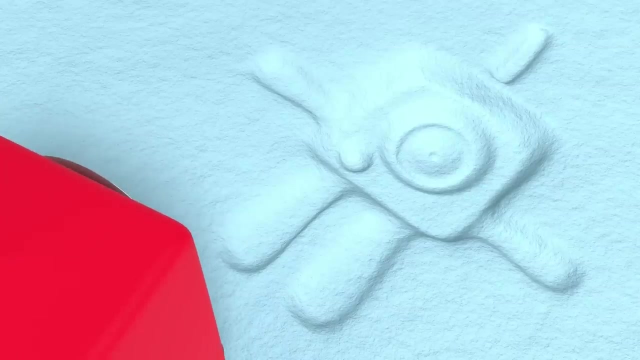 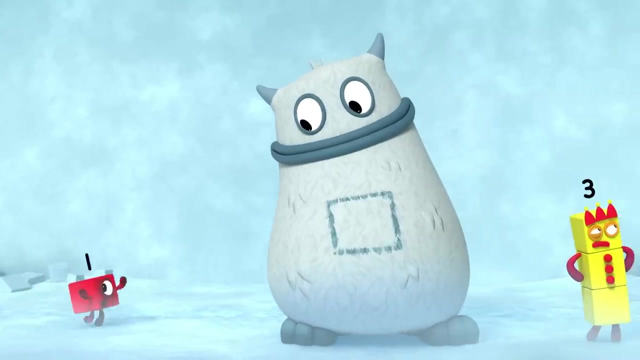 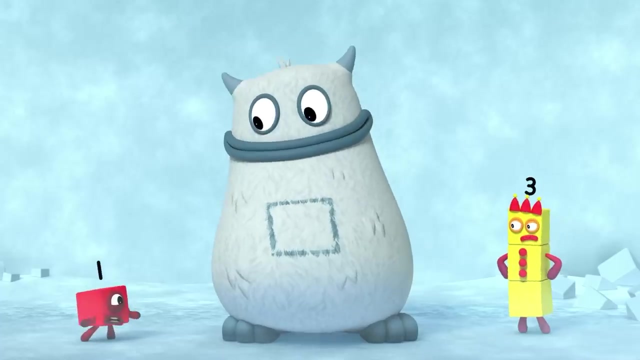 Oh, Nice, smooth snow. Yum Yum yum. Who's in my tum? Nine? Oh no, Where are you? It was me. I was nine And Big Tum gobbled up some of my blocks. How many. 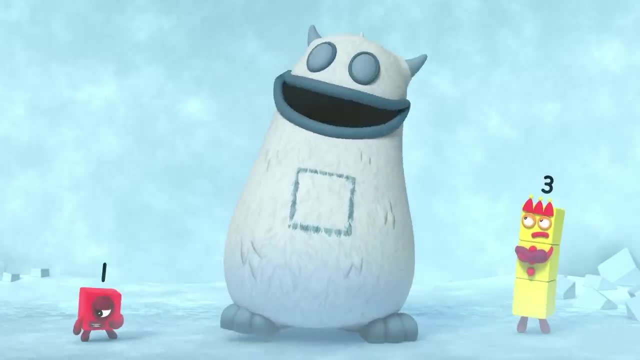 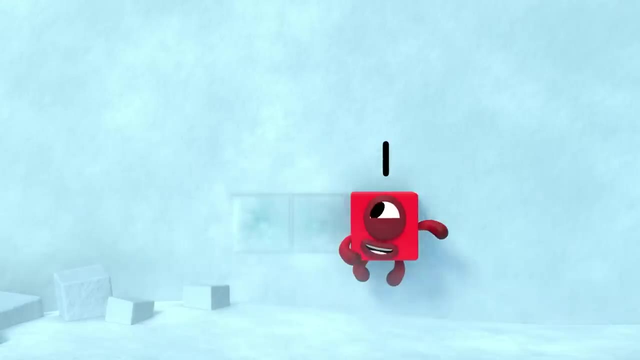 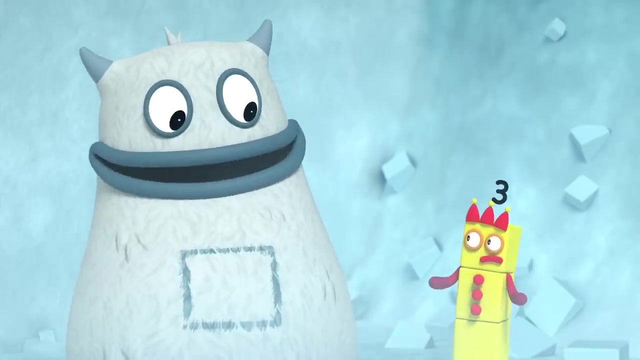 I don't know, I had my eyes shut. Oh, I know, Here goes One, two, three, four, five, six, seven, eight, nine. So nine was here. Then some of his blocks were taken away. 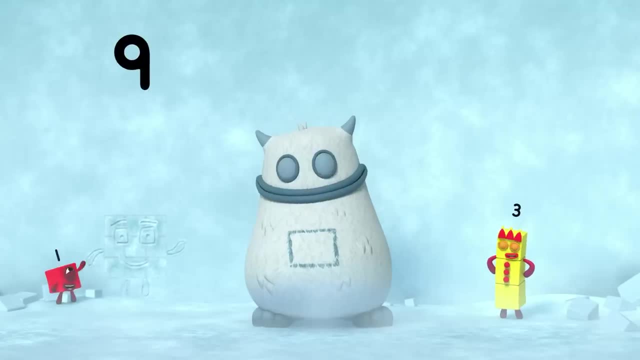 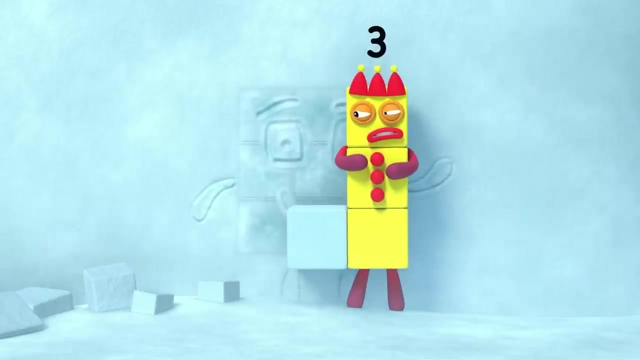 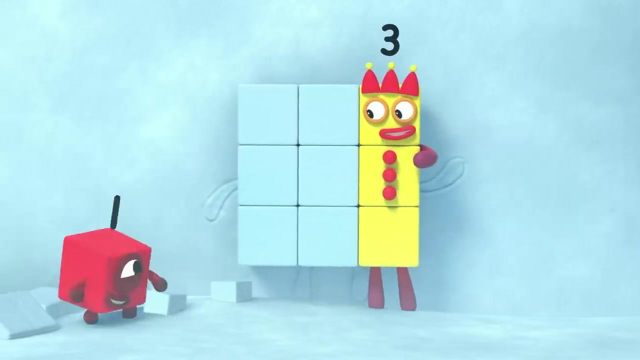 And that left you three, Which means nine minus Yum Equals three. So what's missing? Hmm, Come over here. Three, Hey, That's one, two, three, four, five, six There. So that's what's missing. 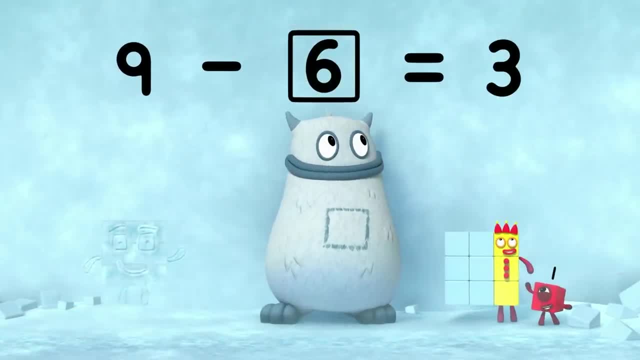 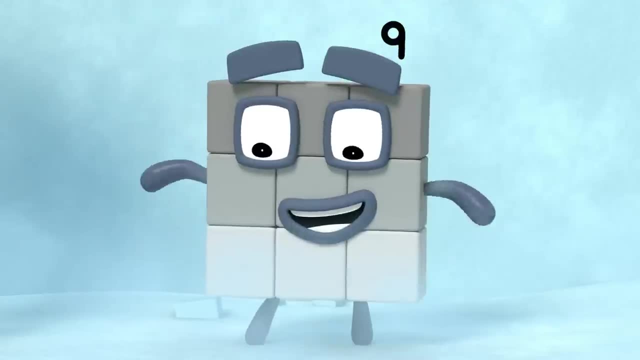 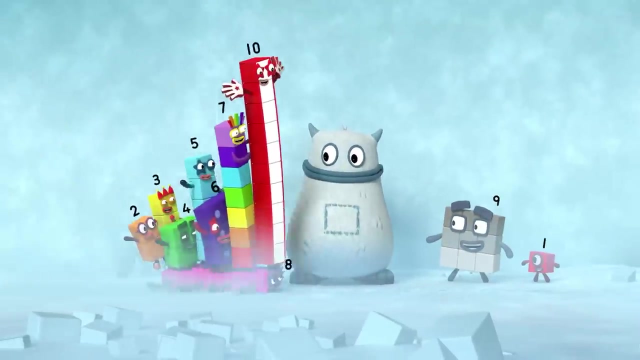 Nine minus six equals three, And six is in your tum. Yum yum. Well done, It's good to be back. Where are the others Up the block sledge? Yum yum, Yum yum. Everybody stay close. 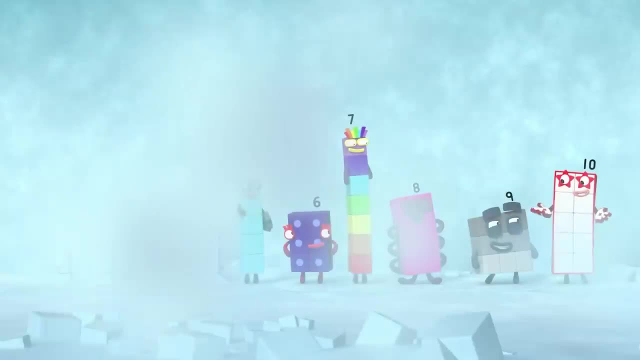 No need to panic. What's wrong, friends? Why don't you? Oh, they're made of snow. Snow, Yum yum. Who's in my tum? That's easy. The real one, two, three and four. 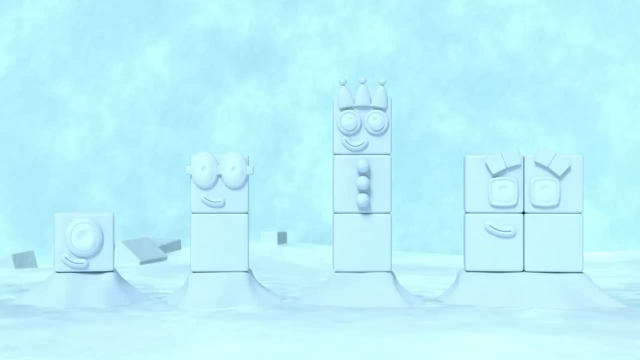 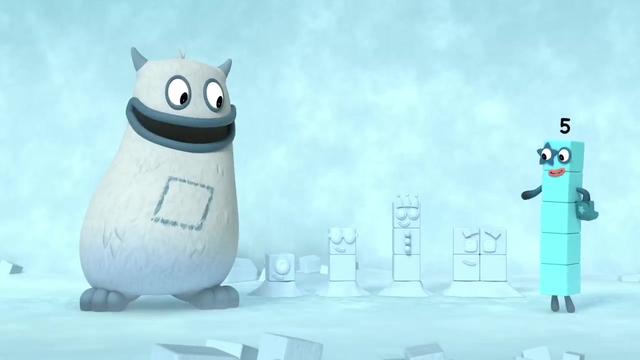 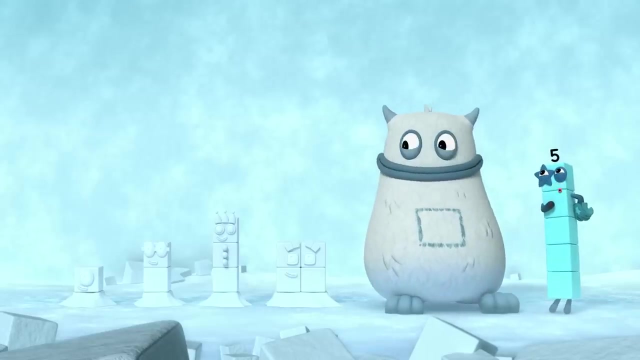 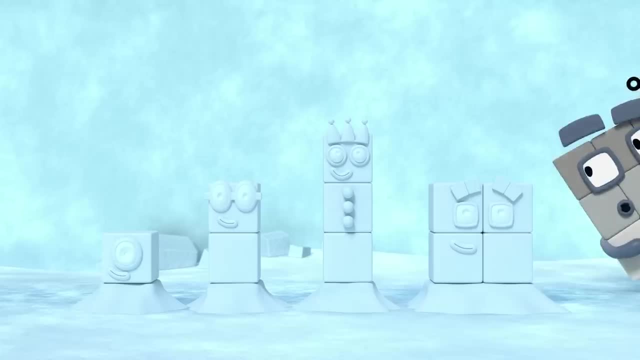 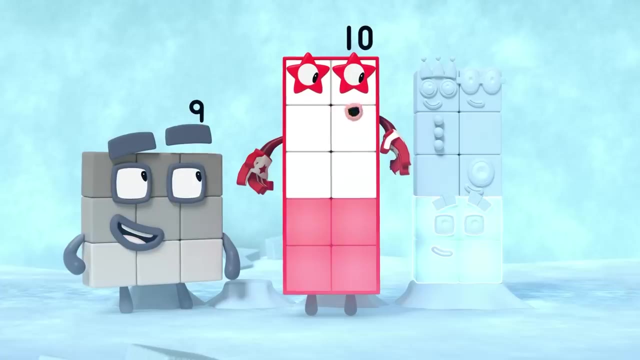 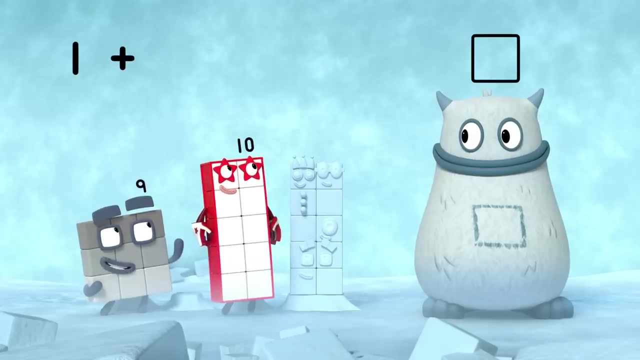 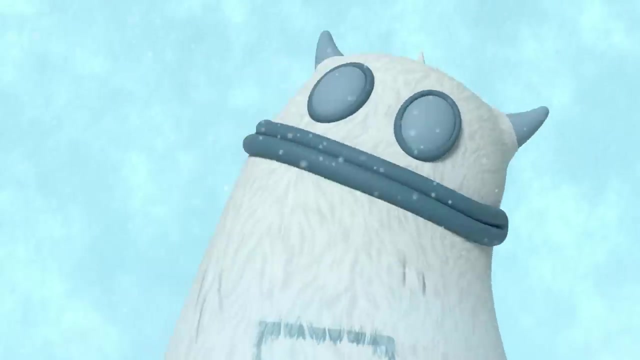 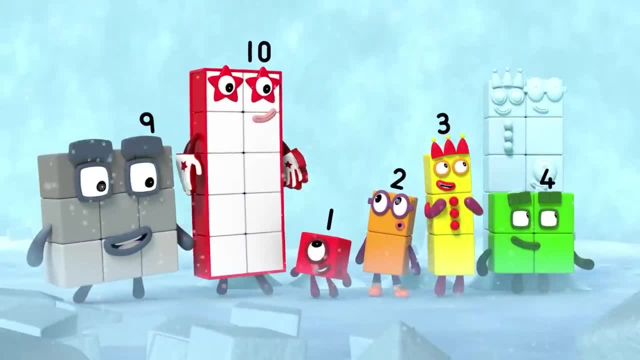 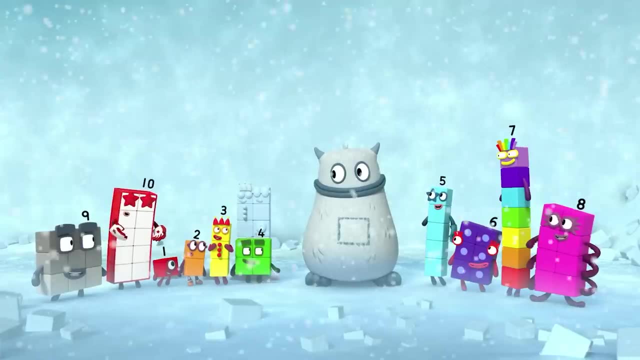 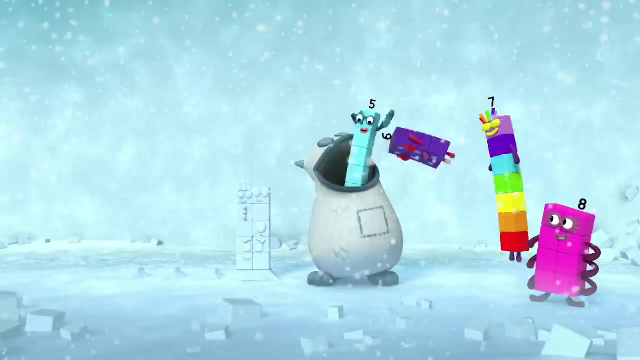 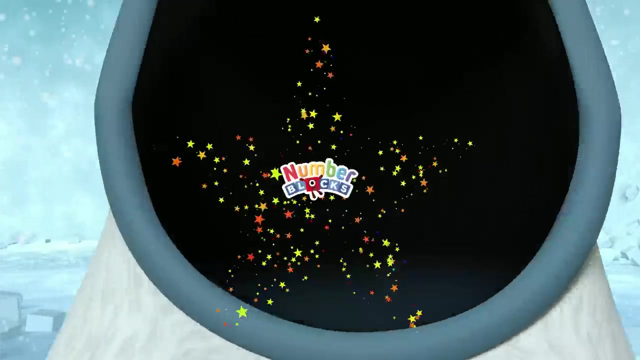 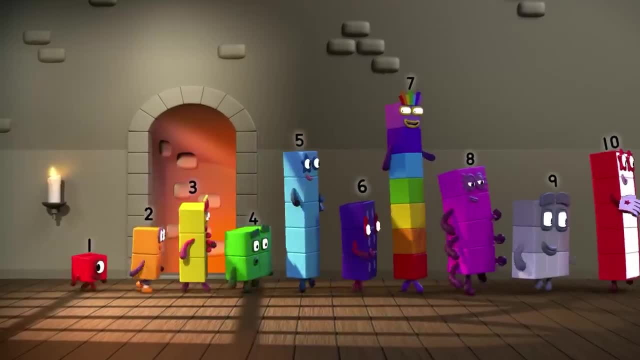 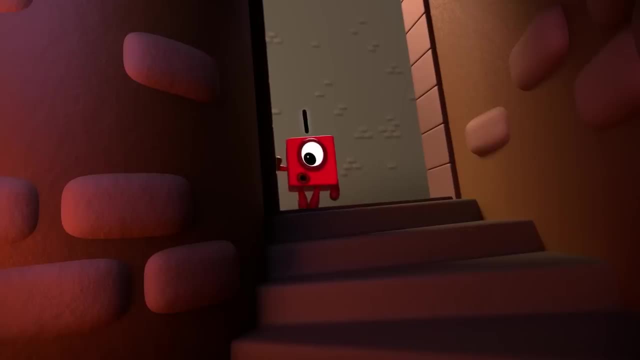 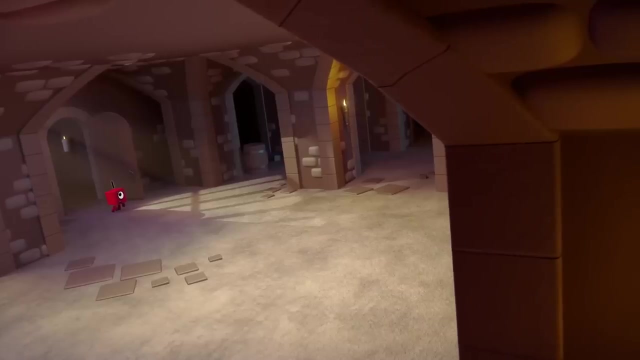 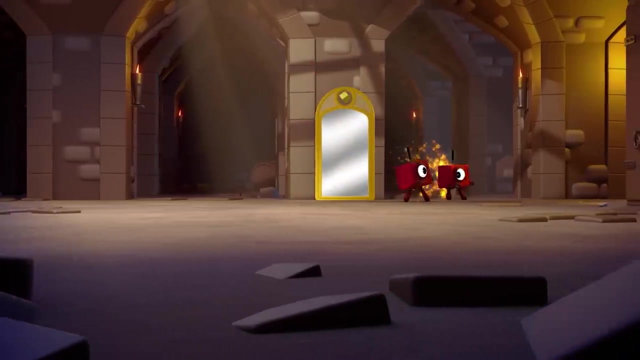 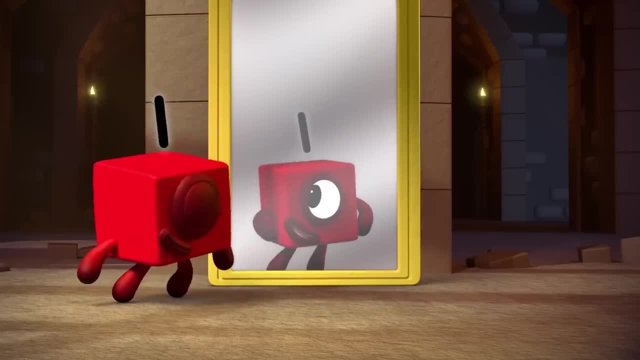 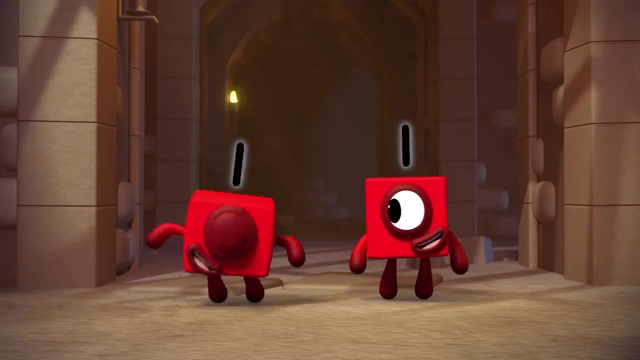 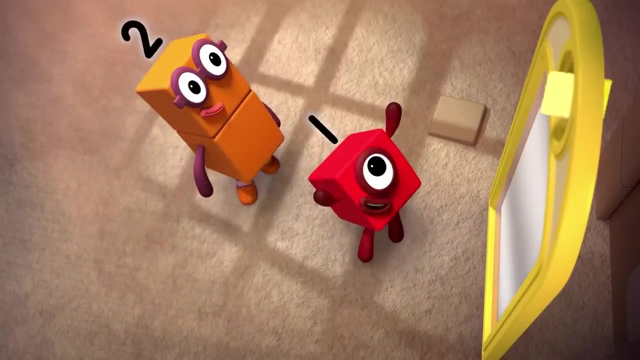 Snow, Snow. Oh, it's a magic mirror. Oops, I've made two. lots of me. Making friends is fun. Oh, let's make three. next, Oh, mirror, mirror, hear my plea. I wish you could make three of me. 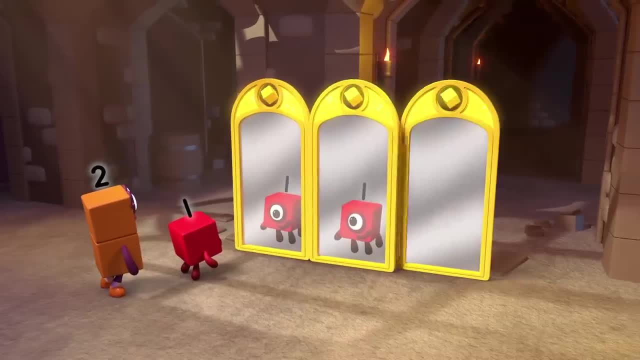 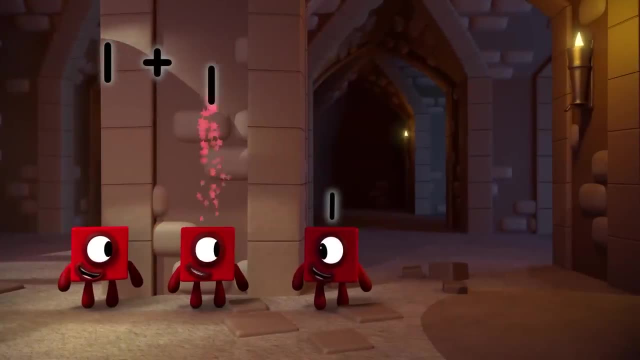 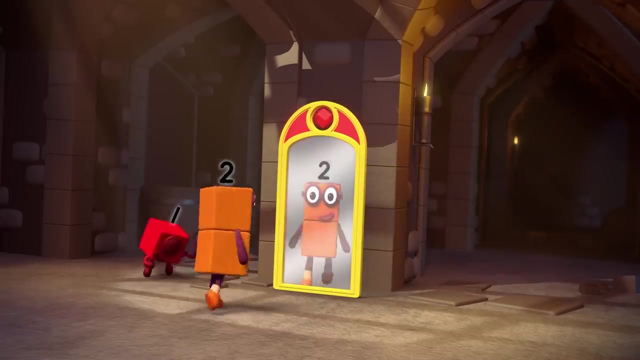 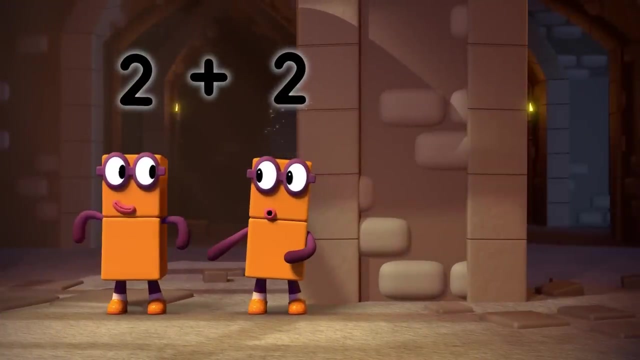 Your wish is my command. Wow, Three lots of one. One plus one plus one equals three. My turn, my turn. Two lots, please. Two lots of two. Two plus two equals four. I'm four, I'm two lots of two. 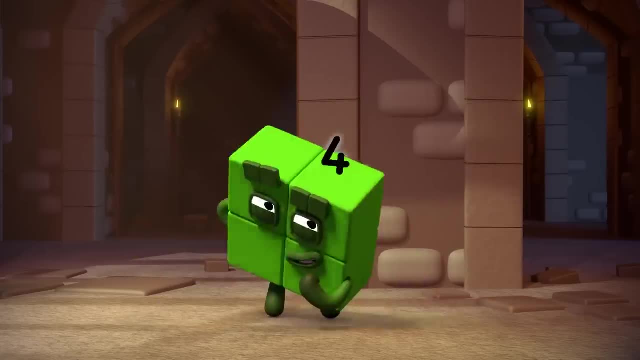 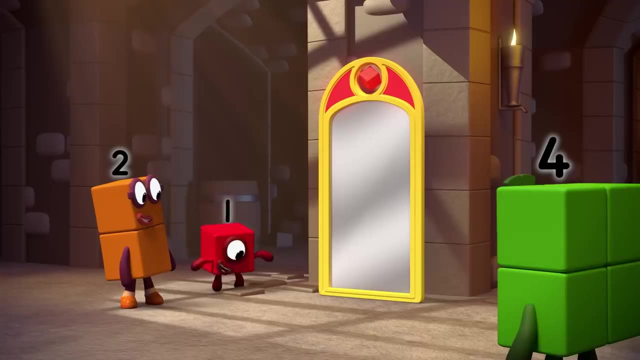 The terrible twos. Ahem, Aha, Oh, the magic mirror is even more magical than we thought. Oh, the others will want to see this. Keep an eye on it while I'm away and don't mess around with it. 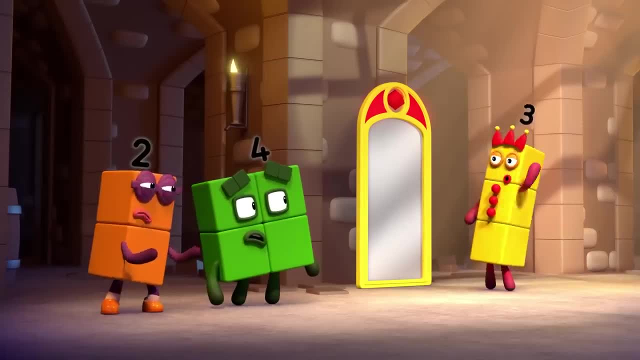 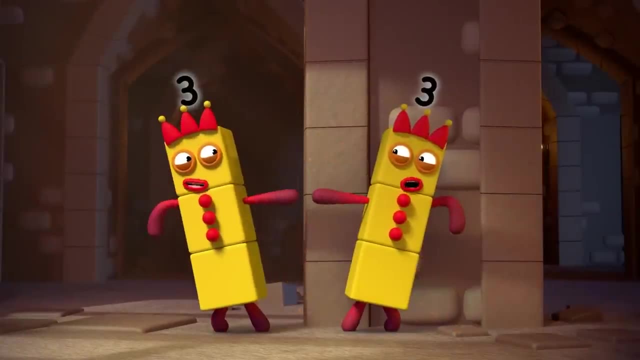 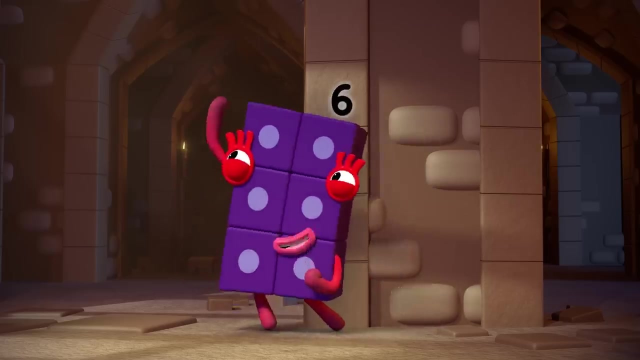 Right, my turn. One said not to. Oh, go on, it's only fair. Two lots, please. Two lots of three is six. Number six is on the floor. Don't be shy, Let's have some more Good idea. 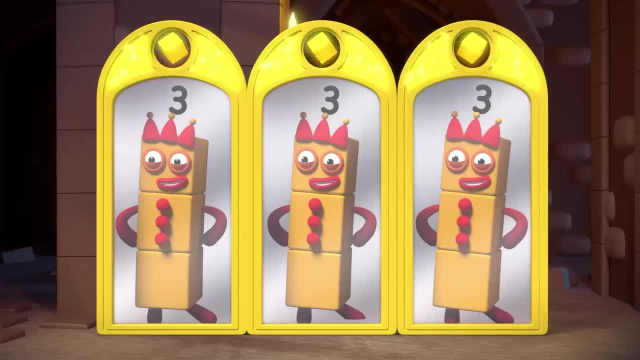 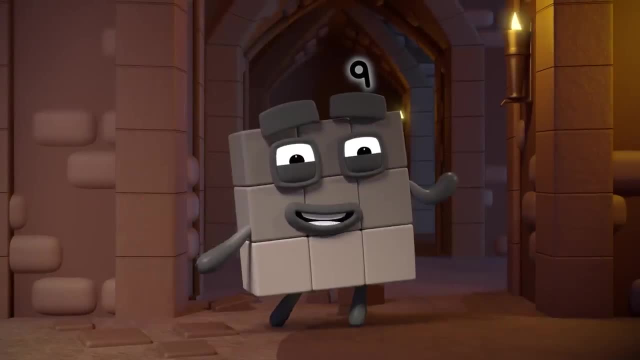 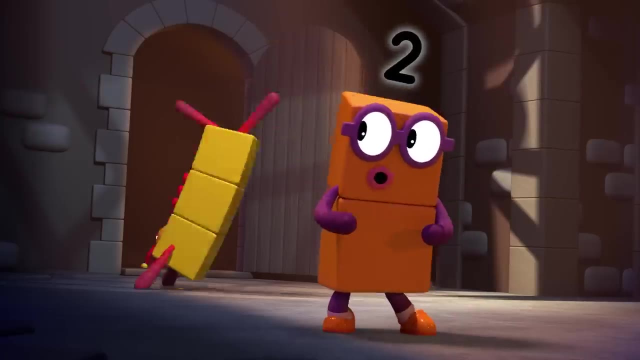 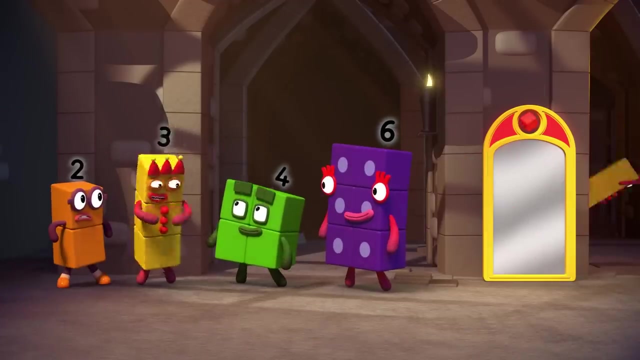 Three lots, please. Three lots of three is nine and three, threes, see, Yay, Oh yeah. Oh, we should probably stop now, But look, there are so many of us here already. Won't Bumbi be surprised if she comes back and everyone's here. 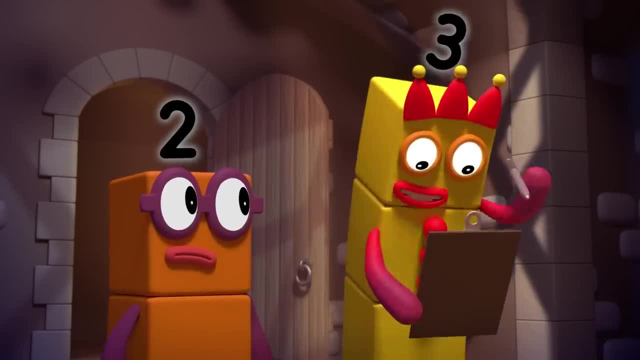 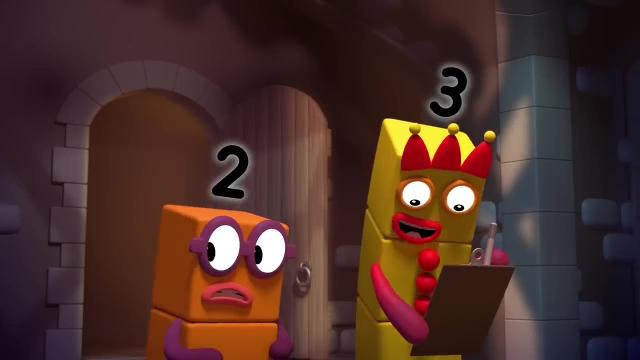 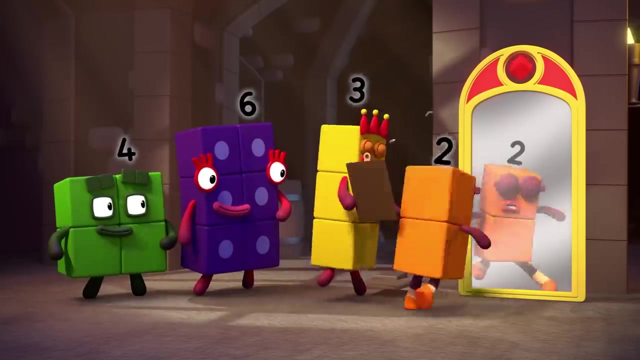 Mm-hmm. All right, then We've got two, three, four, then six. Oh no, We're missing five. How many lots of? who is five? Hmm, Let's try you. Oh, Three lots, please. 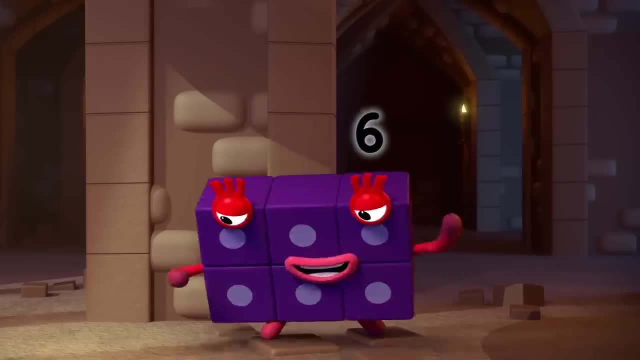 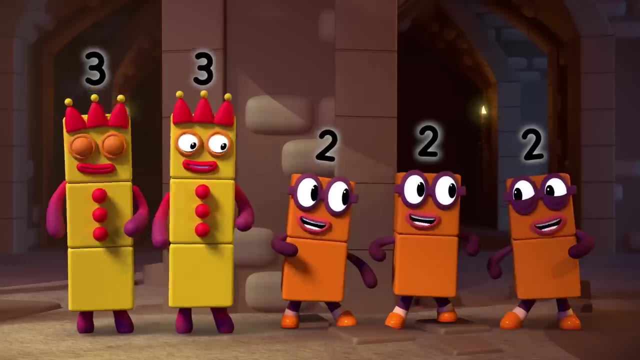 Three lots of two is six. Number six is on the floor. Wait, have I said that before? Two lots of three. Three lots of two. Yay, I was hoping for a five. Maybe I can help. No Two lots, please. 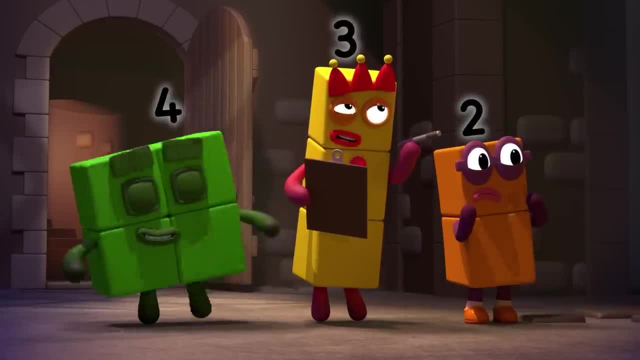 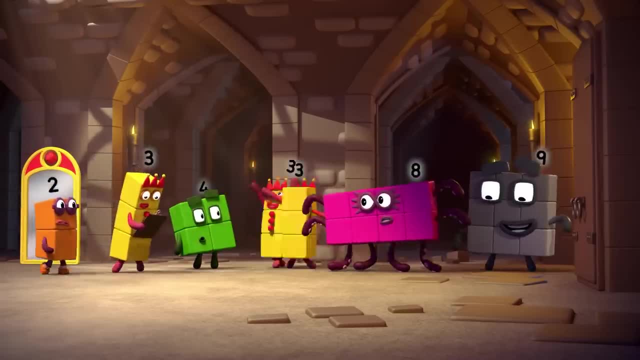 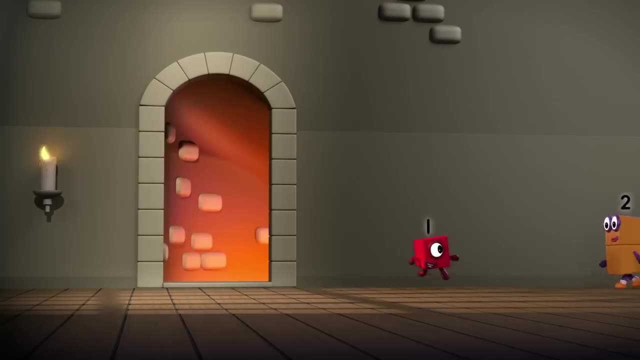 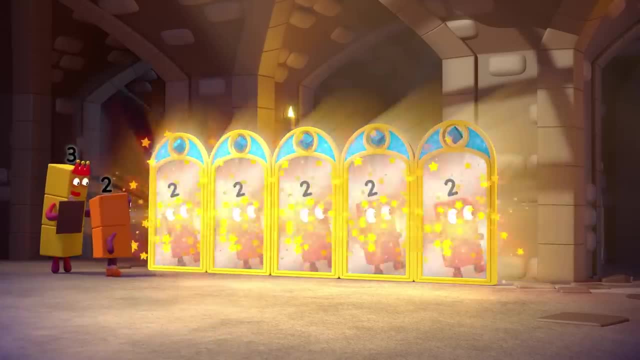 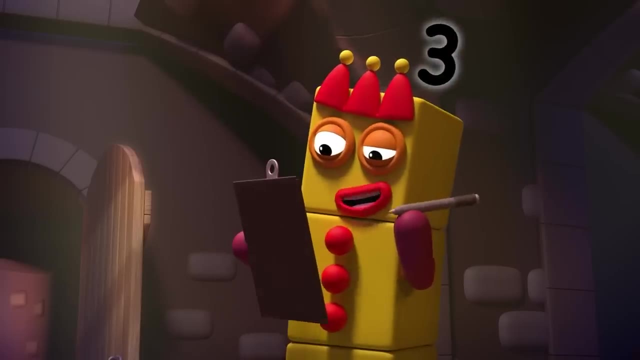 Oh no, Whoa. Five lots of two Is ten. That's ten sorted. All we need now is five and seven. Next, Get ready for our really big surprise: One's coming hide. Why can't we make five and seven? 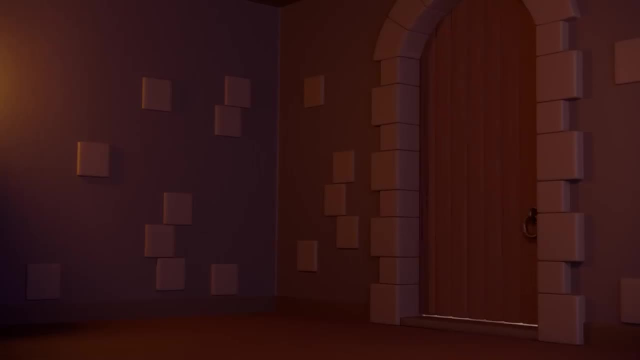 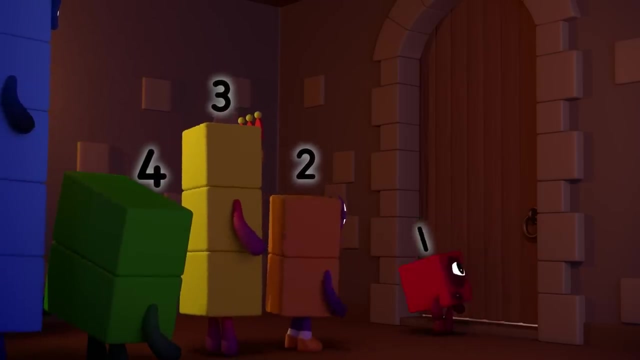 Oh, Who wants to try next? Let's go. No, Come on. Oh no, M-m-m. No. Who wants a five, Ten? Let's try six. Listen, Let's try it again, Oh no. 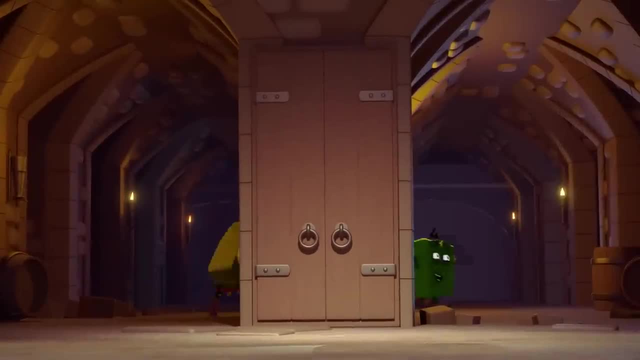 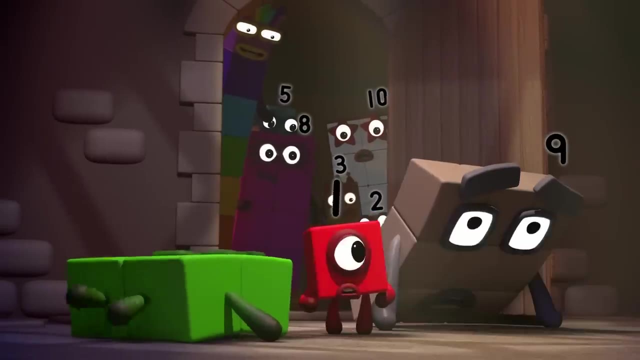 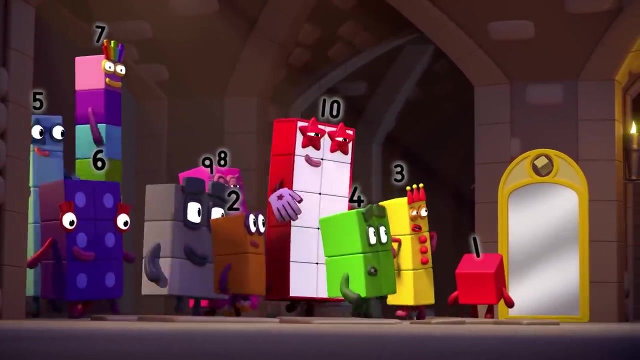 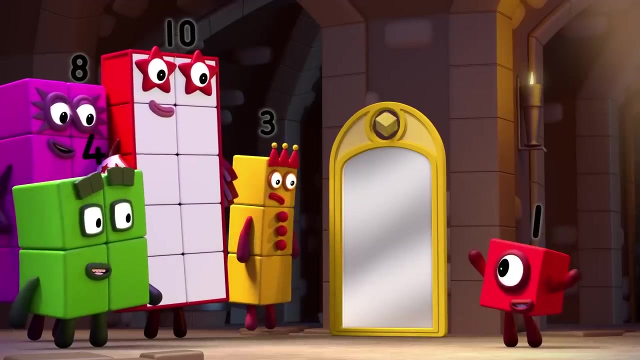 There, Surprise, A magic mirror, Some big surprise. Ah. But what if I said I could make lots of number blocks appear all at once? Now that would be a Ah. But what if I said I could make lots of number blocks appear all at once? 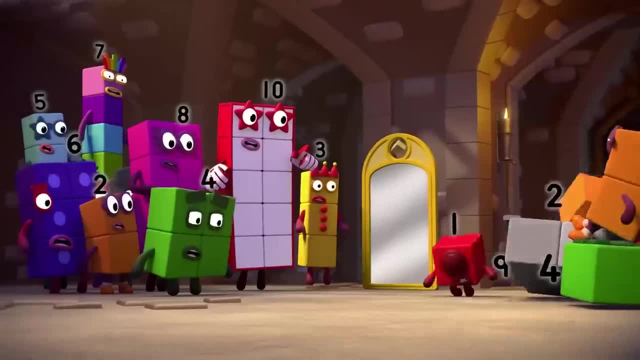 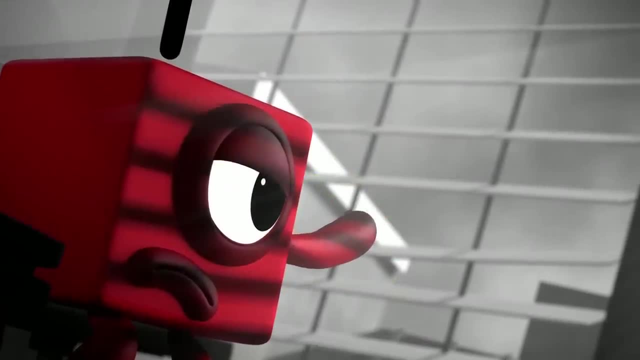 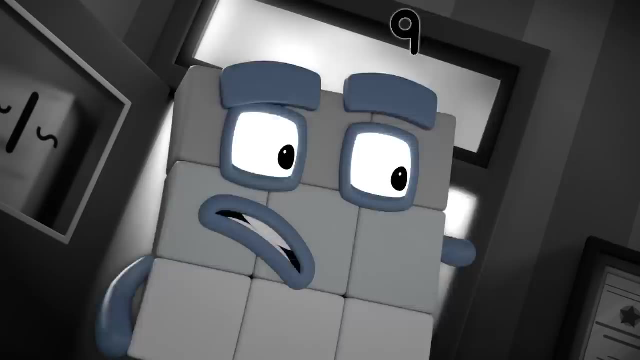 Now that would be a Surprise. That was a great day in the big city. I was wondering where my next case would come from when You've got to help me. One: It's gone, Everything's gone. Slow down. Nine: Tell me what happened. 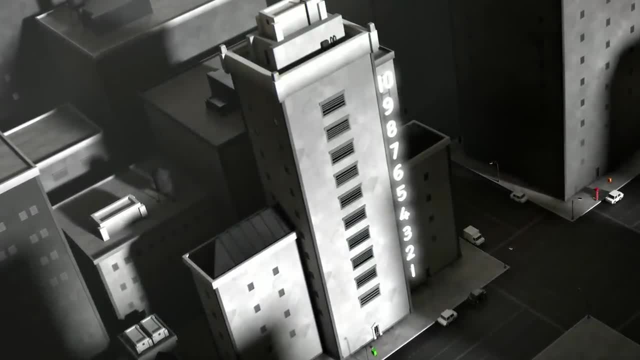 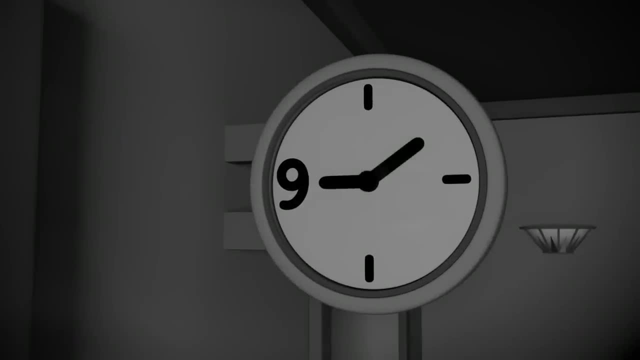 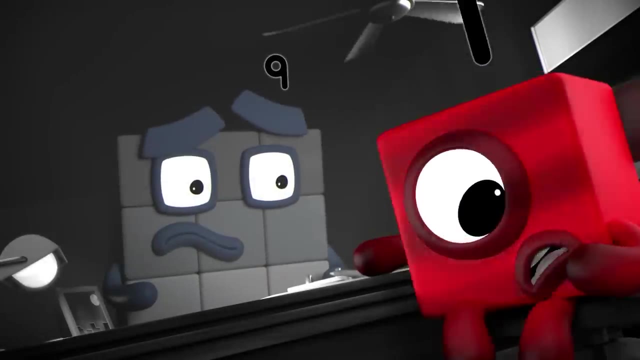 I live in Apartment Nine on the ninth floor of Numerical Towers. I left home this morning at nine o'clock to buy a newspaper. When I came back nine minutes later, the door was open. Everything was gone. A mystery indeed. I'll take the case. Let's look for clues. 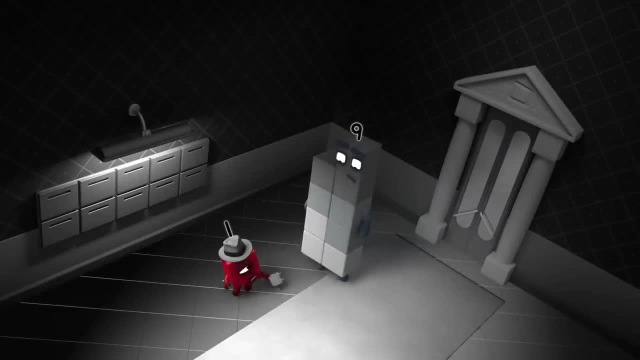 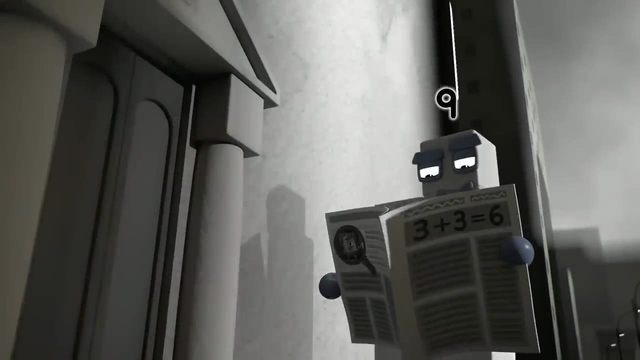 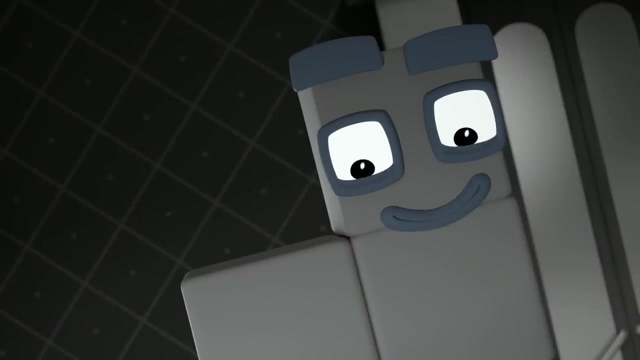 Did you notice anything strange or unusual when you got back? Er, no, No, Nothing. Oh, there was one thing: A suspicious, shadowy stranger in a coat and hat pushed past me and ran out of that door. But apart from that, nothing. 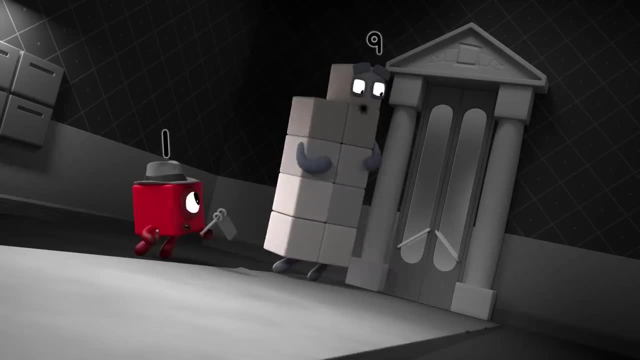 Can you describe this stranger? They were as wide as the door, so two blocks wide with a flat head. Clue: one Flat head when standing two blocks wide. Anything else I could see over their head when we were both two blocks wide. 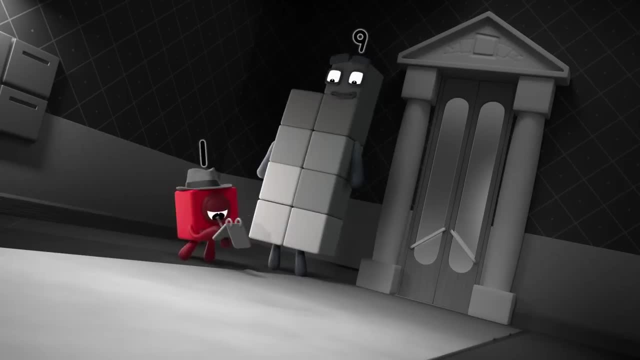 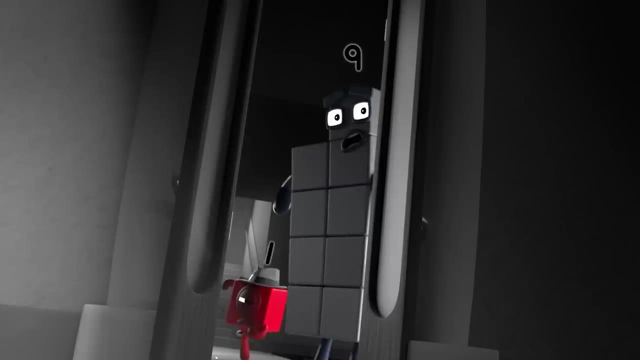 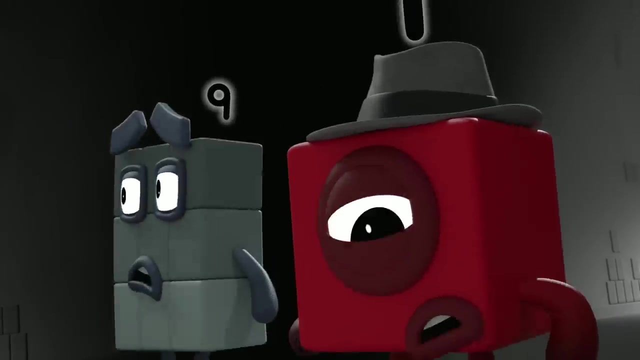 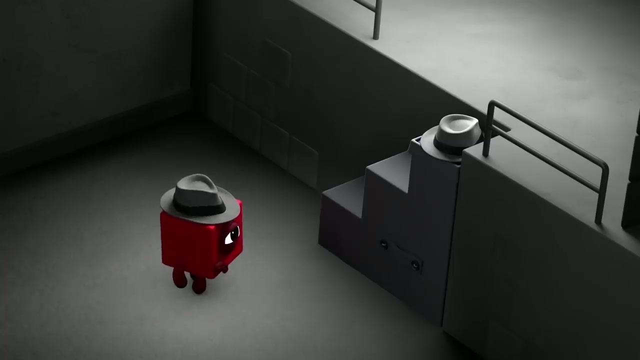 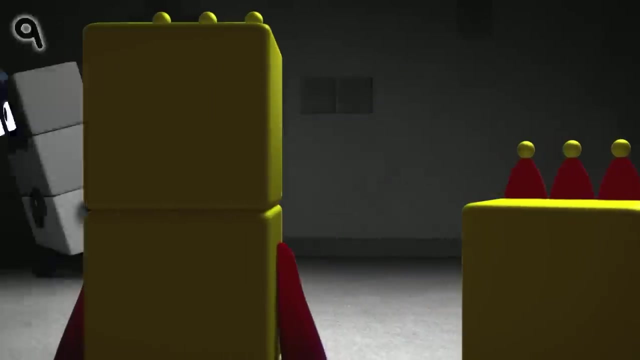 So they must have been smaller than me. Clue two, Smaller than nine. Look, Hat, Coat, It's them. After them, Quick There On the steps, The hat, These aren't steps, It's No. 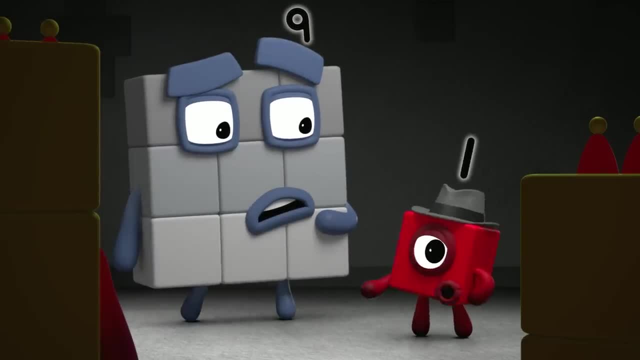 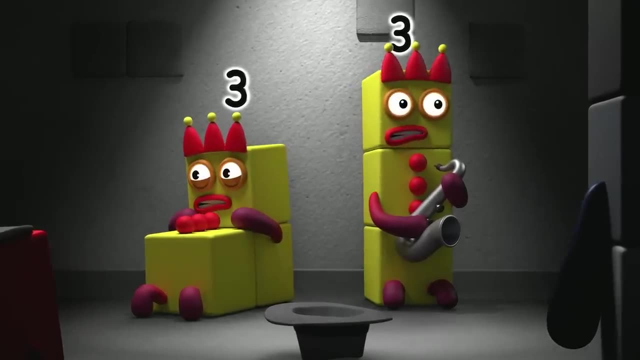 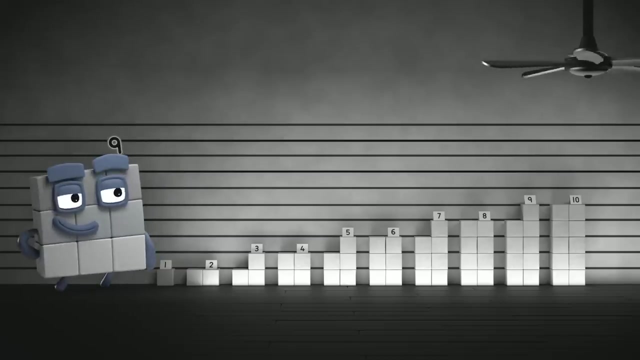 Did either of you see a suspicious step-shaped figure in a coat and hat? Sorry, friend, No one else down here, Just us. Something didn't add up, Or did it? Let's look at what we know. Clue one: 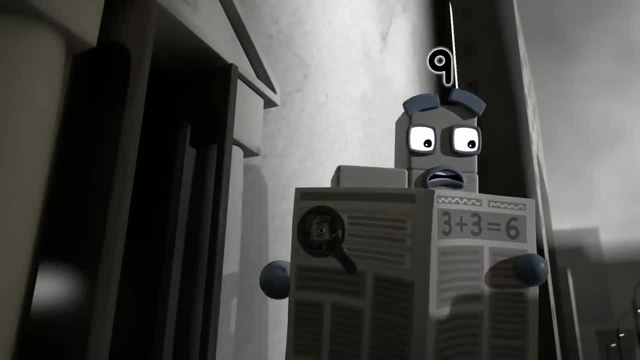 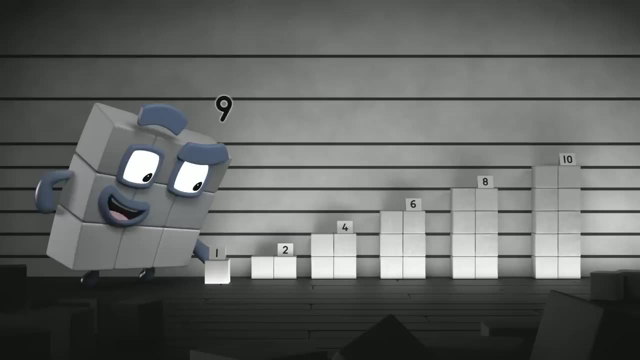 The suspect had a flat head when standing two blocks wide, So it can't have been three, five, seven or nine And it wasn't you, because you can't stand two blocks wide. Two, four, six, eight, ten. 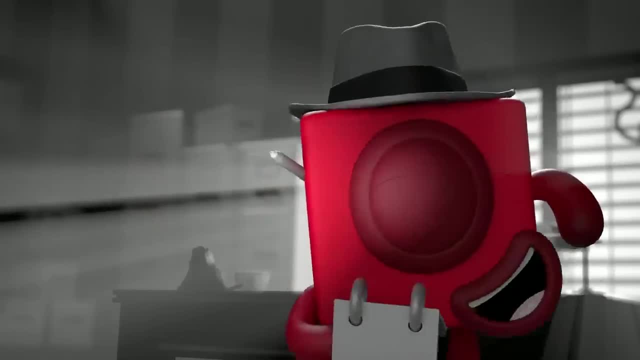 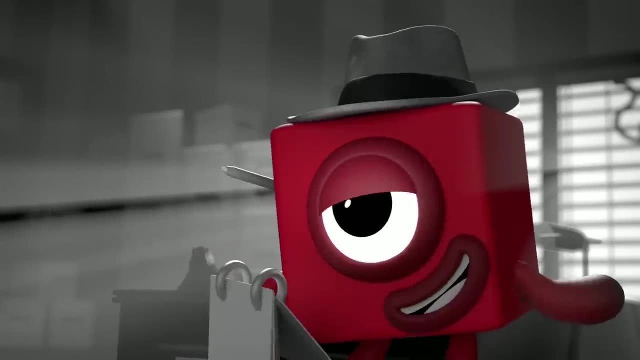 The suspect must be an even number. Bingo, And remember clue two. The suspect was smaller than nine, so it can't have been ten. That still leaves two, four, six and ten. Two, four, six and eight. 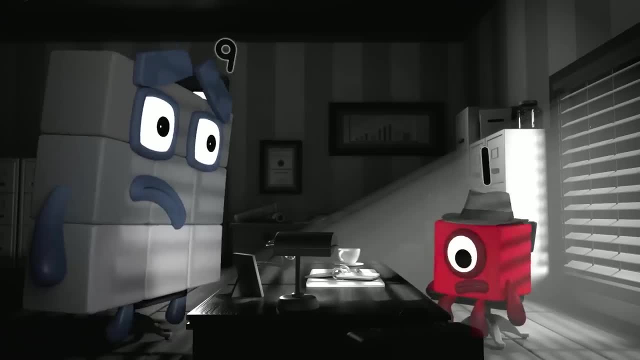 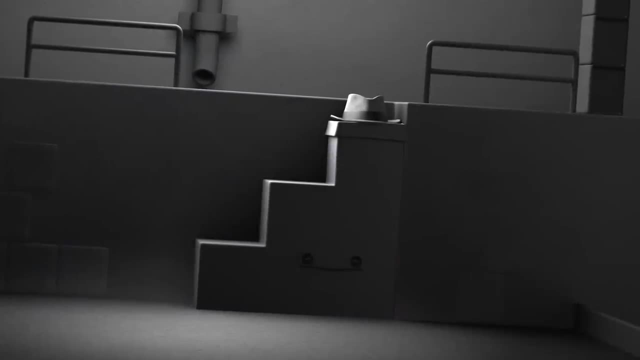 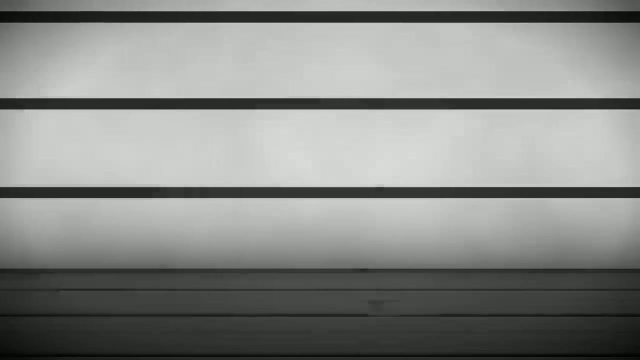 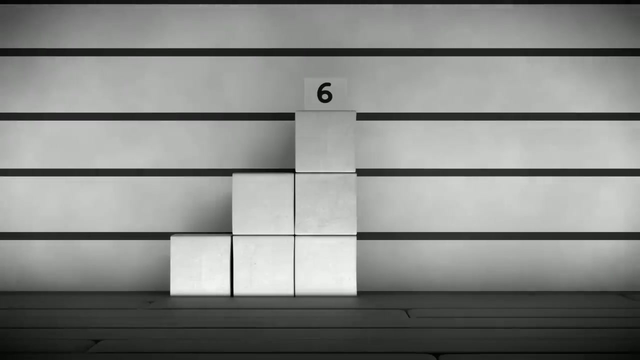 But which was it? Wait, There's one more clue, we nearly forgot: The suspect can make a step shape, Not two or four or eight, So it must have been Six. And who did we meet in the alley Three? 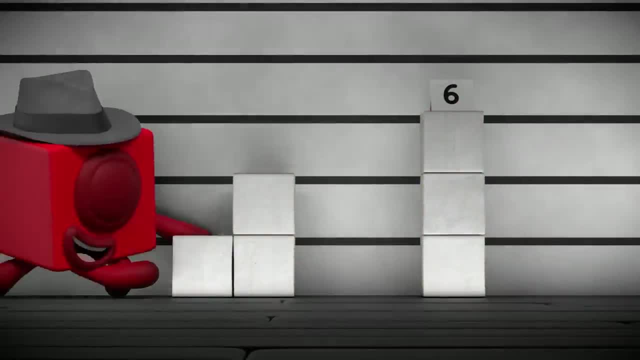 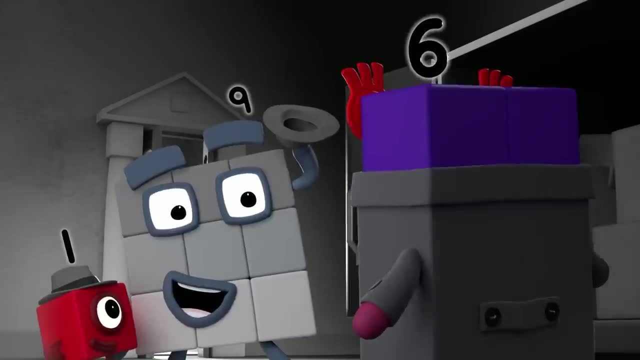 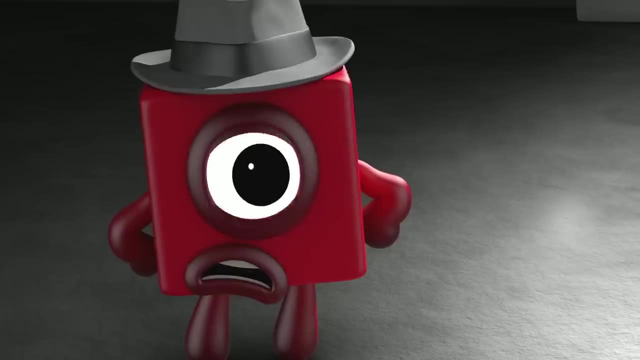 And another three Equals six. Stop Thief. Ha, You've got it all wrong. Oh, where to begin? I'm not taking these things, I'm moving them in, Moving in. Come up and I'll show you. 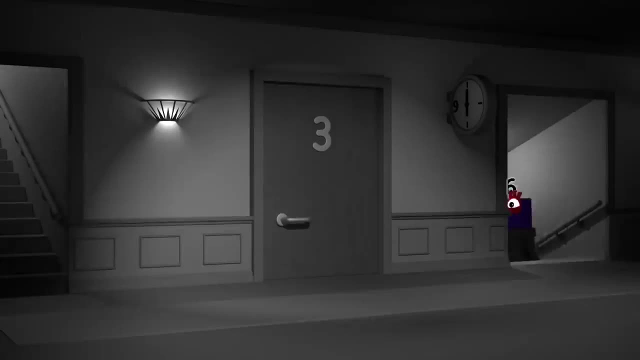 One, Two, Three, Four, Five, Nine. Wait, Nine doesn't come after five. This isn't apartment nine, It's apartment six. Look Number six turned upside down looks like a number nine. No one stole your things. nine. 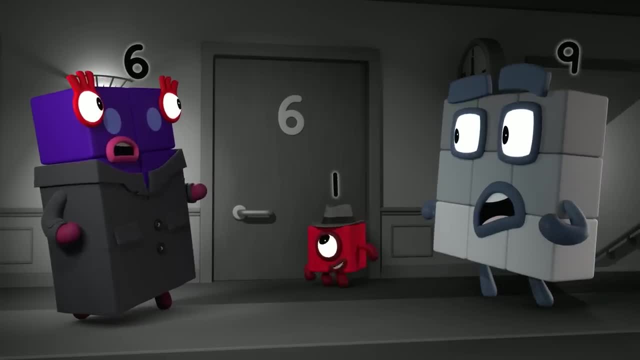 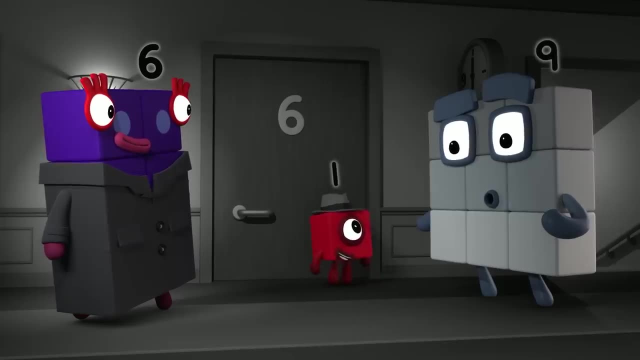 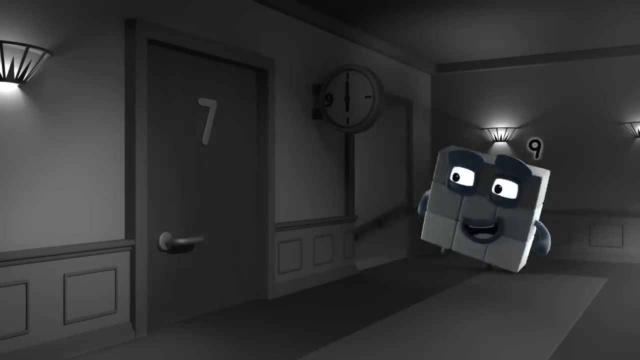 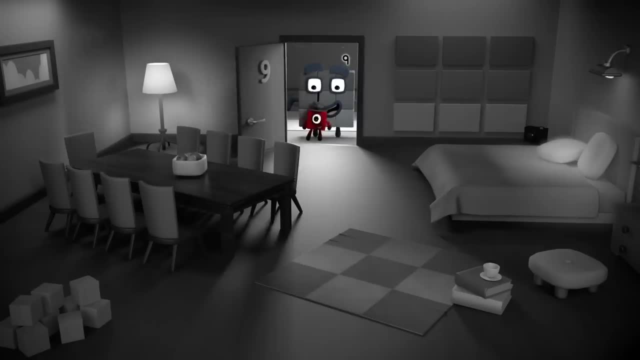 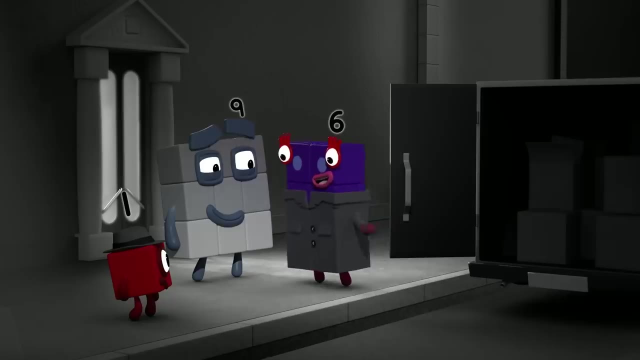 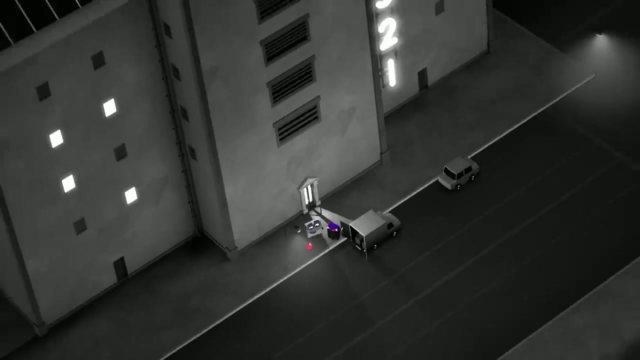 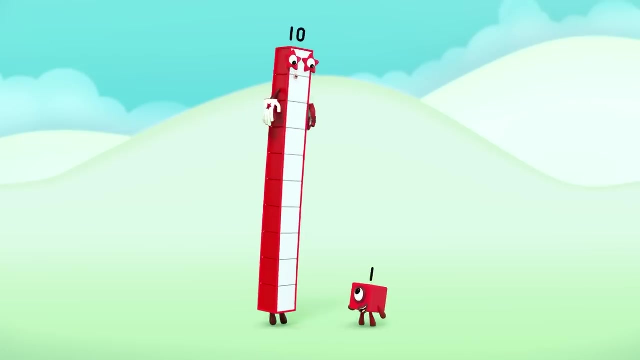 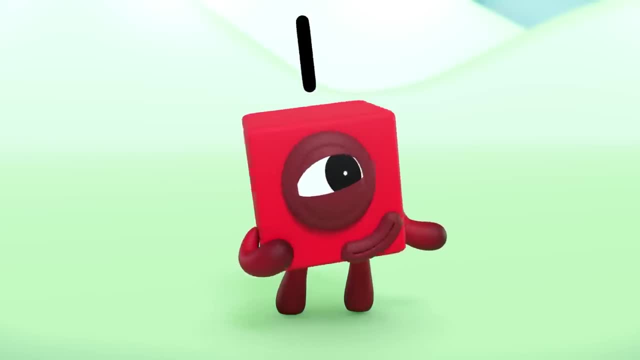 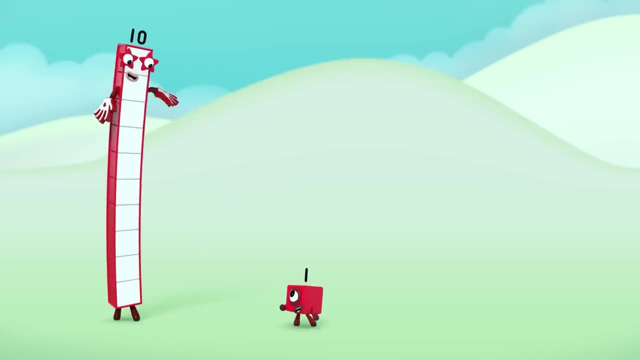 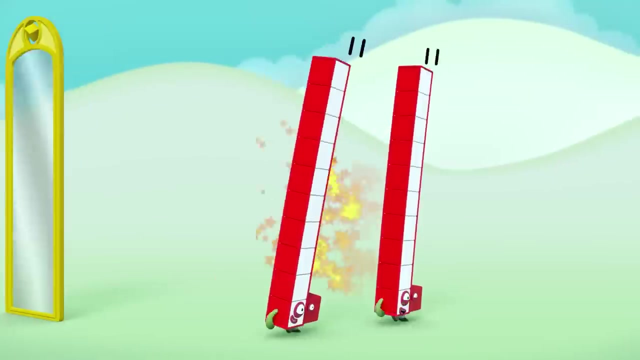 Ha, Oh, um, hmm, What was that? Who was that? A new number block 10 plus 1 equals 11!. Hello, I'm 11.. So am I, And I'm 10 and 1.. Oh, 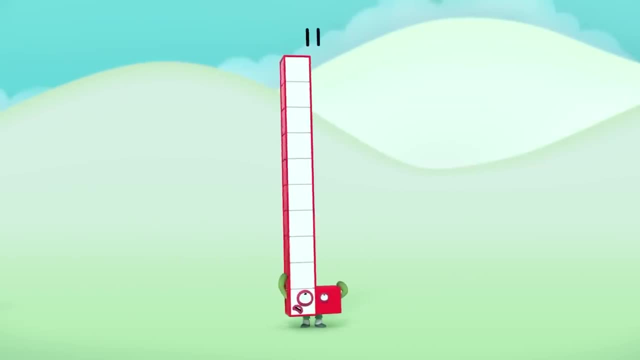 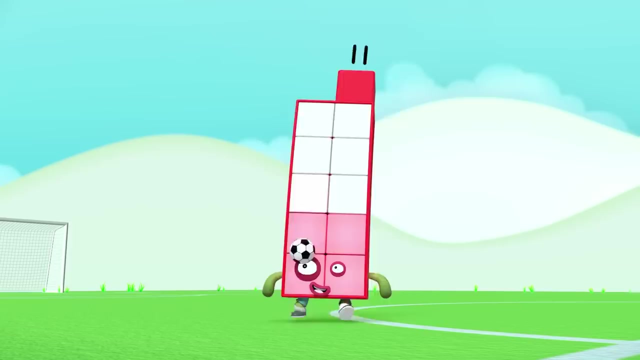 That's better. Oh Whoa, 1,, 2,, 3,, 4,, 5,, 6,, 7,, 8,, 9 and 10.. And one more is 11.. I am 11 and I love football. 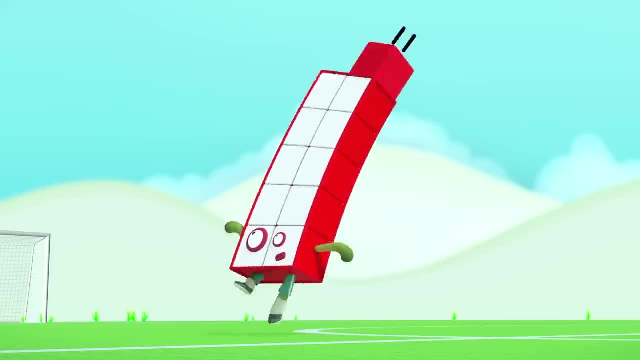 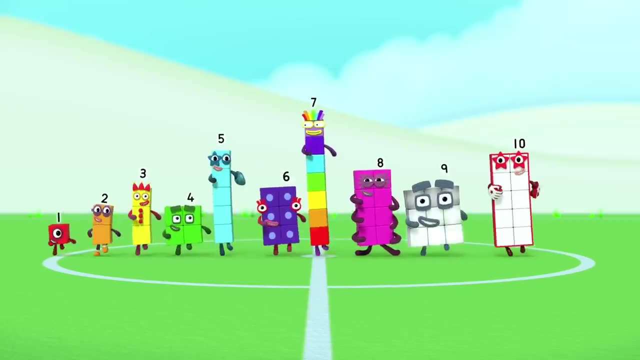 Whoa, Wow, Let's play football. Hooray, Yeah, Hooray, Hooray, Hooray, Hooray. 1,, 2,, 3,, 4,, 5,, 6,, 7,, 8,, 9 and 10.. 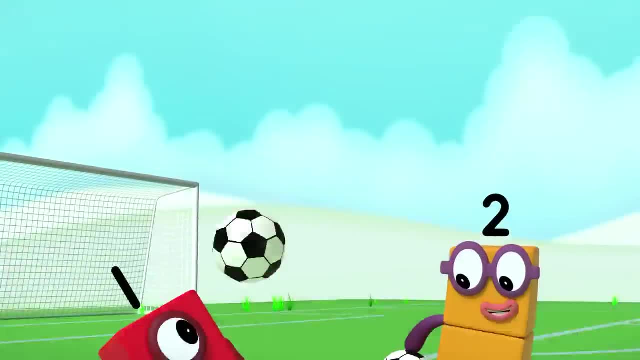 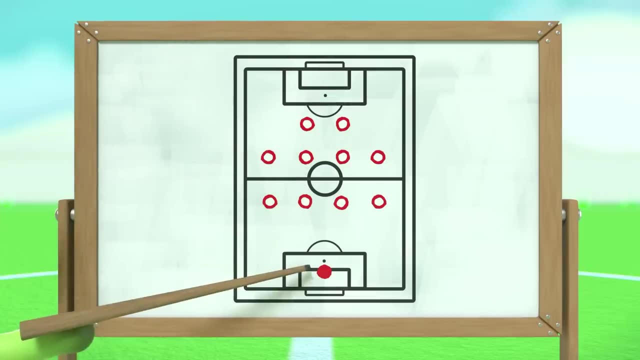 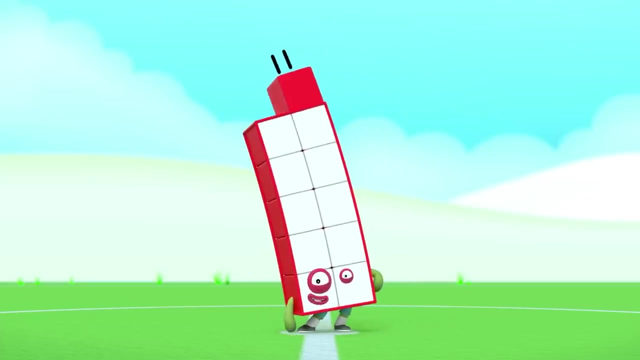 And one more is 11.. We're on our way to victory. We're on a roll With 10 on the pitch and 1 in goal. We will never be denied. We'll take it in our stride With 10 and 1, 10 and 1, 11 on our side. 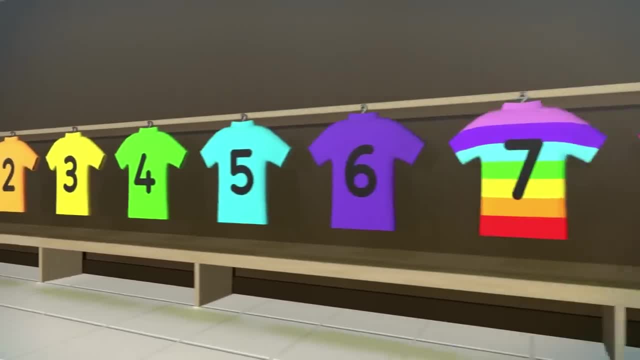 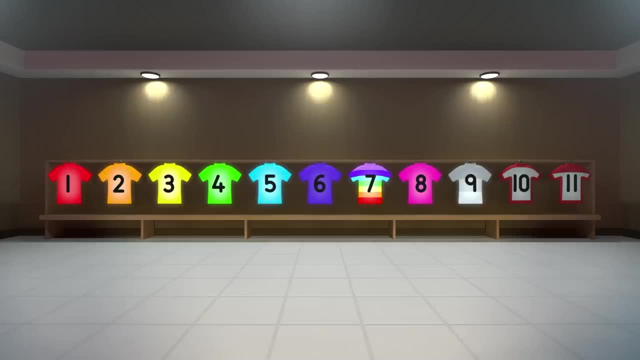 Football shirts. Football shirts, One for every number. block Football shirts: 1,, 2,, 3,, 4,, 5,, 6,, 7,, 8,, 9 and 10.. And one more is 11.. 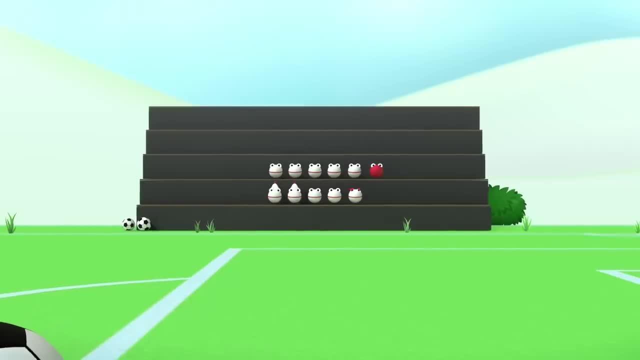 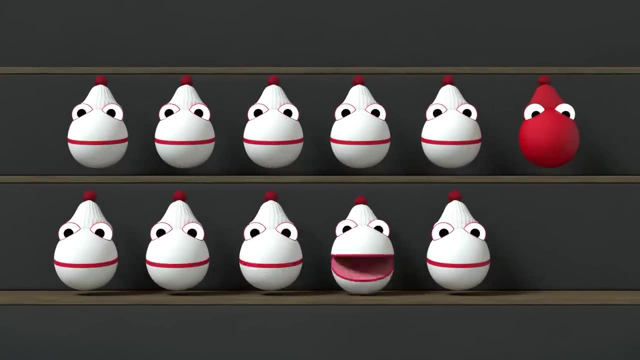 Hooray, Bubble hats. Bubble hats, One for every number. block Bubble hats 1,, 2,, 3,, 4,, 5,, 6,, 7,, 8,, 9 and 10.. And one more is 11.. 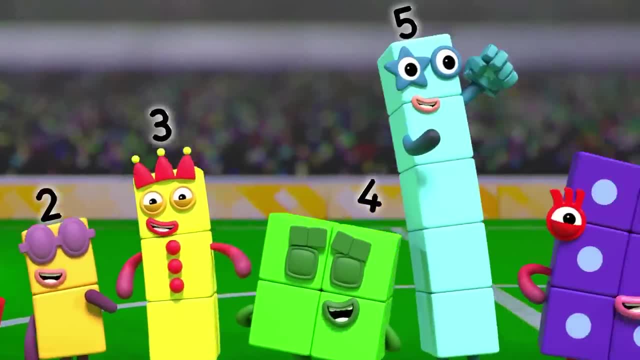 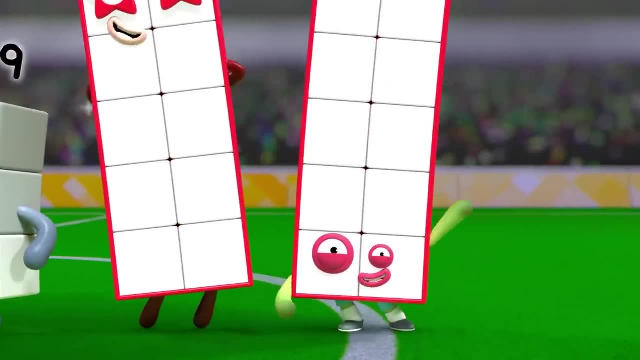 Hooray, Hooray, Hooray, We're on our way to victory. We're on a roll, With 10 on the pitch and 1 in goal. We will never be denied. We'll take it in our stride. 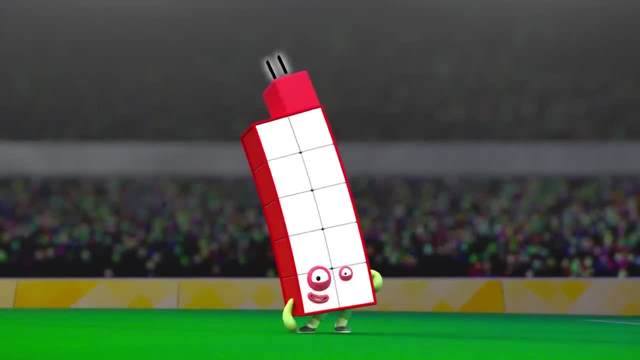 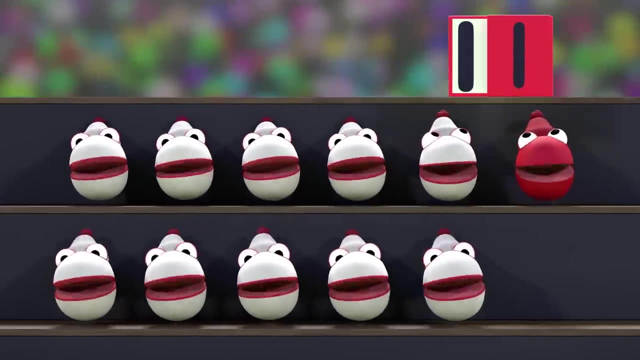 With 10 and 1, 10 and 1, 11 on our stride: 1, 10.. 1, 1. 10. And 1. 11. 1, 10. 1, 1.. 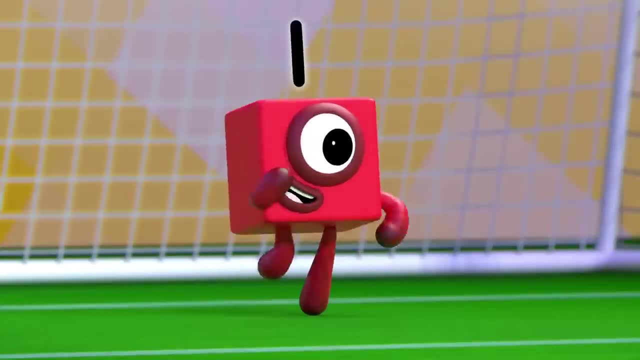 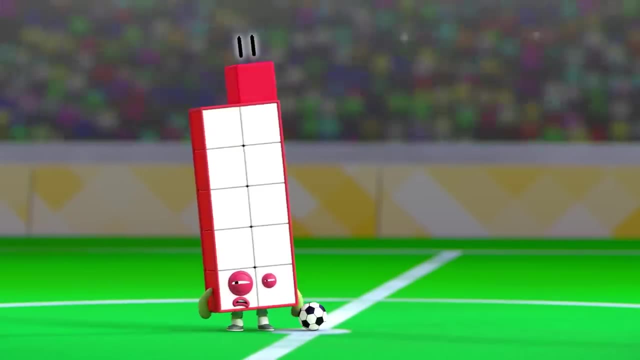 10. And 1. 11.. The number blocks are out on the pitch for the big match And their captain, 11, looks ready to leave. Looks ready to lead the team to victory. Something's wrong. What can it be? 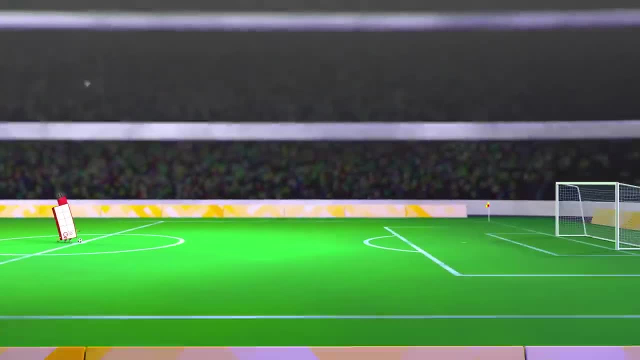 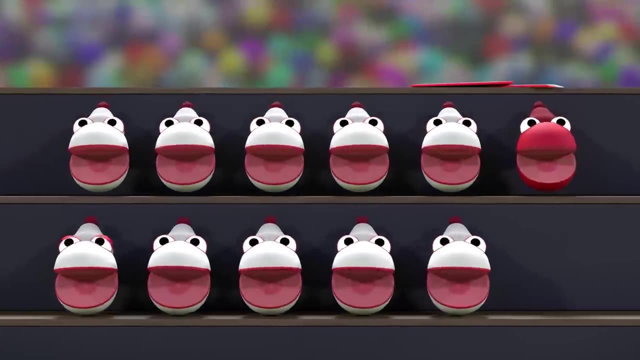 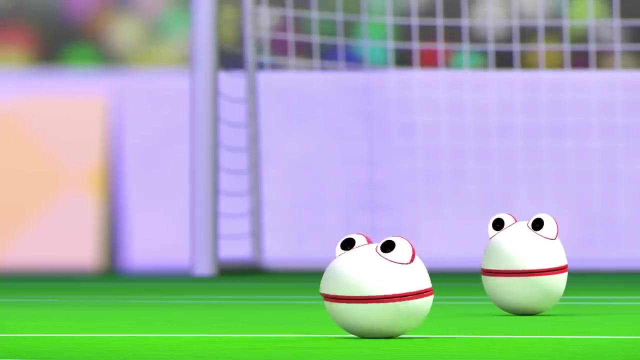 I've forgotten something. Huh, The other team, Oh, Oh Oh, We need 11 more players. Number blocks Game on And the number blocks have kicked off. It goes high towards the goal And saved by one. 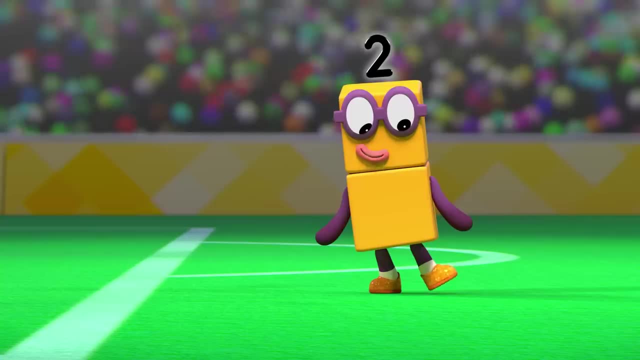 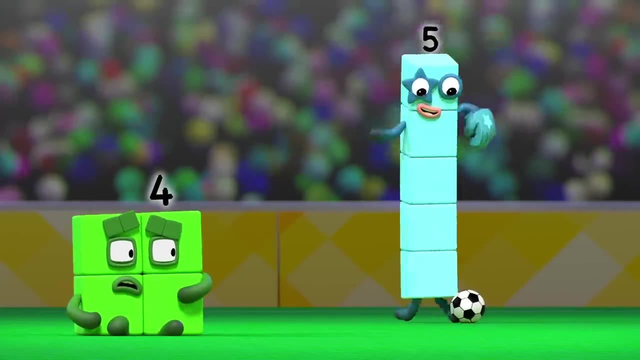 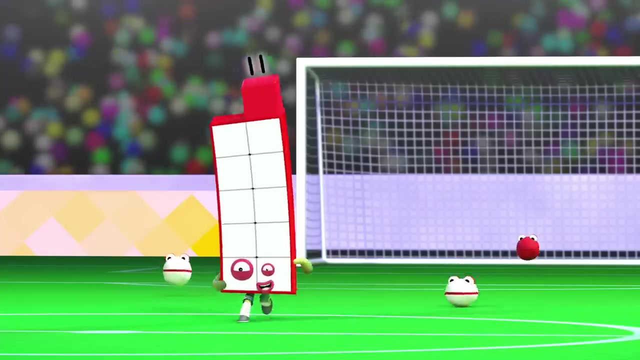 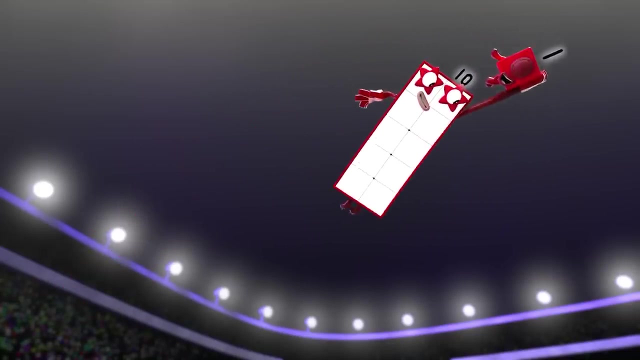 Take a bow, one. One throws it out to two. who passes it? that's right to three, four, five, six, seven, eight, nine and ten. Now pass it to eleven. Ten passes, eleven seats for the header and, oh my, splits into ten and one to reach the ball. 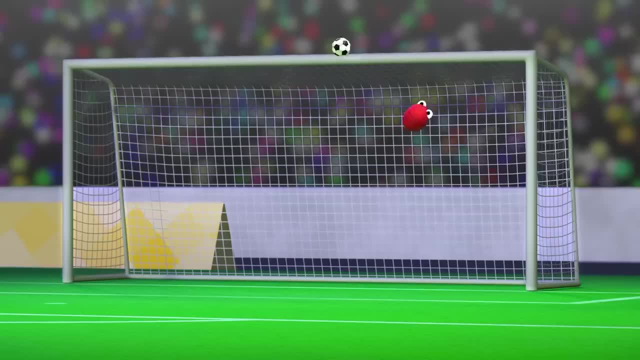 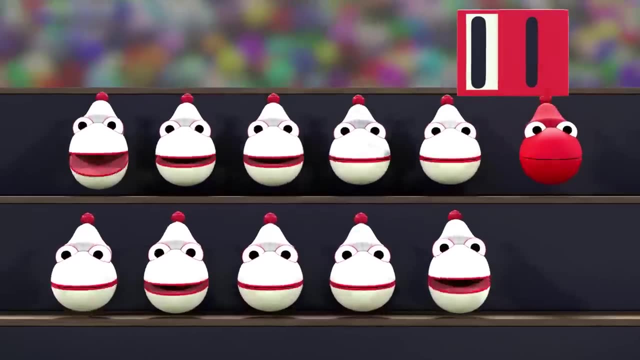 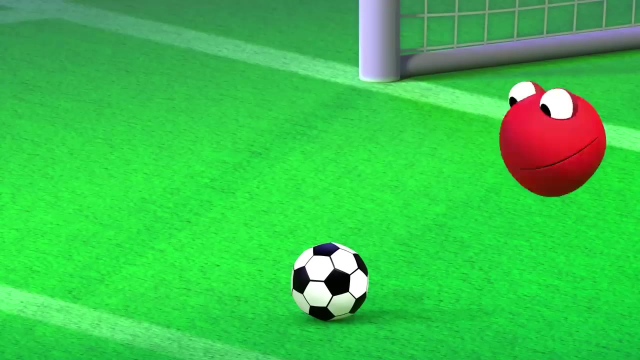 Incredible, And it's a save. What a save. Cut it up to eleven. you're too loud to sound the rest Ten and one. ten and one eleven is the best Number blob. passes to number blob to find number blob. 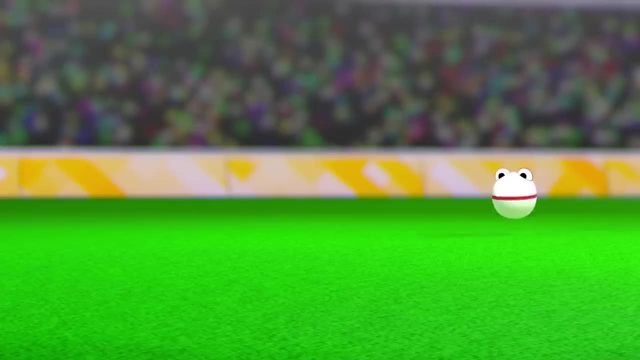 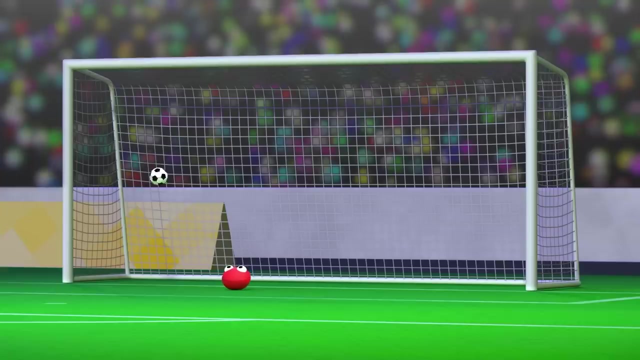 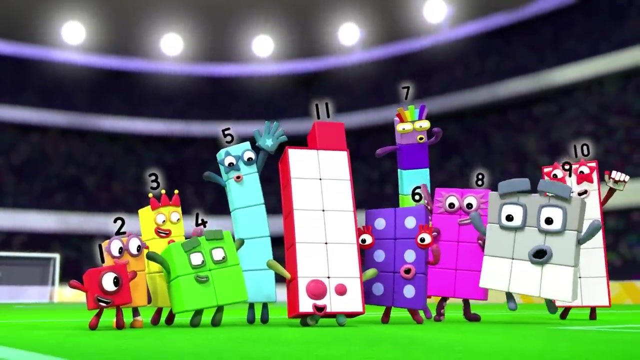 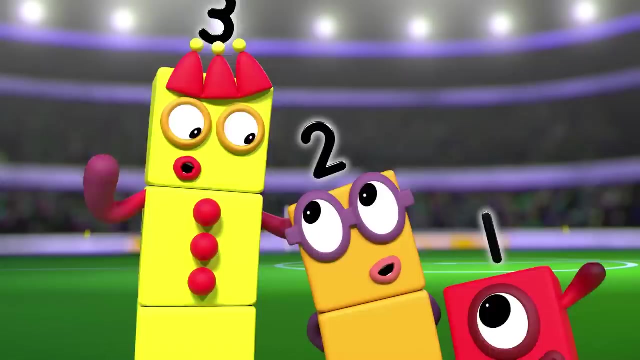 And a lovely header there to number blob Eleven. He heads it to eleven And it's eleven, Eleven, Eleven. We're on our way to victory. we're on a roll With ten on the pitch and one in goal. We will never be denied. we'll take it in our side. 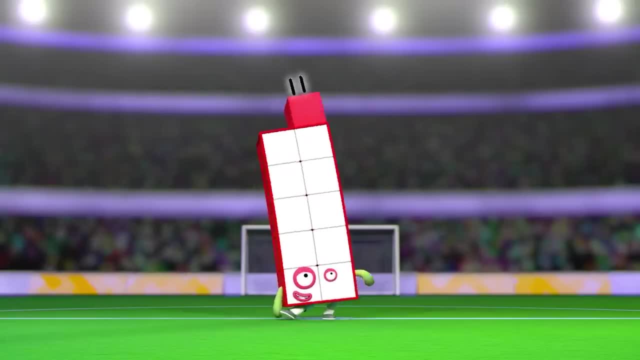 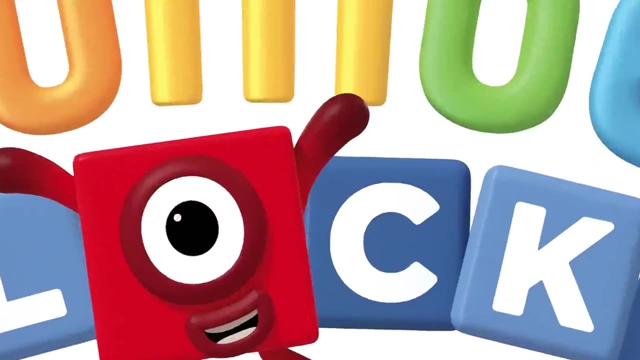 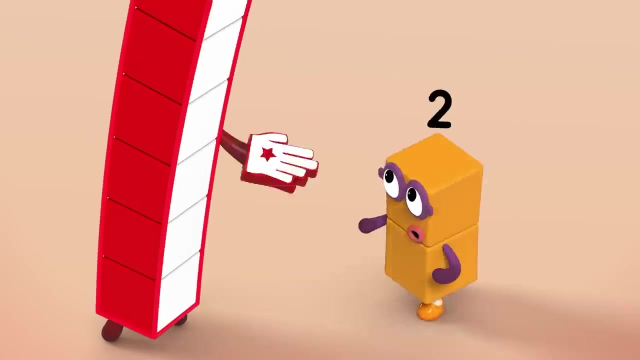 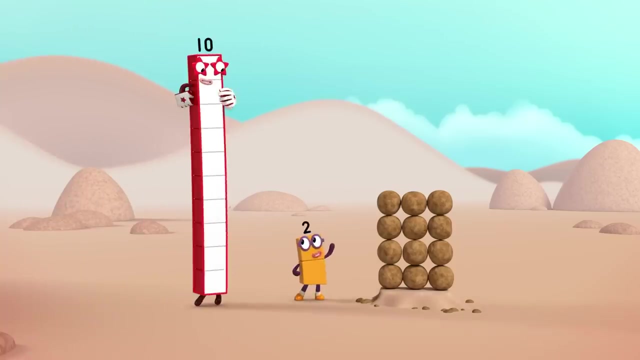 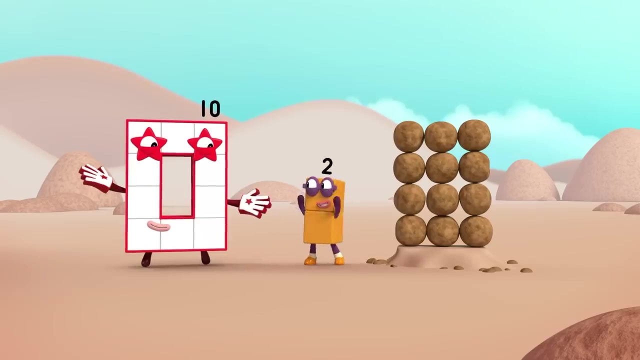 With ten and one, ten and one, eleven on our side. Ten and one, ten and one, eleven on our side. Yay, Ten and two, Ten and all. Look at that. Hey, what am I? A rectangle with a hole. 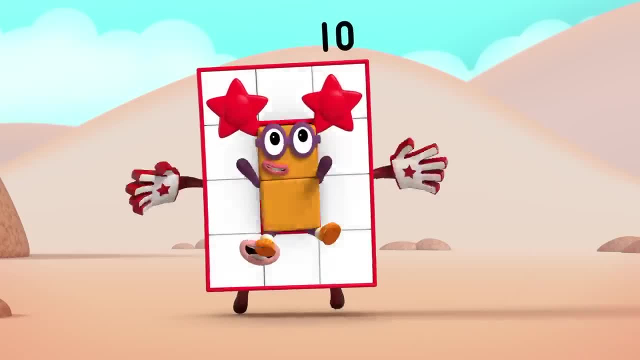 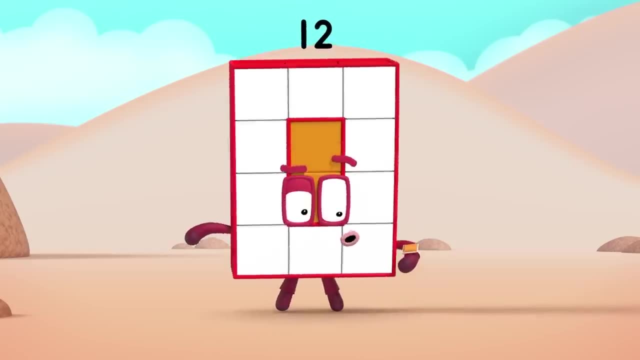 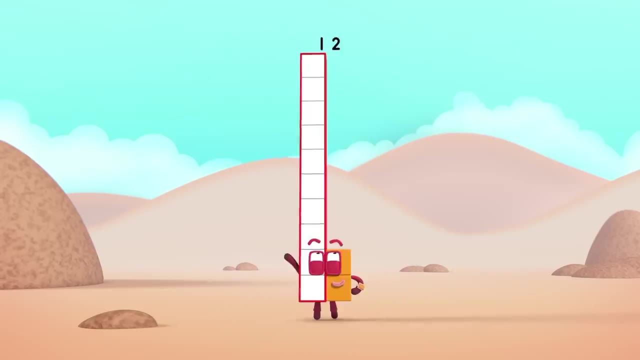 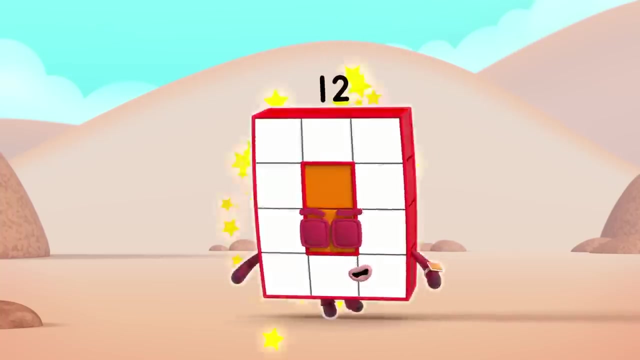 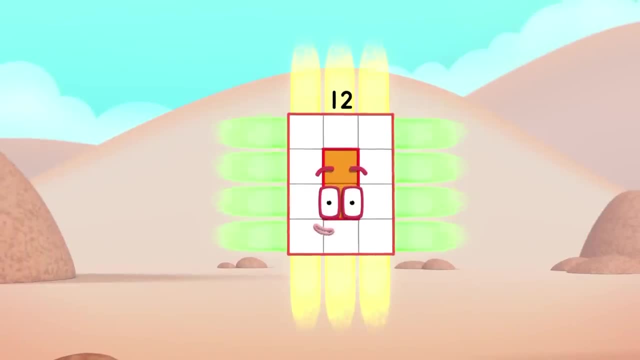 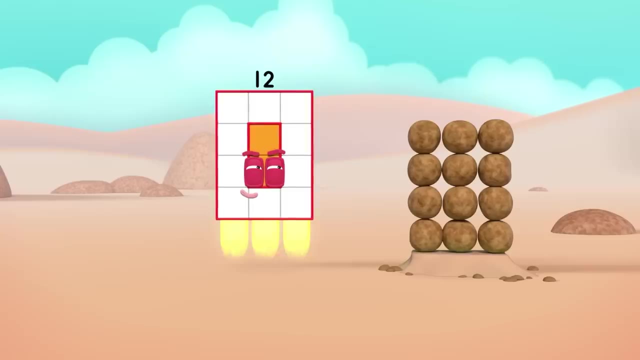 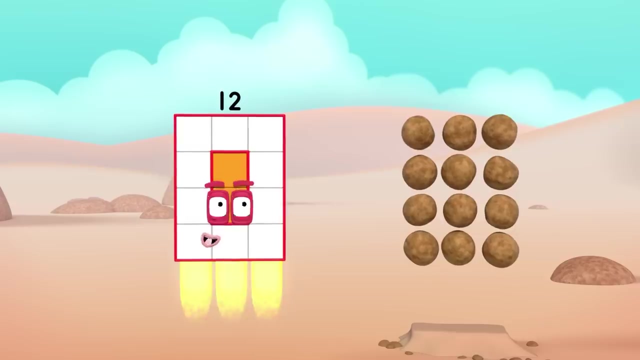 And I am a super rectangle, Super rectangle. and I made a great double: One, two, three, four. I'm twenty And I'm twenty-two. I am fifty: One, two, three, four and I'm ten. 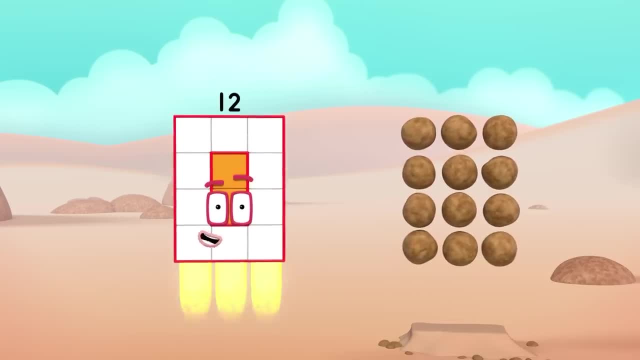 And I'm twenty-two When I'm not short. I'm you sorry, I'm twenty-two, Oh, I'm twenty-two. I'm workers in my job. You stand only one. You and me live in one frame. No. 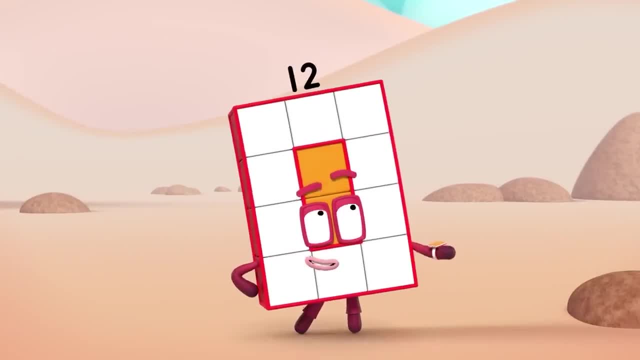 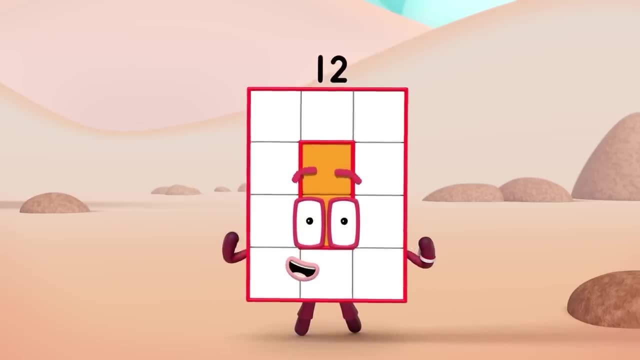 No, The rocks are in columns and rows, My blocks are in columns and rows And that's called an array: Arrays, Ro're, Hey, Whoo, I'm rectangular twelve. I make an array and my rectangle goes like this: 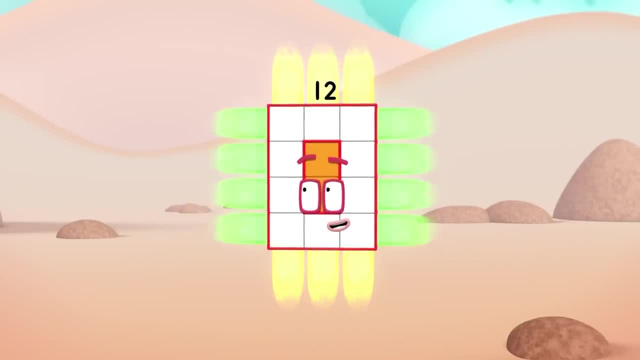 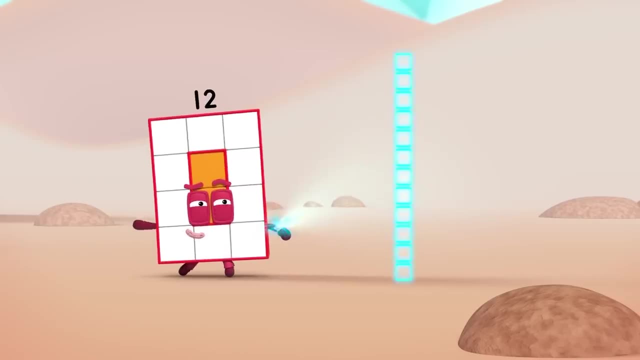 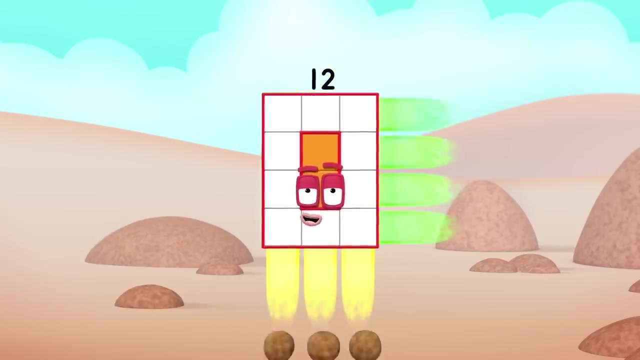 Three by four. Today's the day for an array display. I can make arrays all day. I make arrays in many ways. Stand back, let's play arrays away. Three by four is my first array. Three, lots of four, you could put it that way. 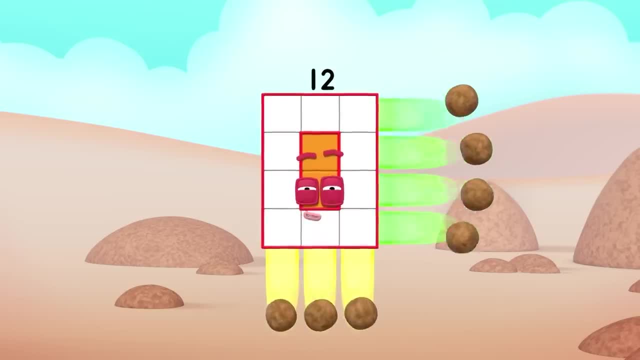 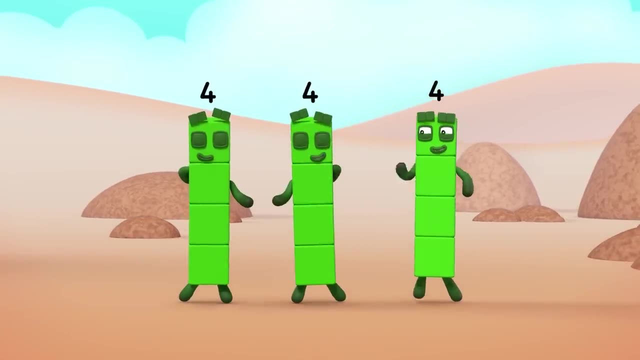 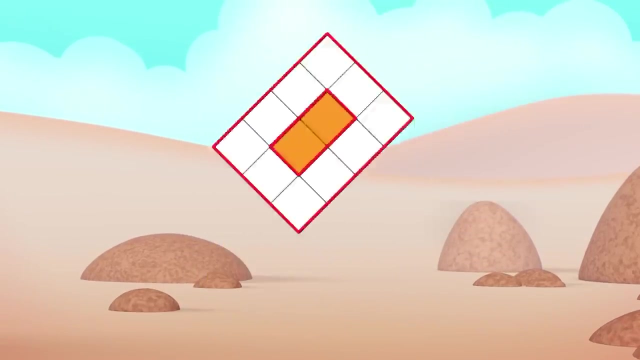 And if you're not following what I say, I'll rectify that right away. Breakaway: Three, fours, A four and a four and a four. Rectangle rise Turn. I'm rectangular 12,, I'm 10 and 2.. 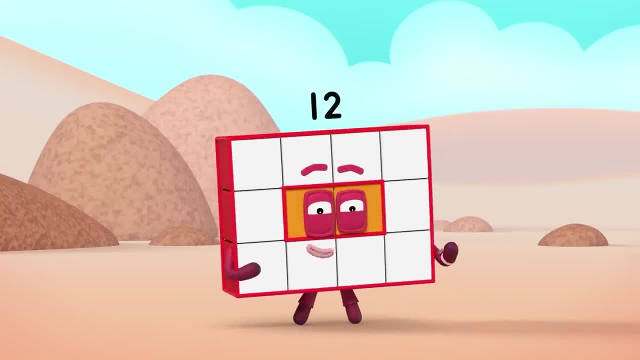 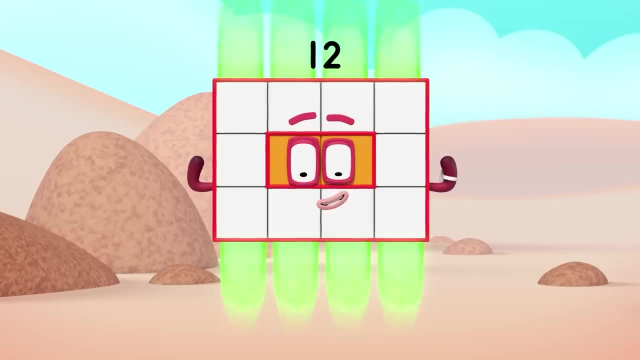 I make arrays. that's what I do When I put my blocks in columns and rows. I make an array and my rectangle goes like this: Four By three, Four by three's. my next array: Four, lots of three. you could put it that way. 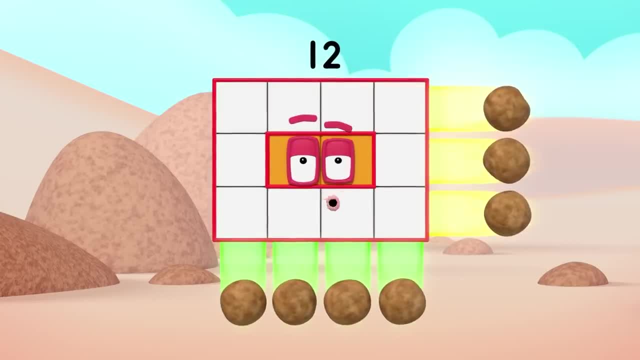 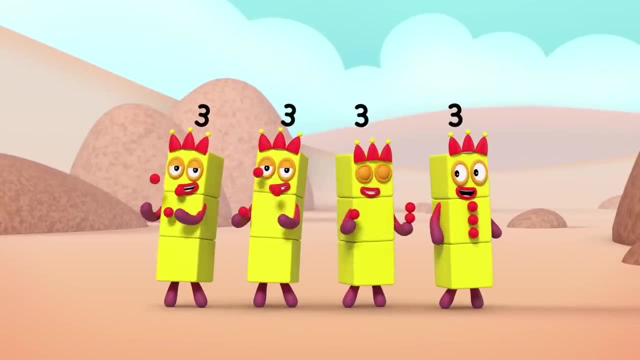 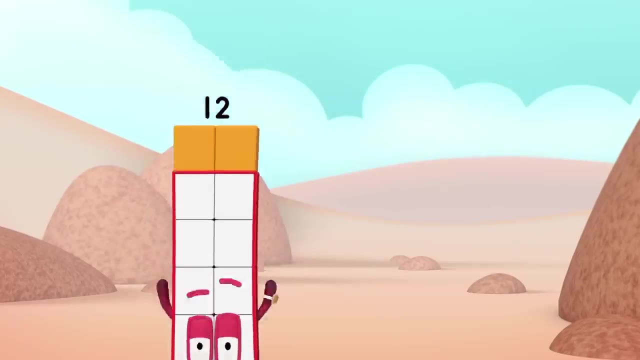 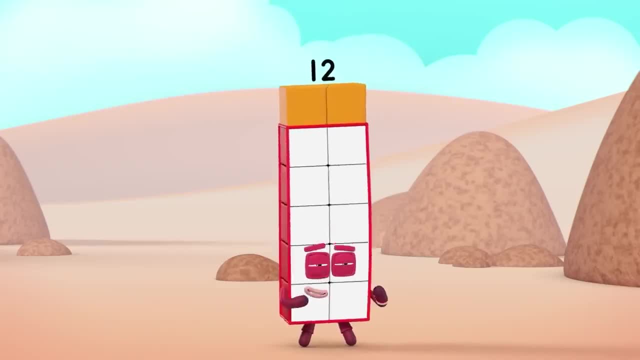 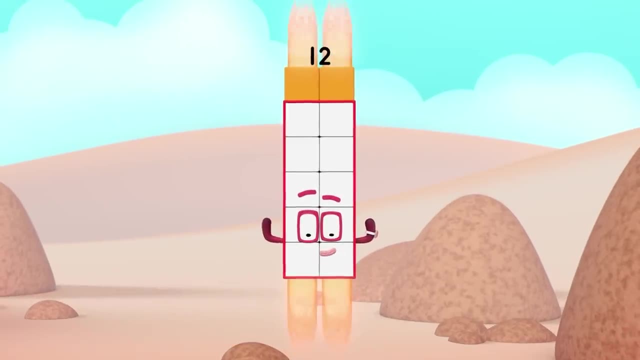 I make arrays. that's what I do When I put my blocks in columns and rows. I make an array and my rectangle goes like this: Two By six. Two by six is another way: Two, lots of six. do you hear what I say? 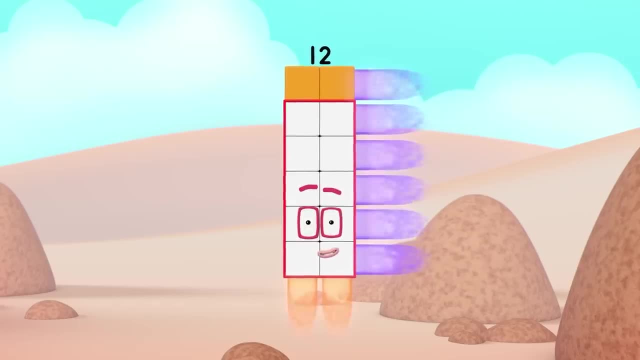 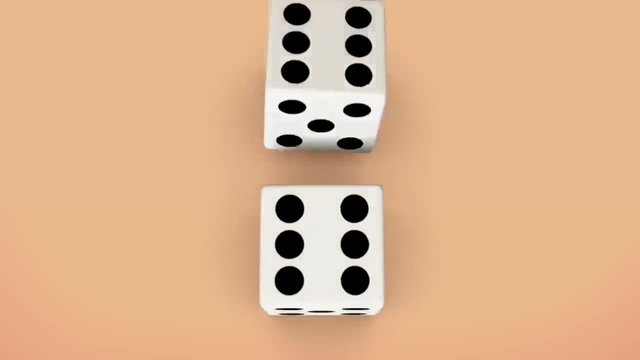 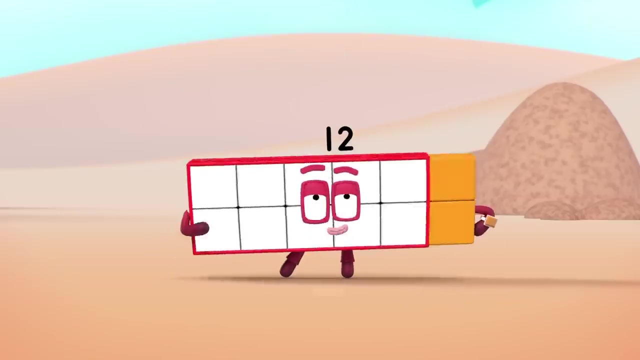 Another rectangular array. So let's split Without delay. Breakaway, Two sixes. Let's roll Double six Turn. I'm rectangular 12, I'm 10 and 2.. I make arrays. that's what I do. 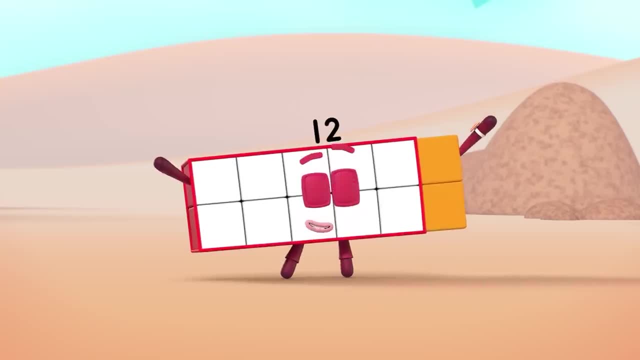 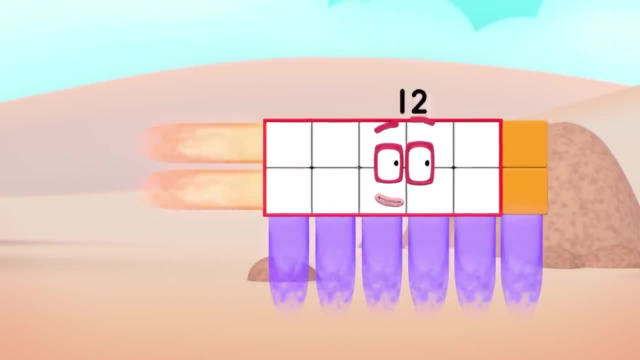 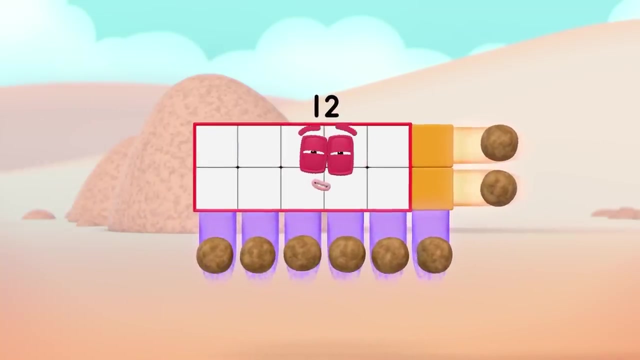 When I put my blocks in columns and rows, I make an array and my rectangle goes like this: Six By two. Six by two is next in line Six, lots of two. it's a clever design, And if you want to see how all this fits, 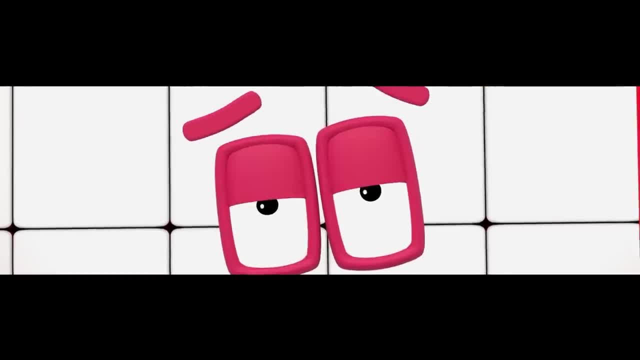 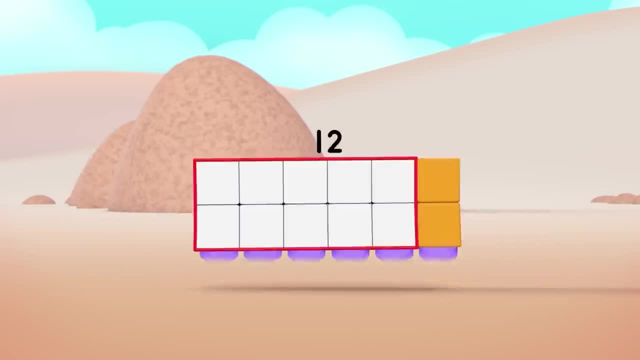 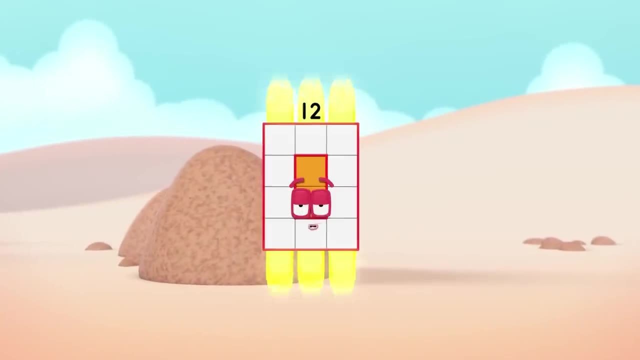 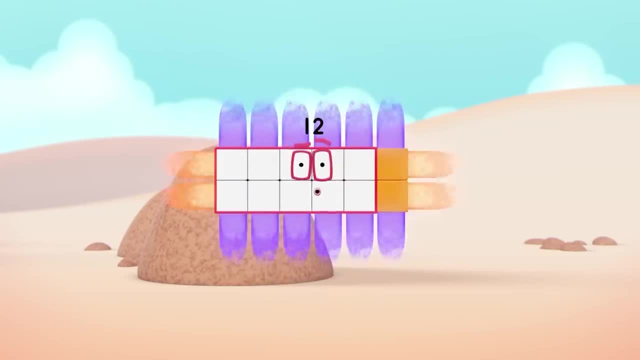 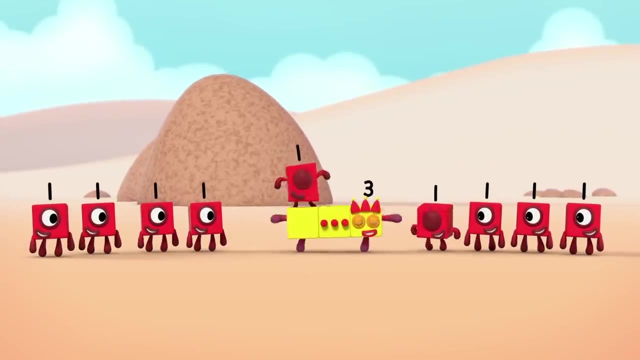 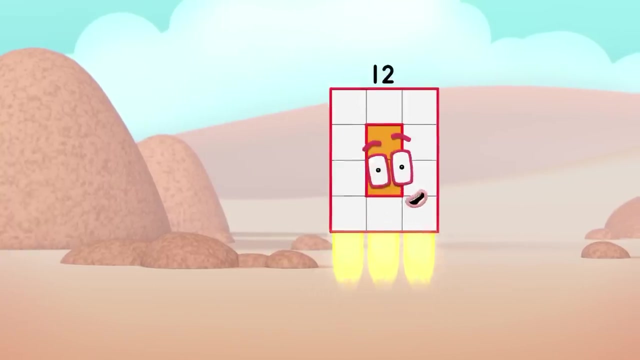 By four Turn Four. By three Switch Six. By two Switch Twelve. By one Breakaway Turn one, One, Two, Turn Eleven, Twelve- It's a new crazy coin of phrase. You'll be in a daze when you fix your gaze on my amazing array displays. 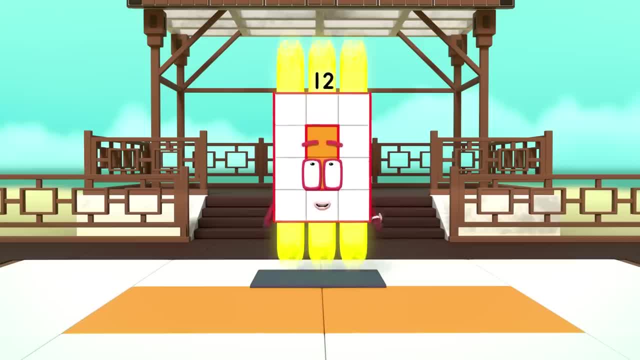 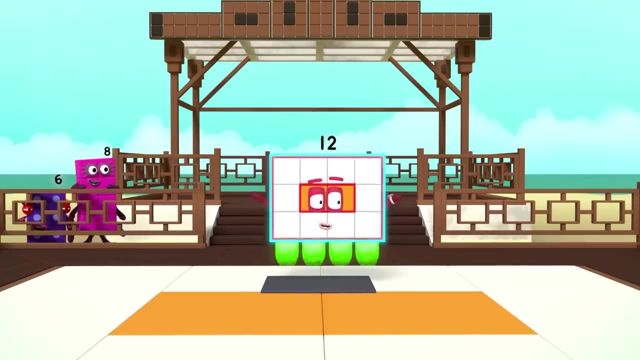 I am 12.. I am three by four. I am a rectangle Turn. I am also four by three, Ooh Ugh. And I am a super rectangle. I can take many forms, Switch. I am six by two. 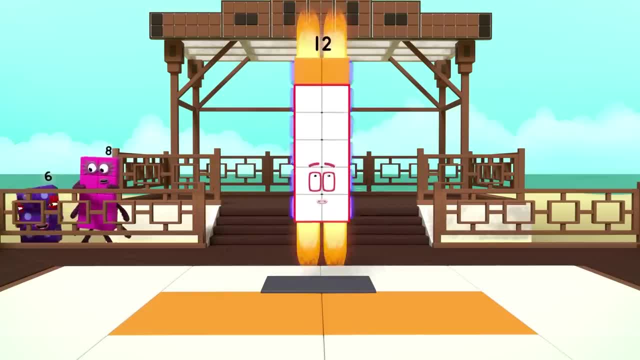 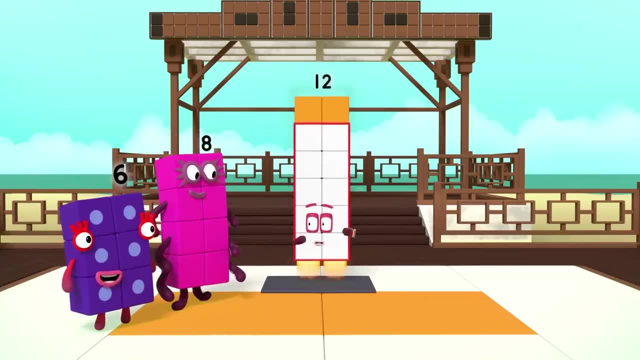 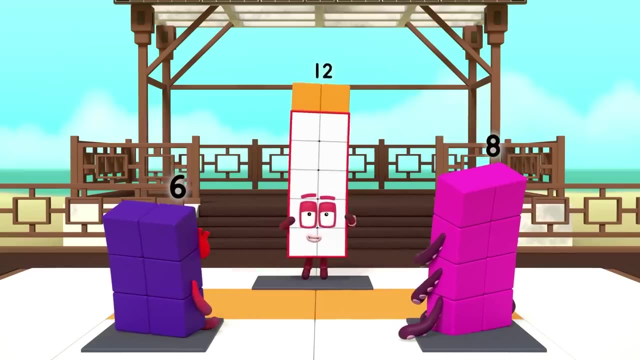 Turn. I am two by six. I am a rectangle. Welcome, my friends. Would you like to master the way of the rectangle? First you need to stand, so your front makes a rectangle shape. Rectangle shape. watch and tell me when I'm making a rectangle. 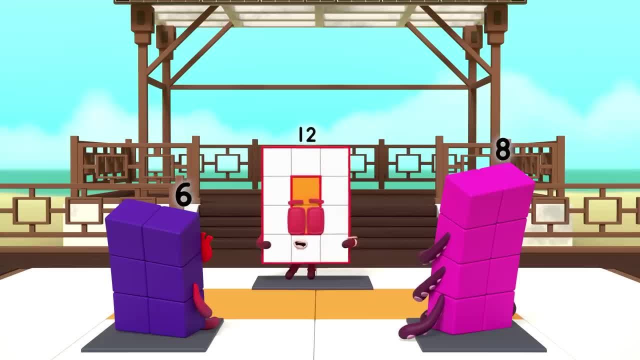 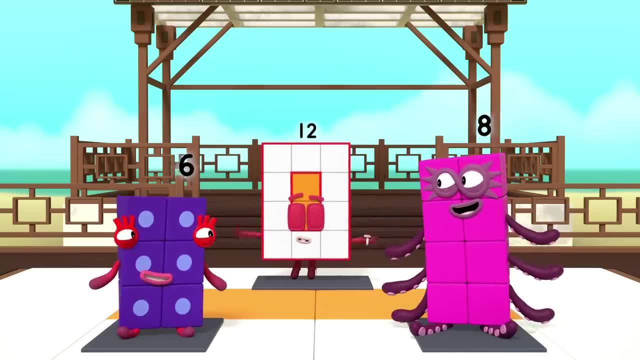 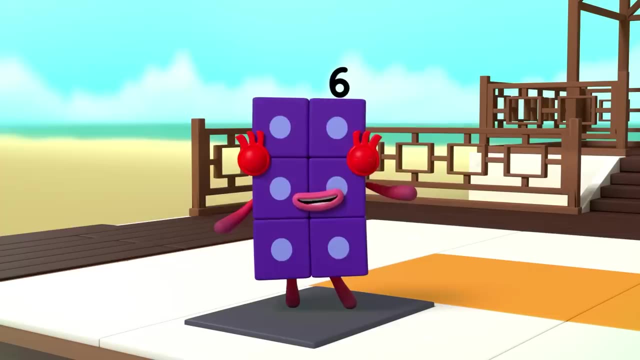 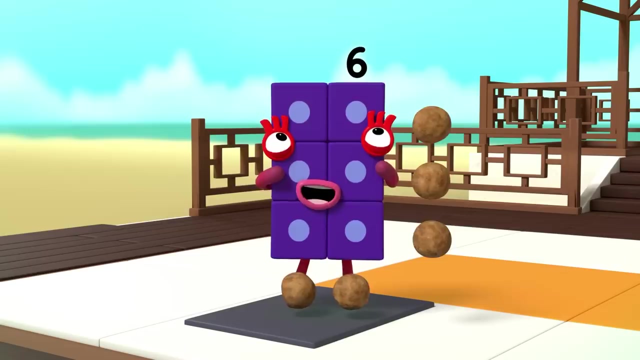 Well done. now look at your own fronts. what shape are you making? That's right. your blocks are arranged in neat columns and rows. now Concentrate on how wide you are. I am six. I am two blocks wide. by Three blocks tall, I am two by three. I am a rectangle. 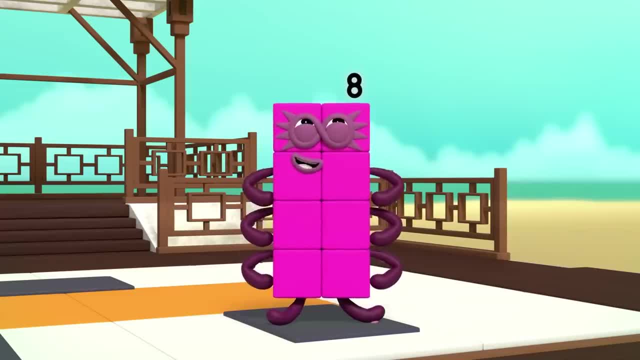 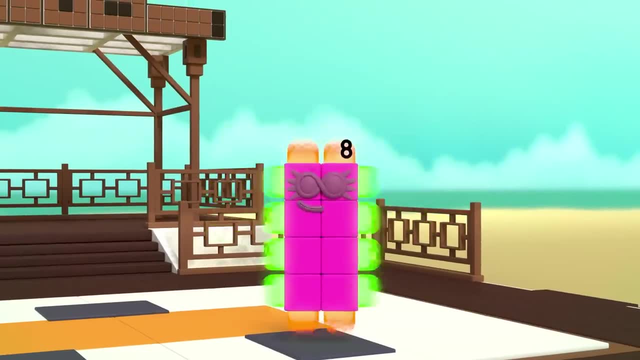 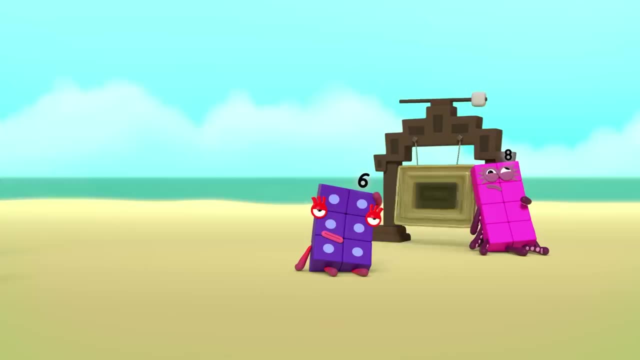 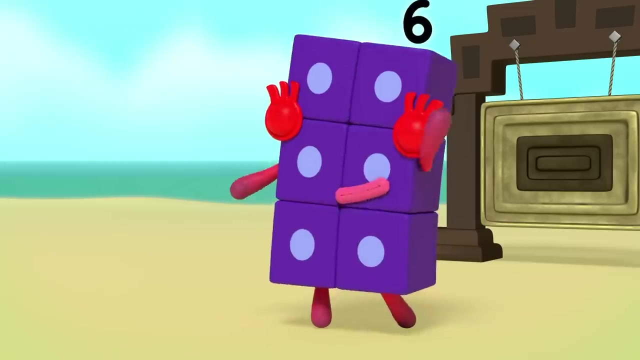 I Am eight. I am two blocks wide by four blocks tall. I am two by four. I am a rectangle up. up and away I Heard a ban. are you okay? six, I'm more than okay. I've mastered the way. Hey, where are my rays? 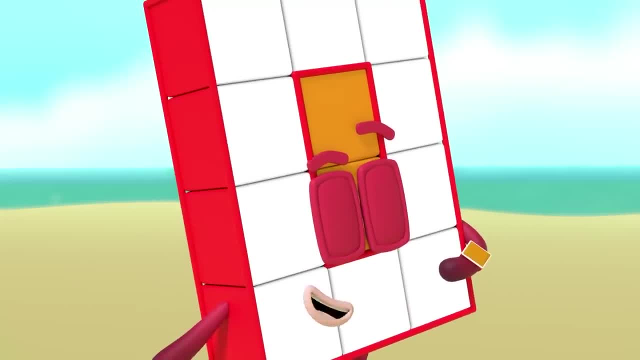 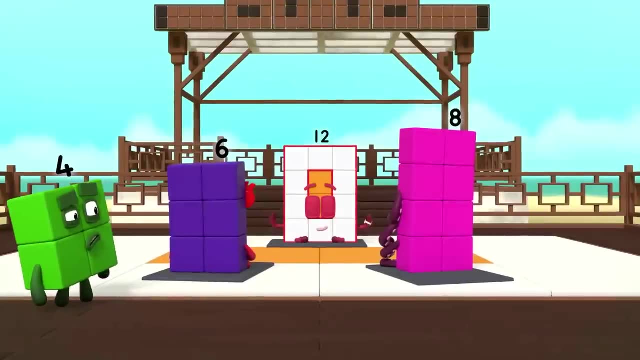 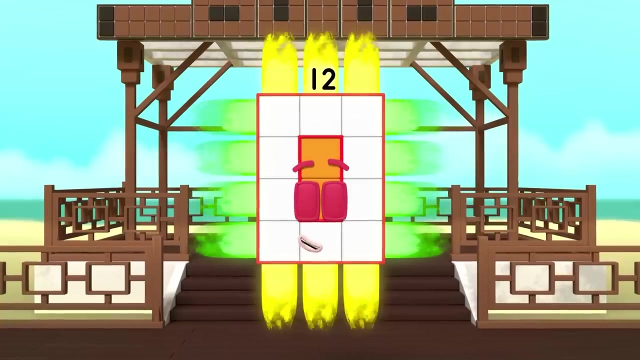 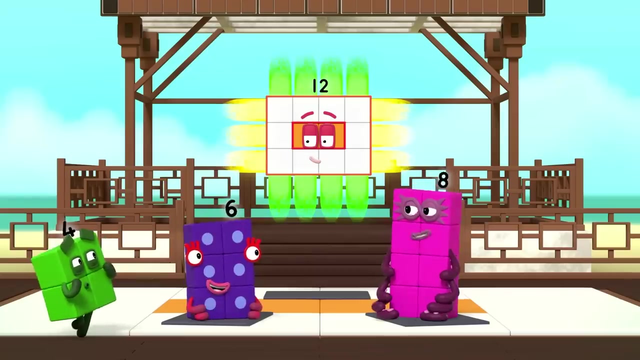 You need to concentrate. it gets easier with practice, So let's practice. It's time for the turn. I Am 12, I am three by four, Which means time. I am also four by three. See who I Am six. I am two by three, which means ten. I. 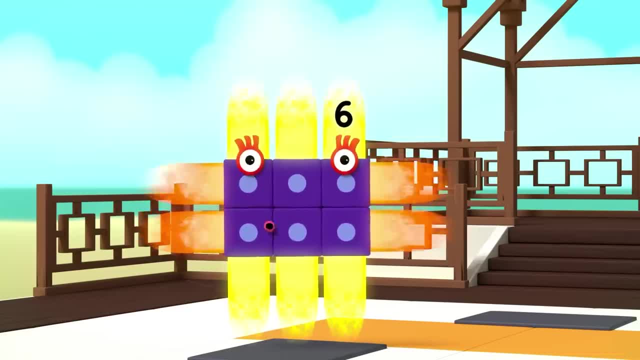 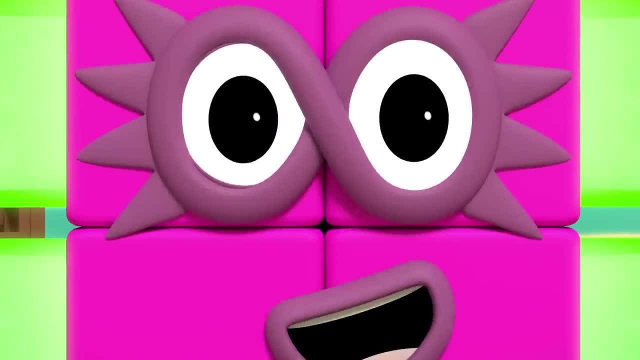 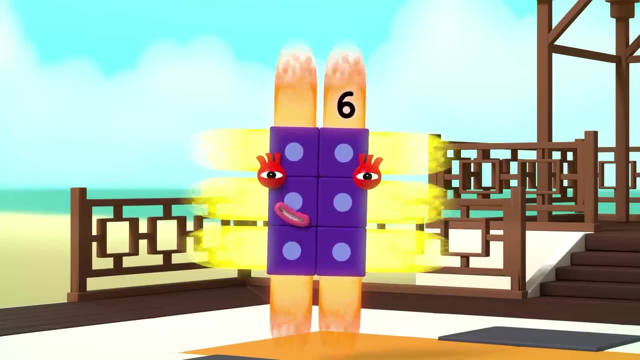 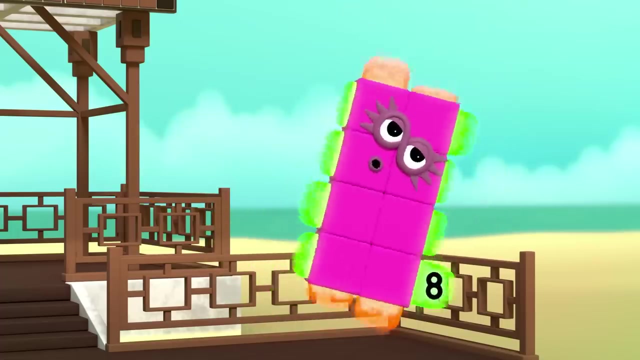 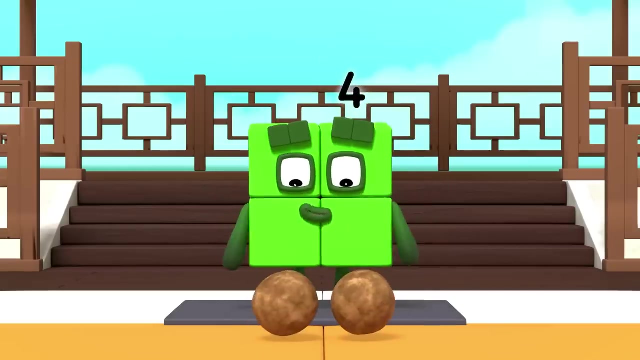 am also three by two. I Am eight. I am two by four, which means octoblock turn. I Am also four by two Ten. two by three ten, three by two, ten ten. Oh, Let me try that. I am four. I am two blocks wide by two blocks tall. I. 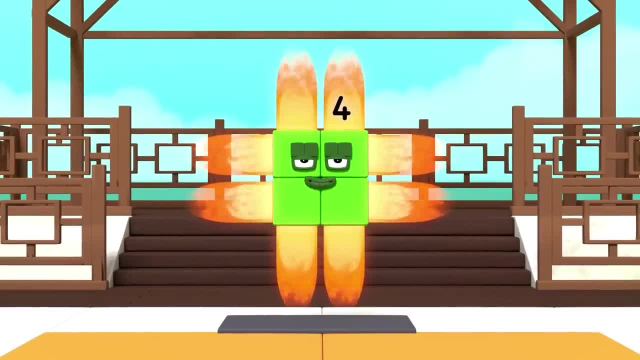 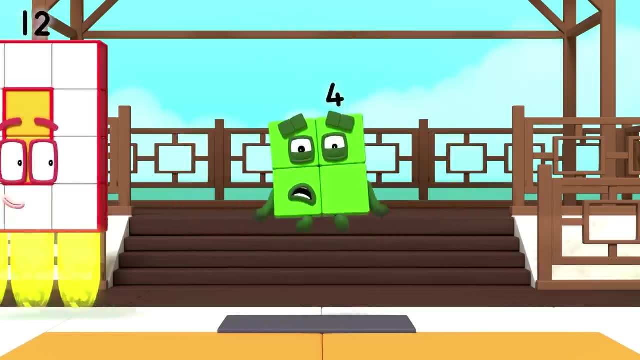 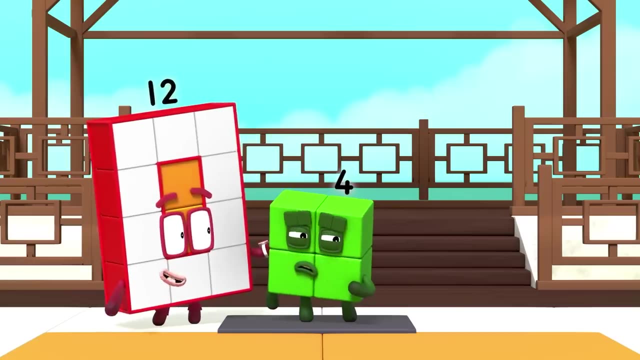 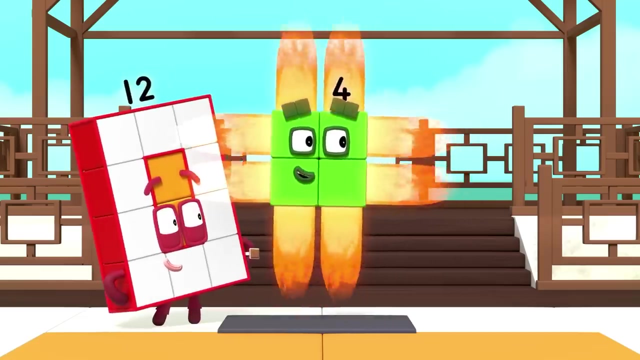 Am two by two and I am also turn Two by two. that's the same again. Oh, did I go wrong? No four, you're a special kind of rectangle That is the same number of blocks wide as tall. a square, A square, A square. Oh, 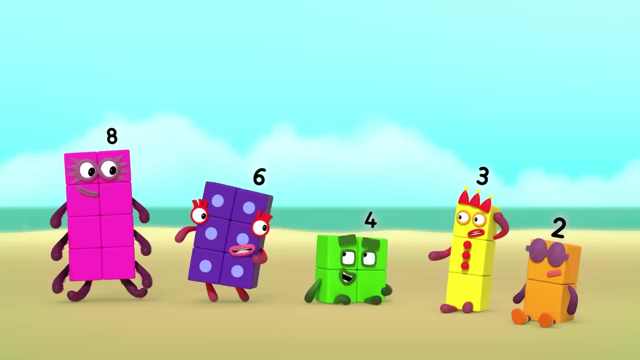 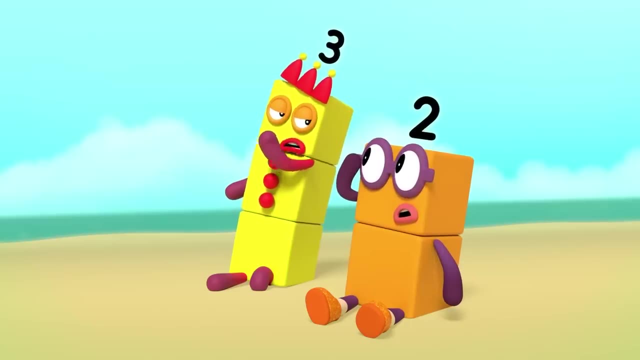 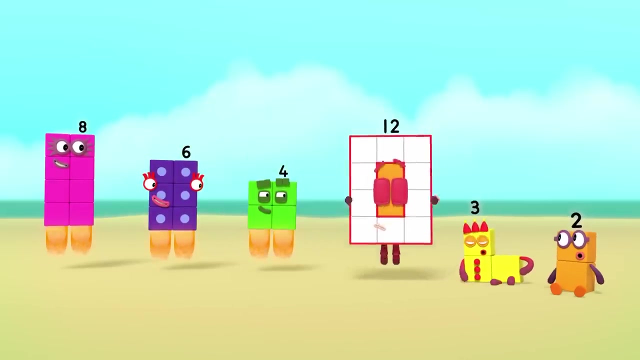 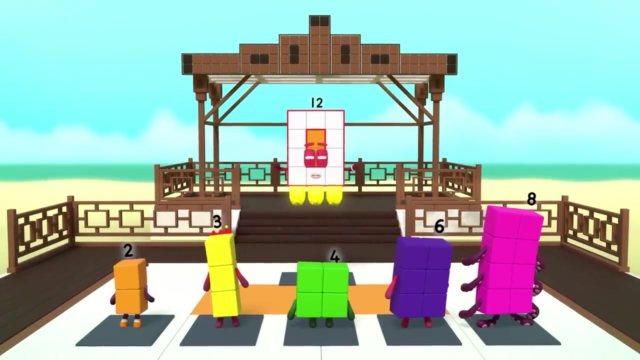 Hey, hey, hey. what's all this? look at us and be amazed. we all have rectangle rays. Oh, It's alright for some. I can't make big, wide rectangles. Whoever said rectangles had to be white Number blocks? stand tall. now what shape are you making? 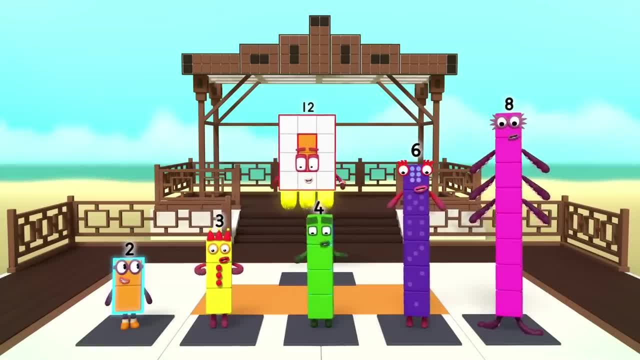 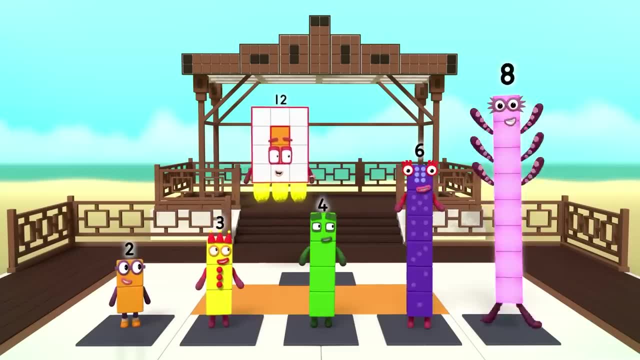 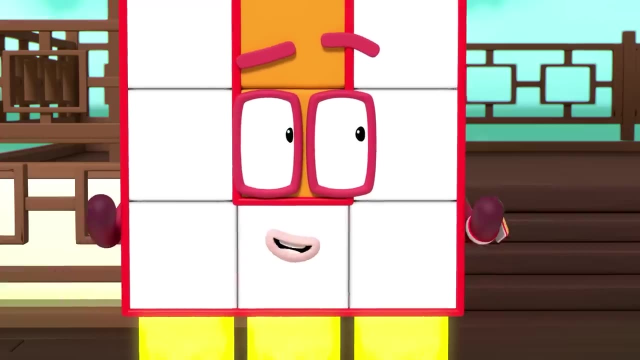 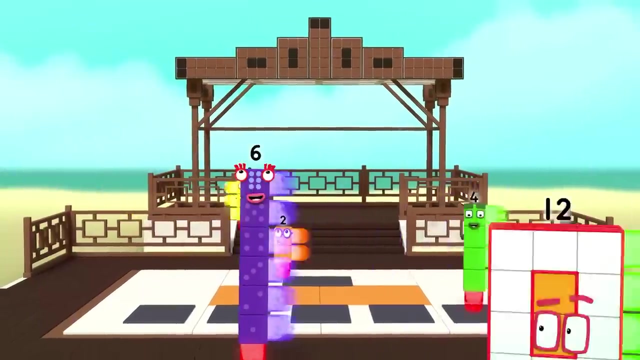 Rectangle, rectangle. I am one block wide and I am two, three, four, six, eight blocks tall. I am a rectangle. Maybe I shouldn't have told them. Whee, Oh well, too late now. Oh, Here it is. 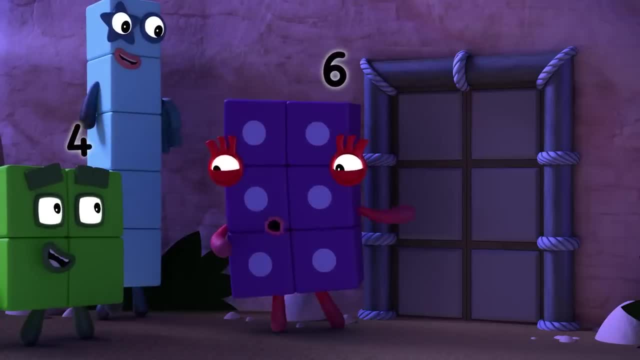 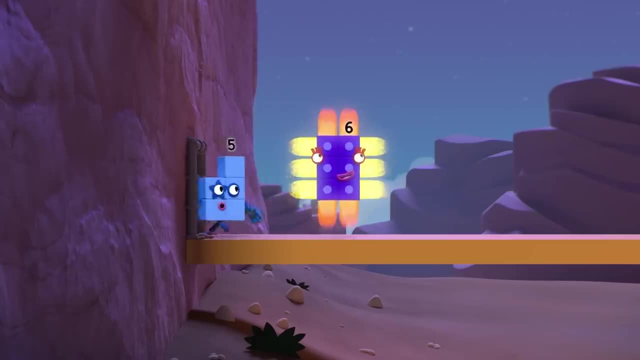 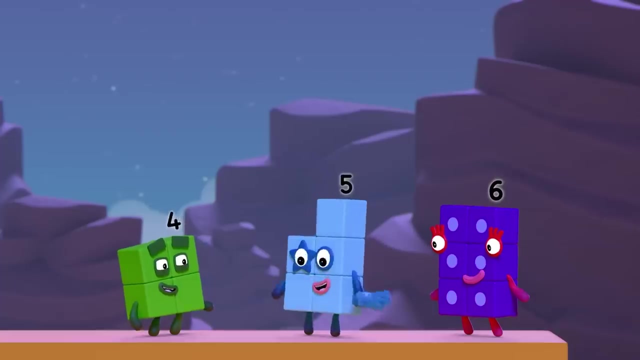 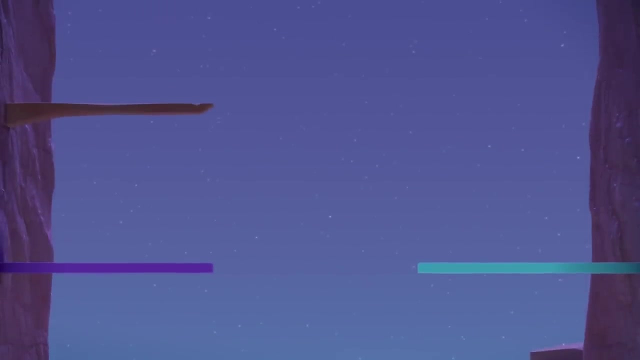 Right where Twelve told us The doors to Ray Canyon. I wonder why it's called Ray Canyon Rectangle. Ray Twelve said if one of you can get to the top, you'll find a big surprise. Yes, we knew, But how? 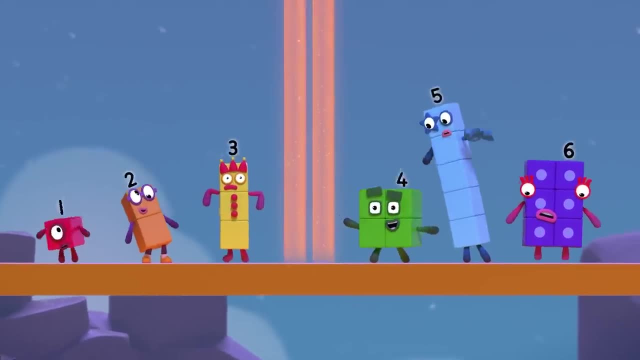 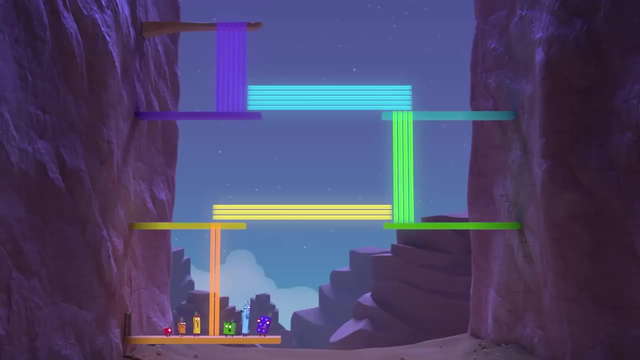 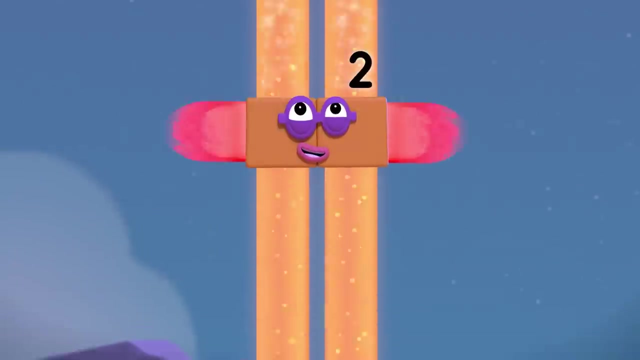 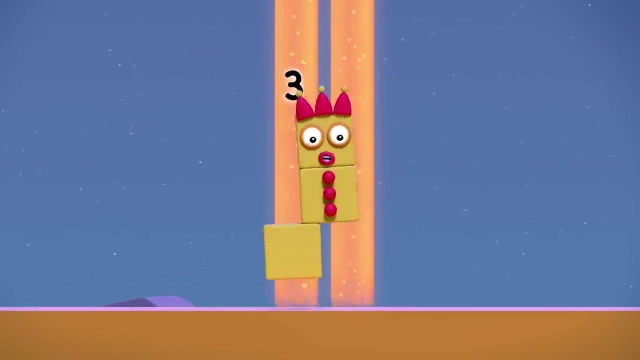 It's too far to jump. Ride the rays. Ooh, How do we ride them? These are two rays, So maybe Whoa Whee Come up. It's fun. Oh, that's no use. I can't make a rectangle. 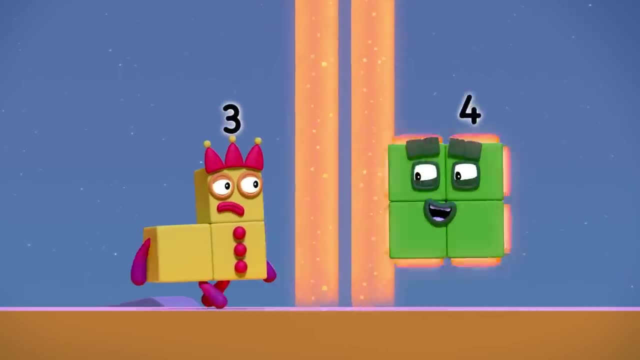 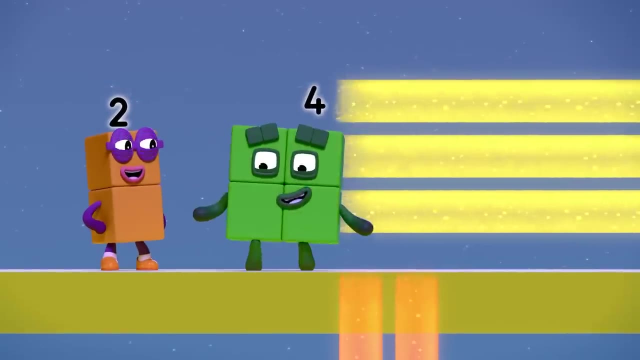 It's too blocky. Can you make a box wide? No, but I can. I'm a two-by-two square. Whee, Yay. If you think that ride is smooth, wait till you check out this move, Ooh. 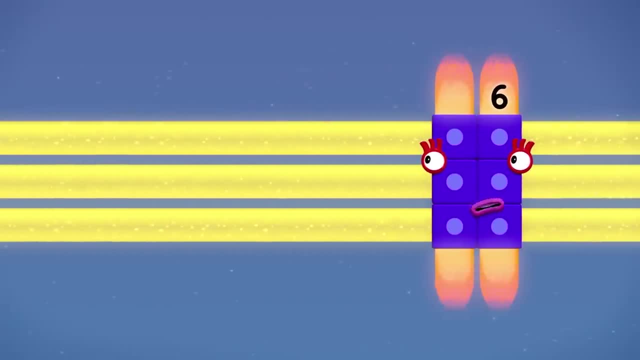 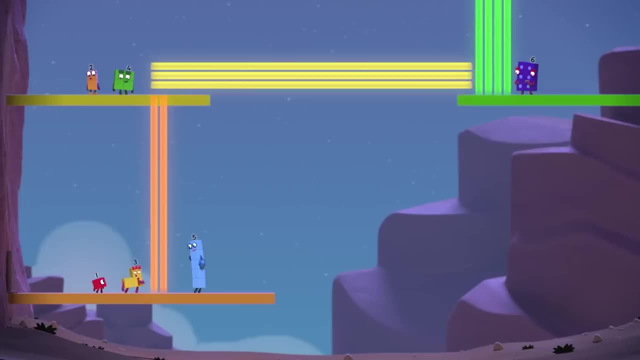 Wow, I'm two, lots of three. I've got two rays and three rays, Ha-ha. Aw, I've got three rays too. you know, I could ride across Just like six if I could get up there, Pfft. 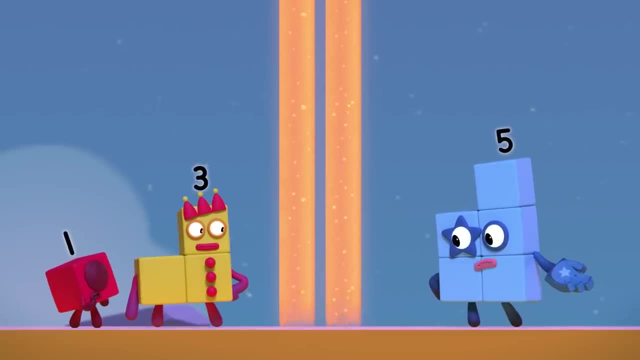 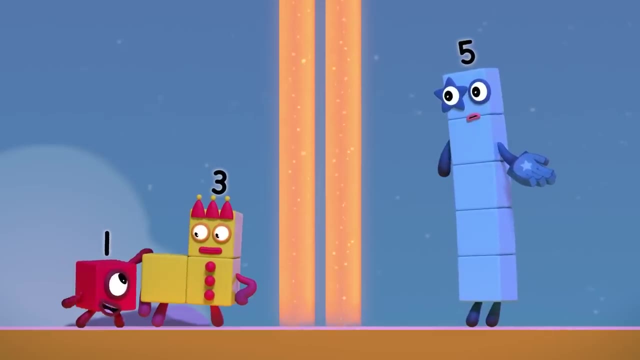 Odd numbers like us just can't make a rectangle that's two blocks wide. Twelve said only one of us had to get to the top. remember, We can all work together to find a way. I don't see how We're out of luck. 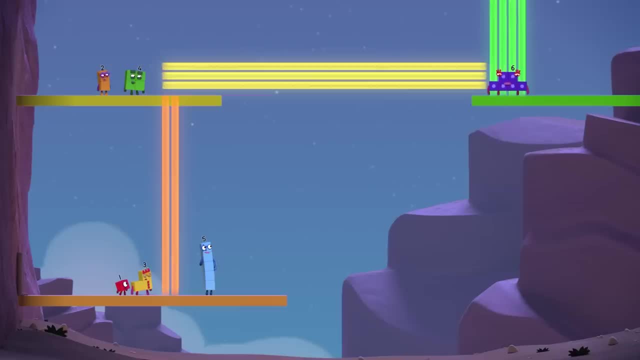 I can't make four blocks wide. I'm stuck. I can, I can, But I'm stuck here. We're all stuck. Twelve must have made him stuck. I'm stuck, I'm stuck, I'm stuck, I'll get back. 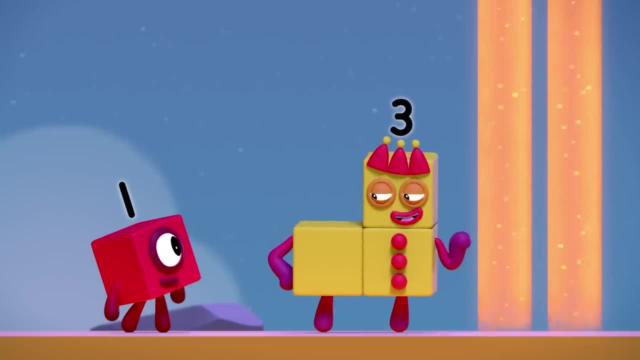 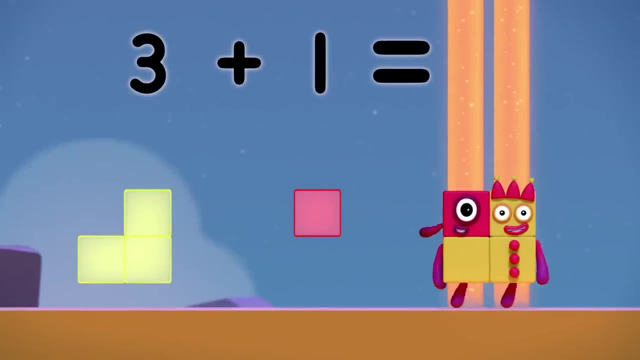 Come one with me, I'm stuck. Ah No, You can't be surprised. Don't be around me, I'm stuck. Come on, I don't want to lose, I'm stuck. Yeah, you're not getting anywhere. 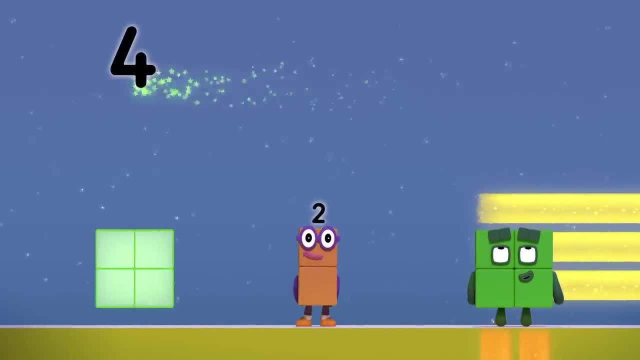 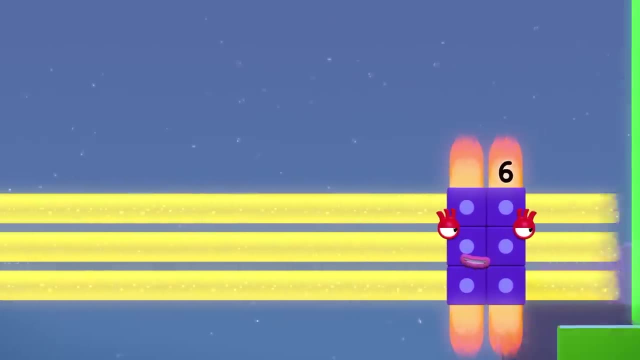 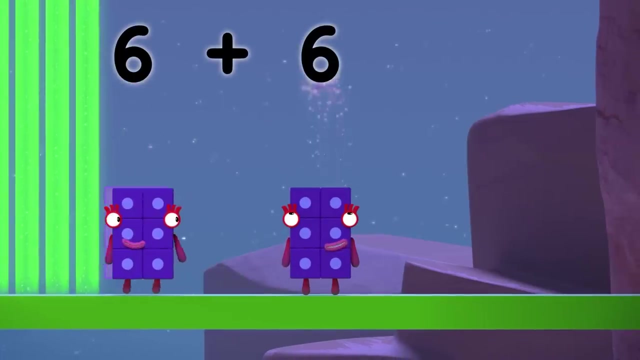 Lots of smooshed foes And I'm stuck. Pff, Oh, Come on you, I'm stuck. Aha, Huh, Six plus six equals Twelve. Oh, well done. Who came up with this idea? 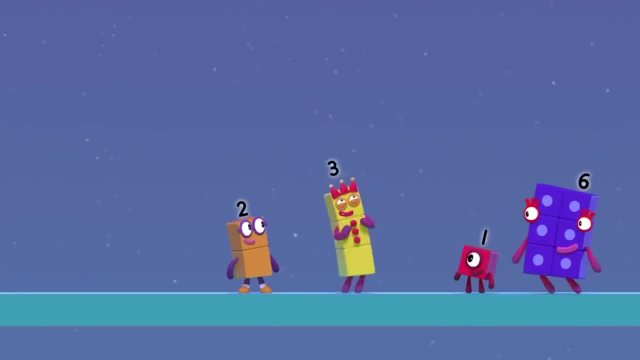 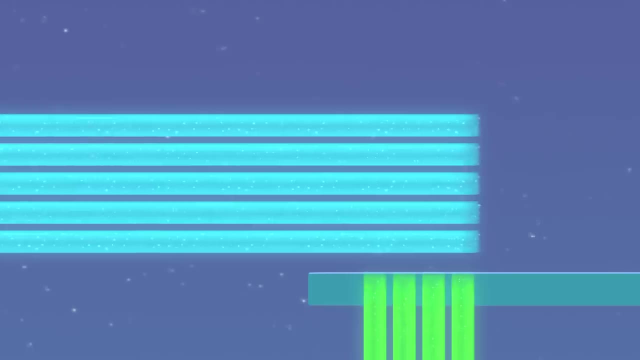 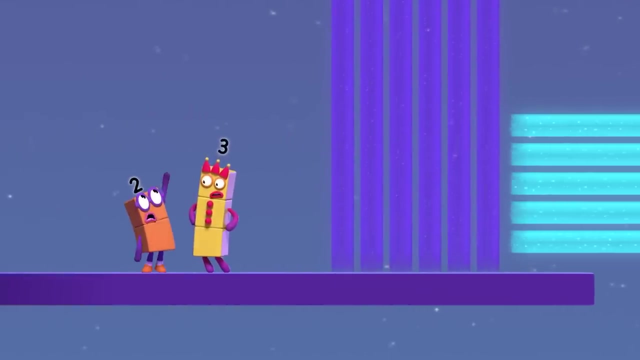 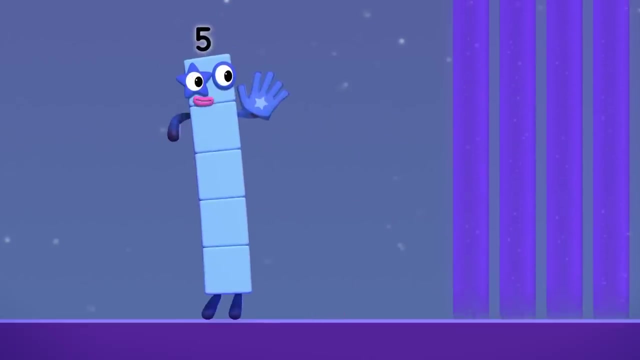 Me, me, me. Three plus two equals Five. Hurray, Yeah, Um, but how do we get up there? We can't make any progress. We can't make anything. that's six blocks wide. We've only got five blocks between us. 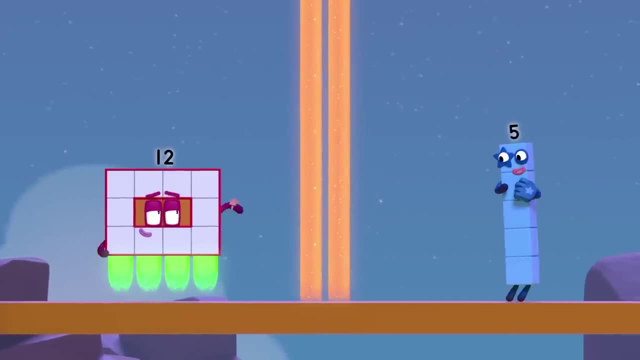 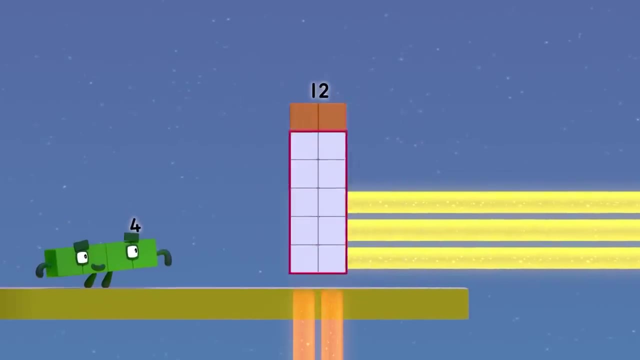 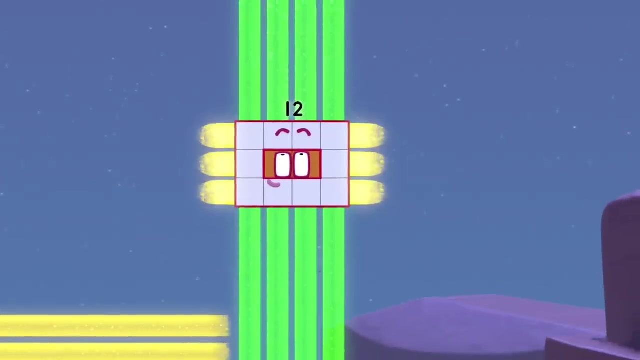 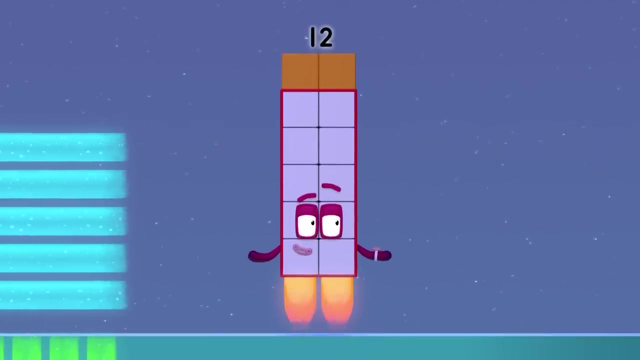 Hello, my friends. Twelve Switch. Congratulations on getting so far. Switch. Oh, By working together you've nearly reached the top. What a super rectangle. But not even I can make every size of rectangle. I can't make a rectangle that's five blocks tall. See, 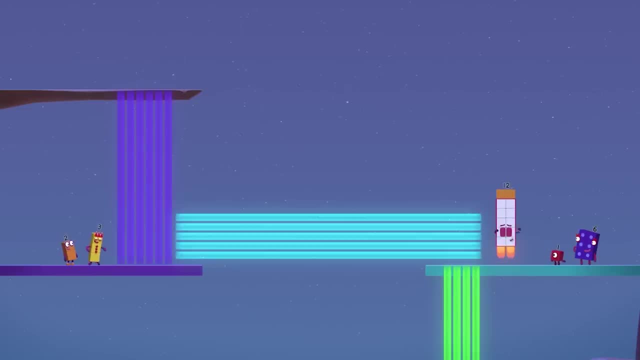 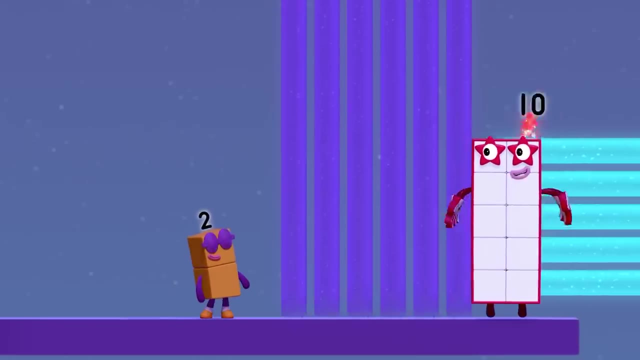 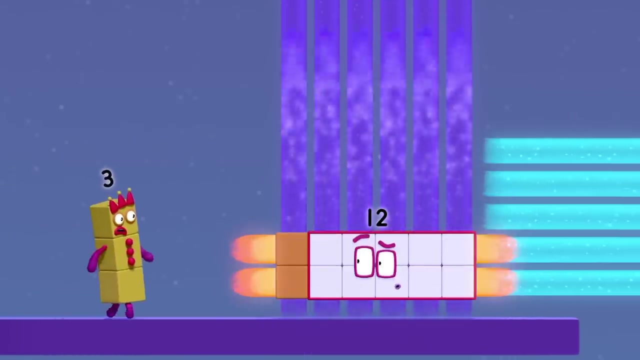 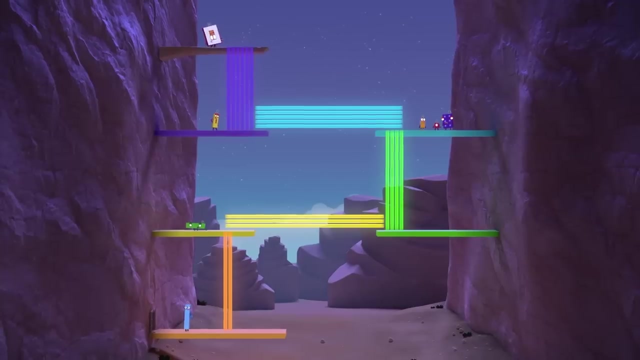 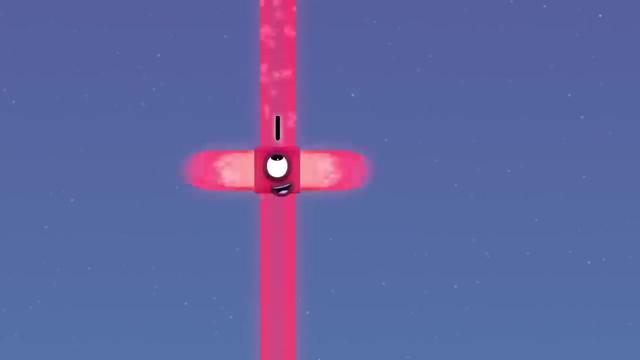 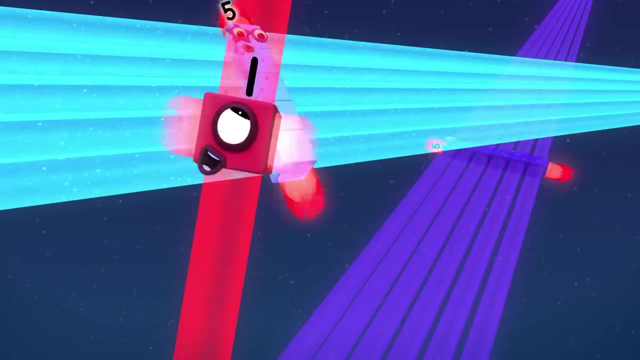 But, like you said, Three. sometimes there's more than one way to solve a problem. Twelve is ten plus two. Ten plus two equals Twelve Ten. I'll drop you a line. What does that mean? Welcome to the racetrack. 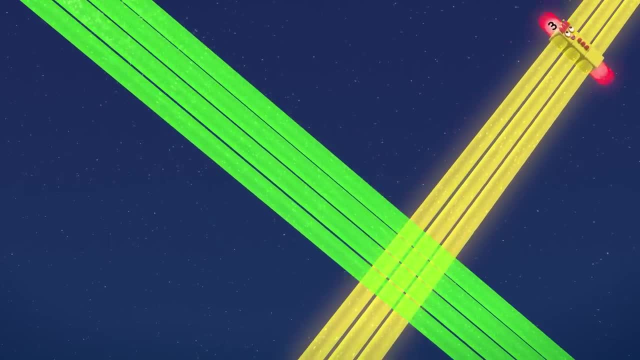 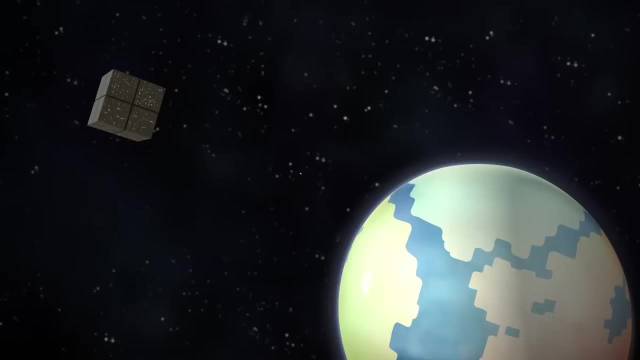 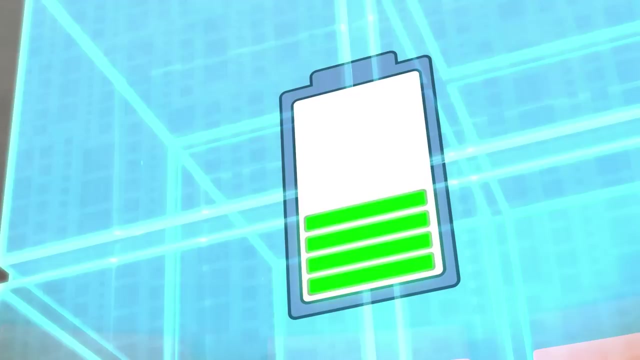 What do you think? I love it. Woo-hoo-hoo, Come in number basis. I'm in position and heading for the Block Star, Careful Twelve. The Block Star's battery is running out. You need to change it before the whole thing drops out of the sky. 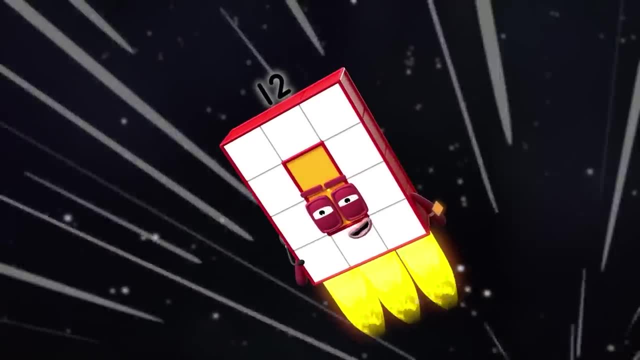 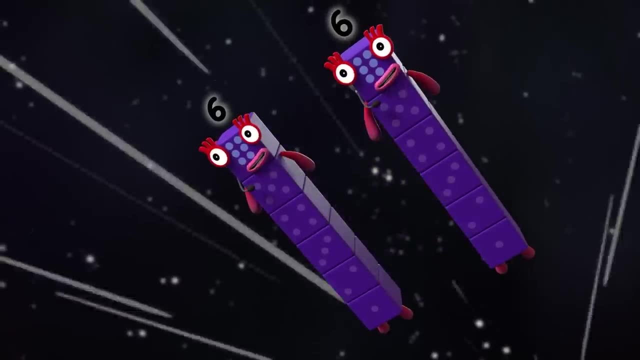 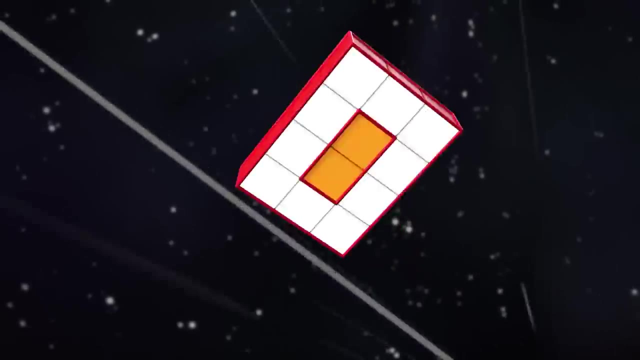 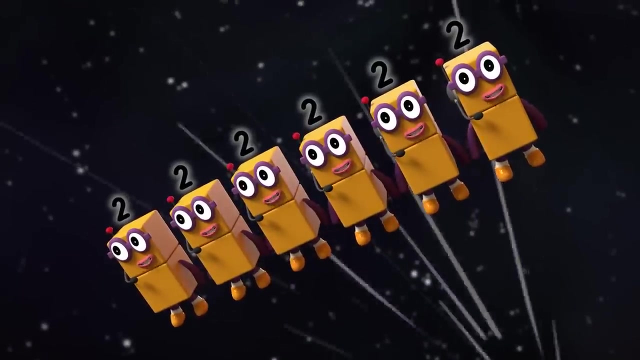 and smashes into Numberland. That block is no match for a super rectangle like me. All teams report in Switch Two: sixes standing by. Switch Three: fours Standing by. Turn Squad 3, standing by. Switch 6-2, standing by. 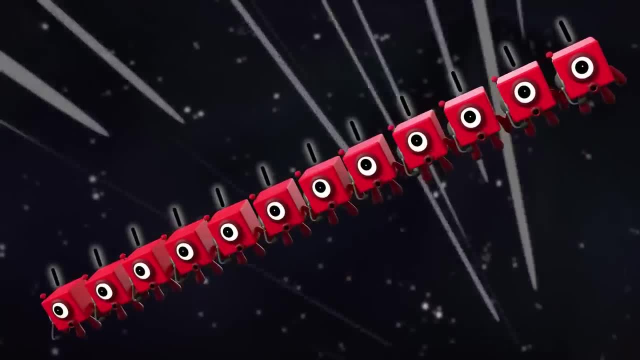 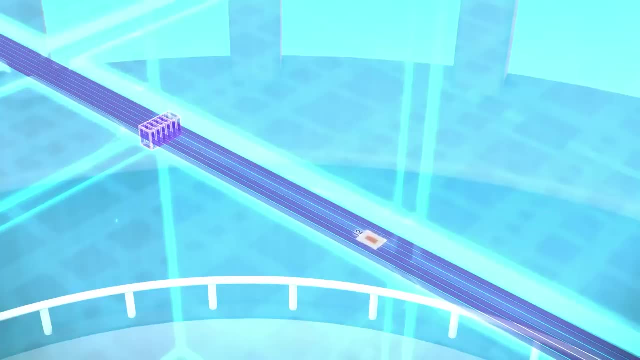 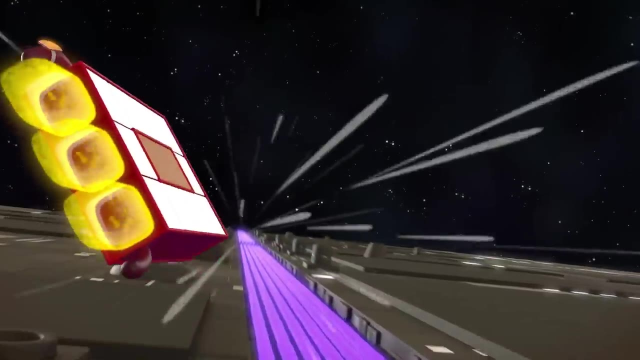 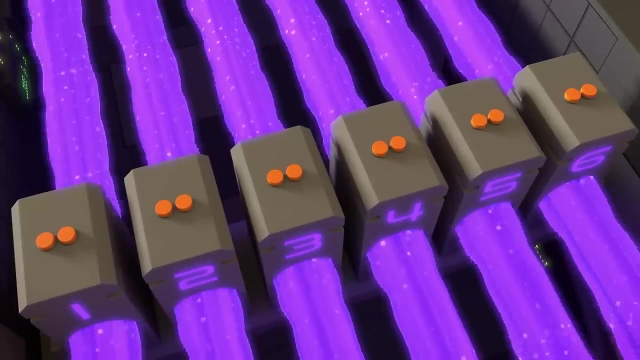 Switch 12-1, standing by. Switch, I'm going in. Hold on tight. You need to turn off the force field before you can get to the battery. Can you see a line of towers ahead? Yes, six of them. Each has two buttons on top. 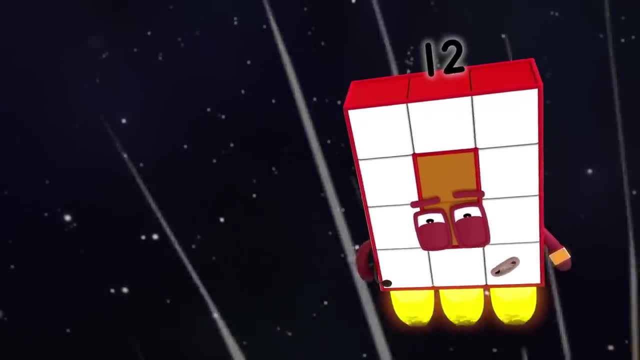 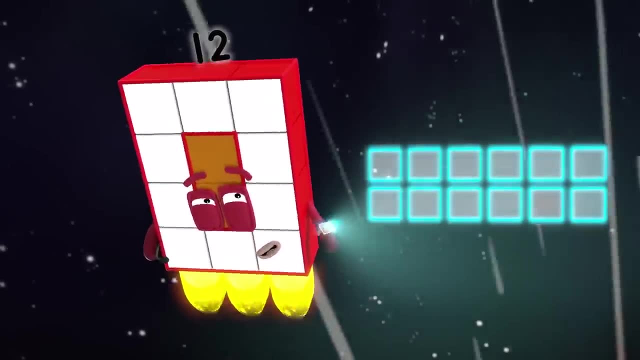 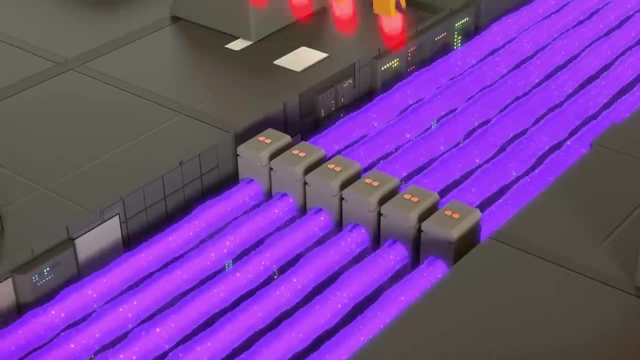 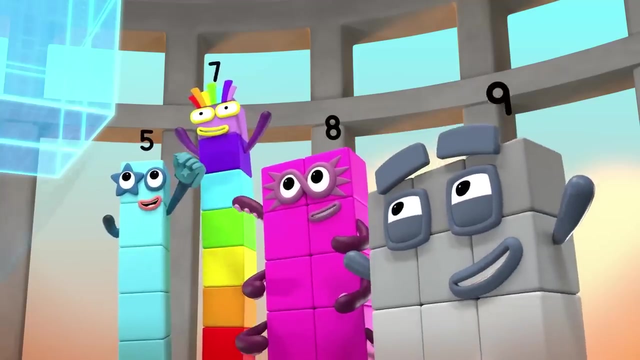 You need to press all the buttons together. Six towers, two buttons each Array display. This calls for switch Wee 6-2 Switch. Hello, Yes, You've done it. 12!. Now head for that battery. There's no time to lose. 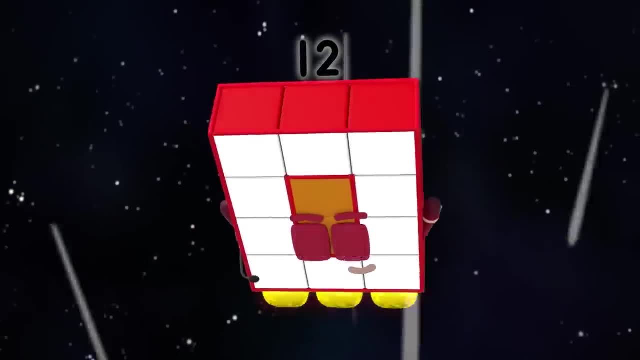 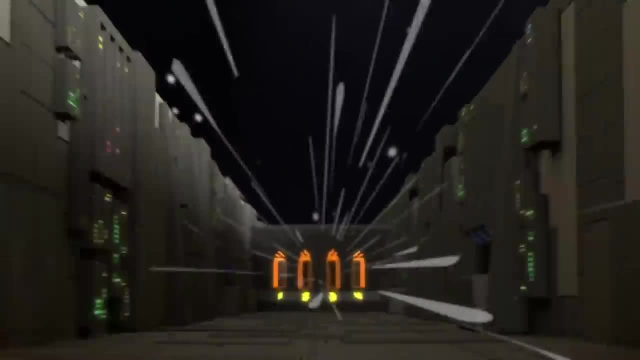 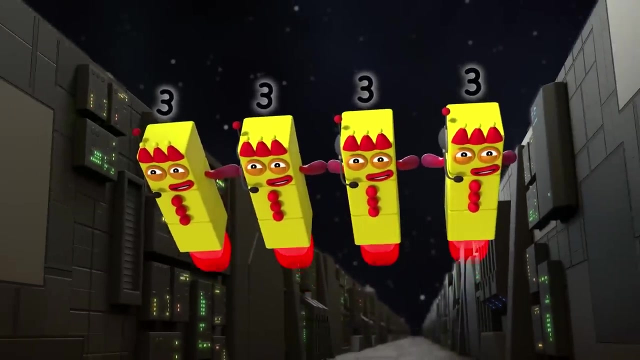 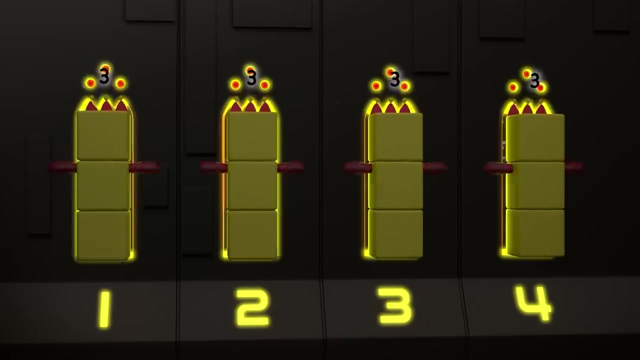 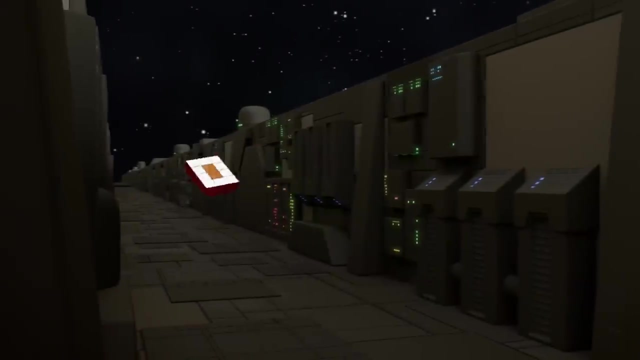 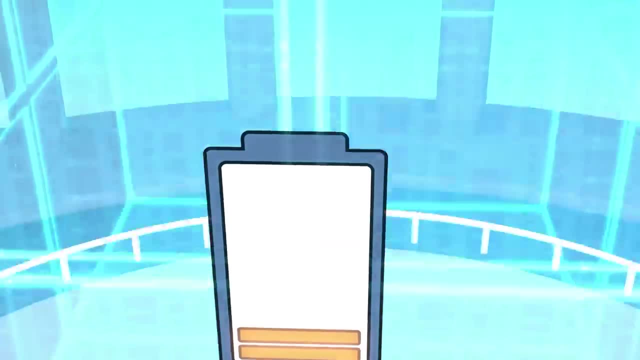 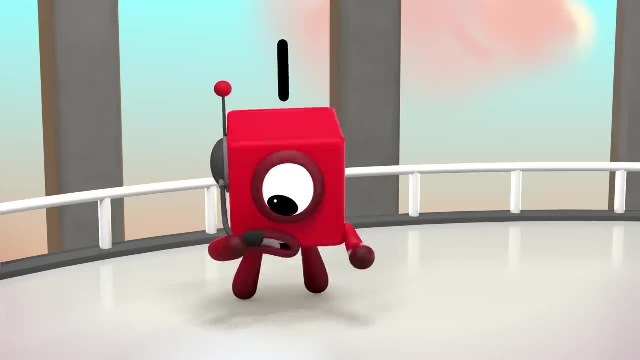 Yuck Oop, Ah. Those block ships have gone haywire. It must be the low battery. don't let them slow you down. Hup Hoo, Oh, Oh, I think it's dead. Oh wait, it's Blake, I've got just the team. 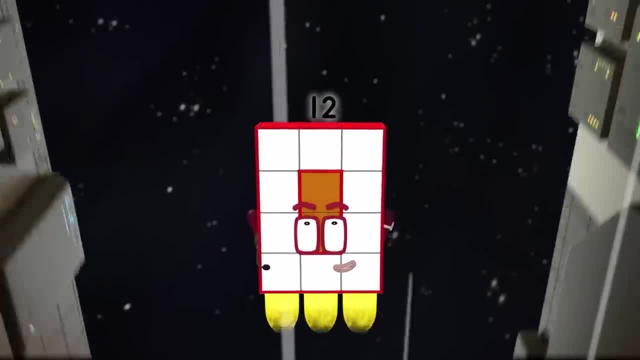 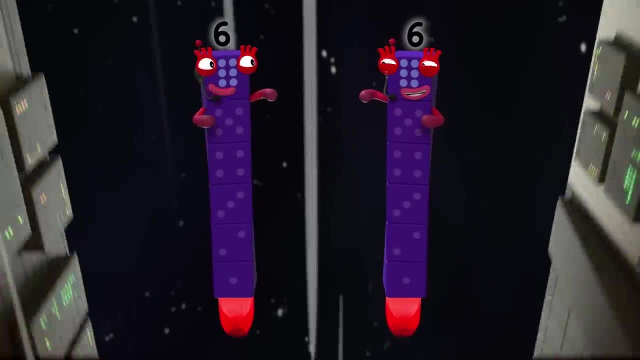 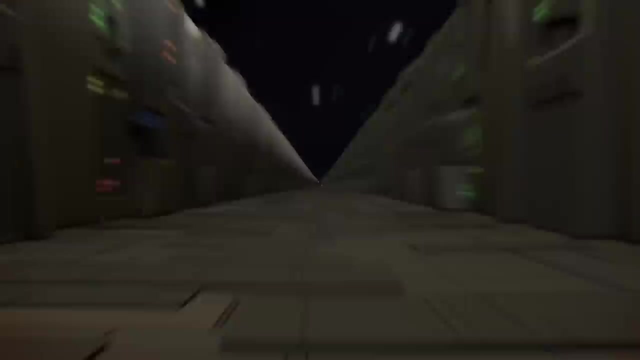 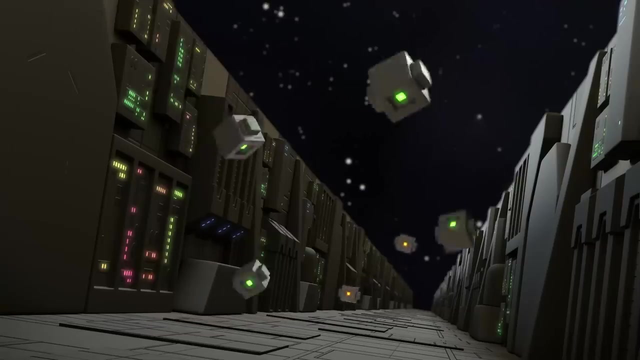 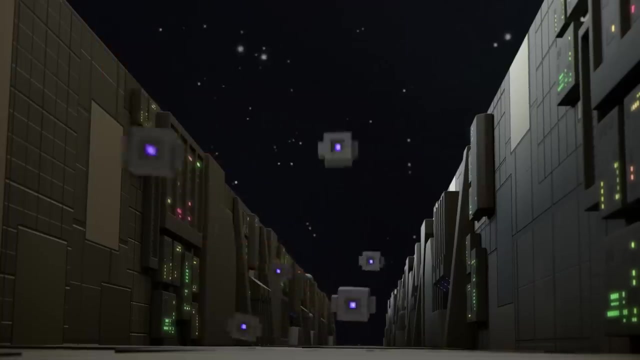 Switch Two sixes. We've got a great escape technique. Let's play a game of hide and seek Switch. Catch me if you can. Whoa, I've got a bad feeling about this. A razor's blade Long and low. 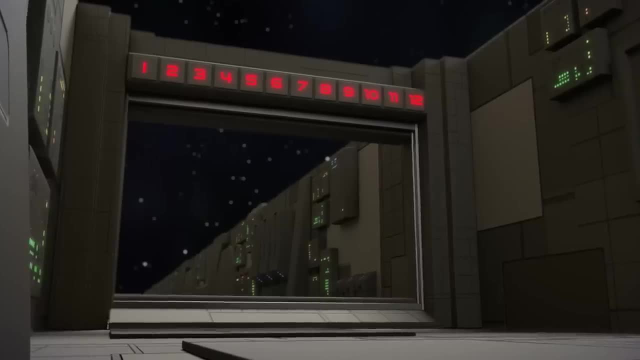 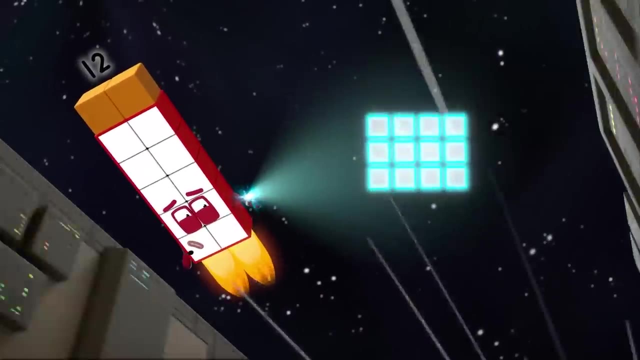 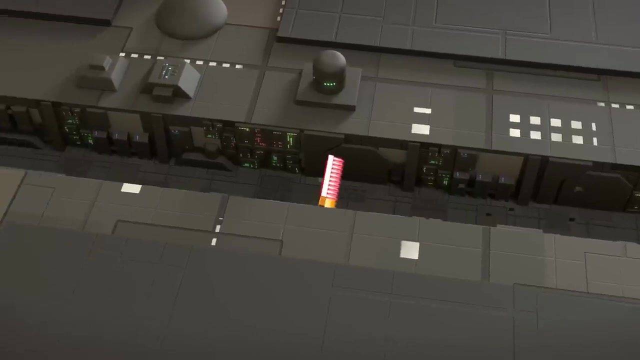 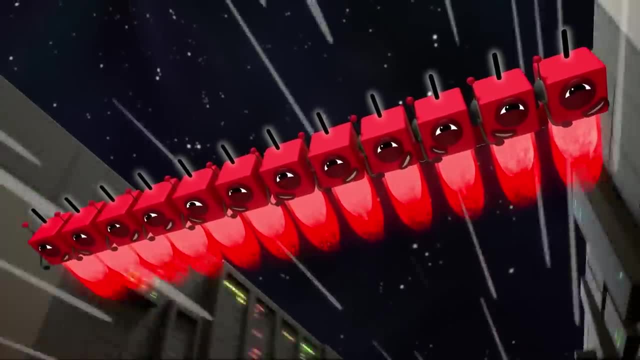 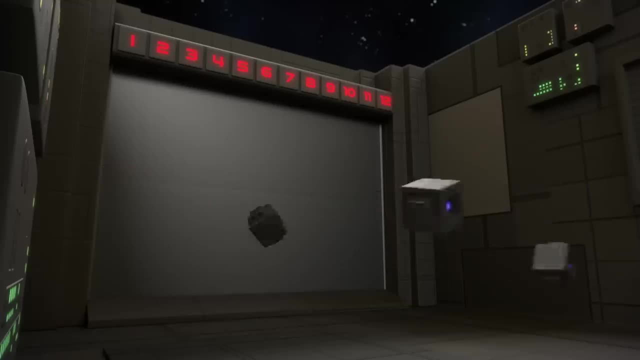 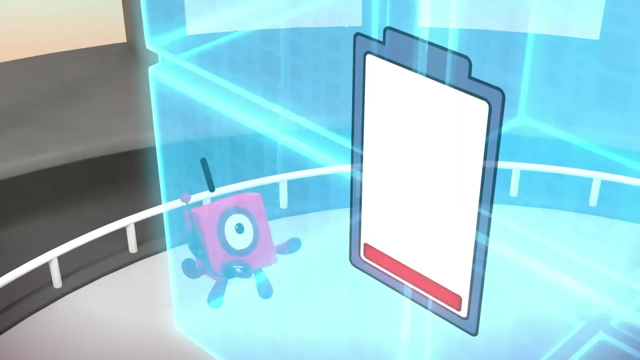 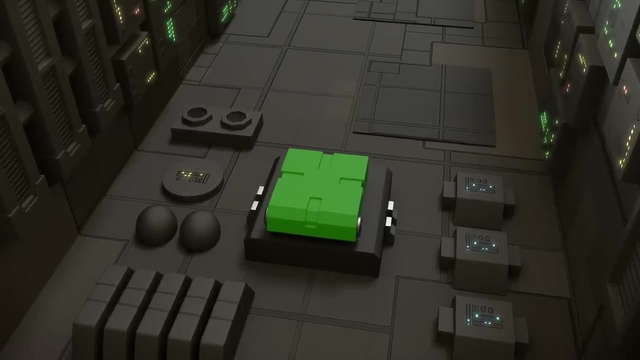 Oh no, Oh no, Oh no, girl, 12 ones. Whoa, Battery level almost dead, but you're right on top of it. You need to open the cover, take out the old battery, then put in a new one as fast as you can. 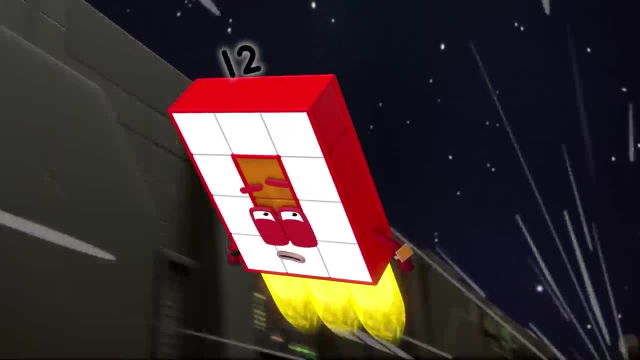 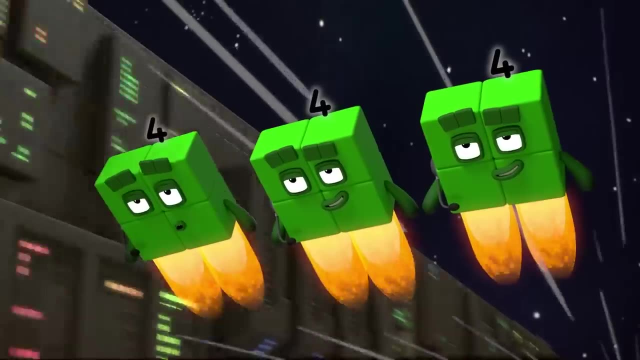 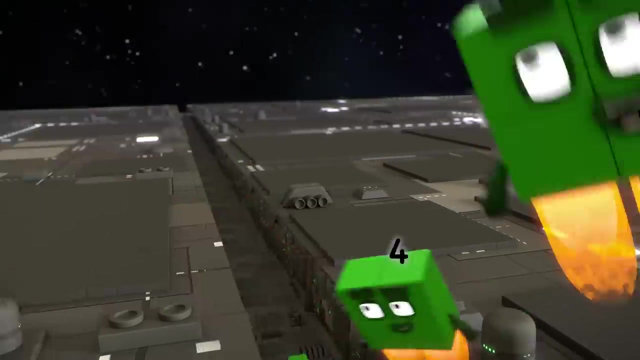 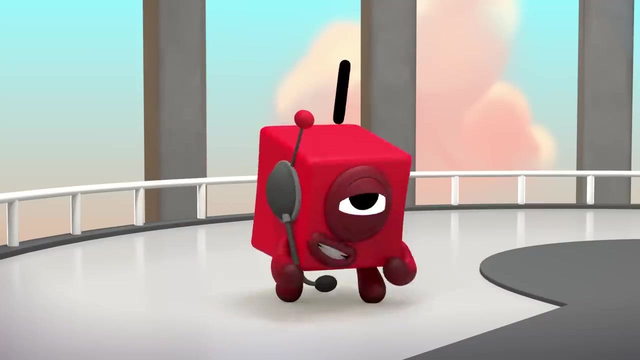 Phew, that's three different tasks, But I can do them all if I use the four. This is it Target approaching One, two, three, four. Yay, You did it. Now witness the power of this fully operational disco cube. 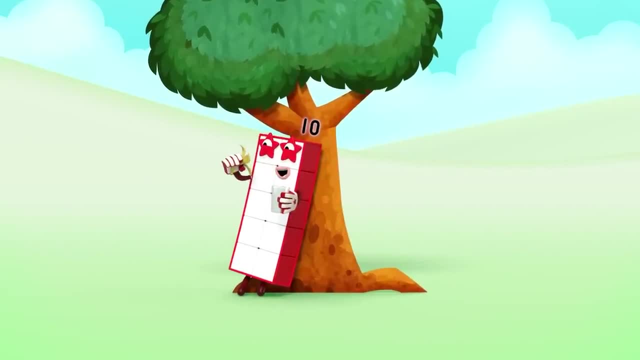 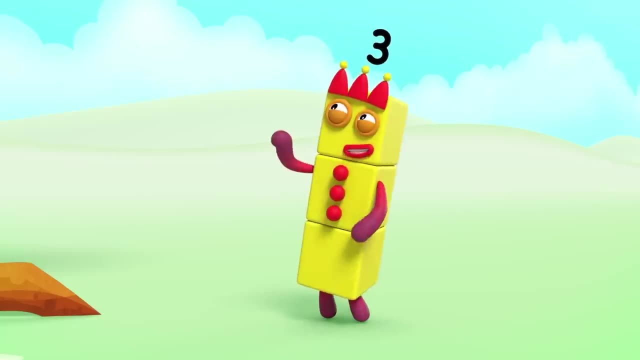 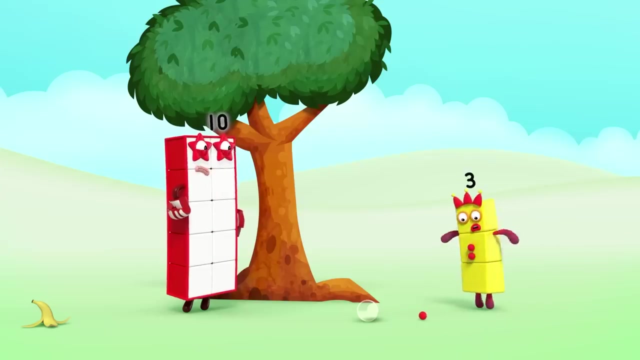 BAM, BAM, BAM. Three, Oh sorry, Ten. I'm just so excited to show you my new trick. Look at this. Oh, Is that it? No wait, I'm not having much luck with mine today, Oh no. 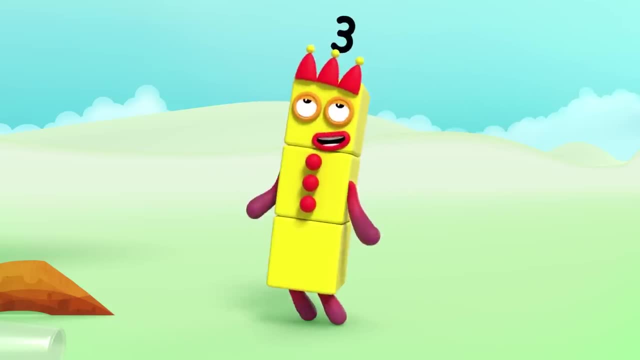 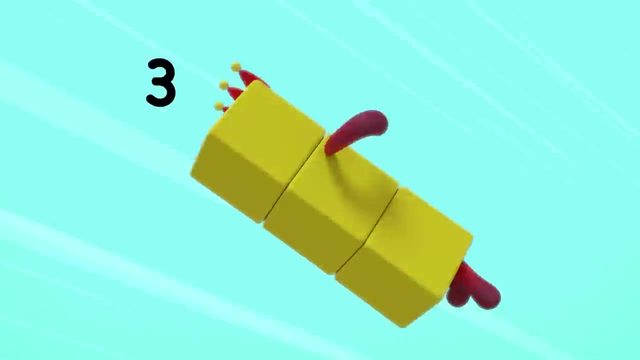 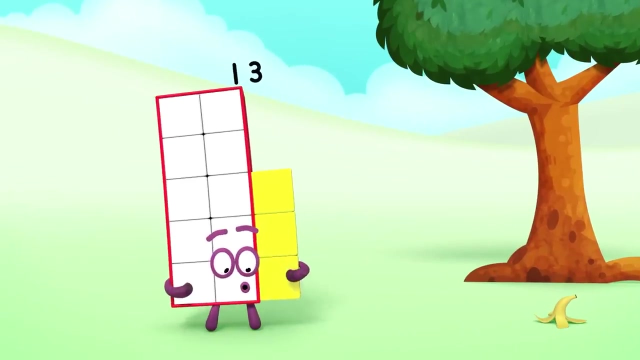 My new trick: Ready set go. Ready set go, Steady go, Oh unlucky, Oh Hi, Who am I? I'm one, two, three, four, five, six, seven, eight, nine, ten, eleven, twelve, thirteen. 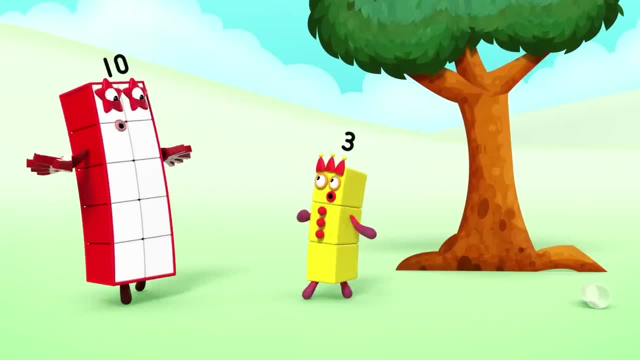 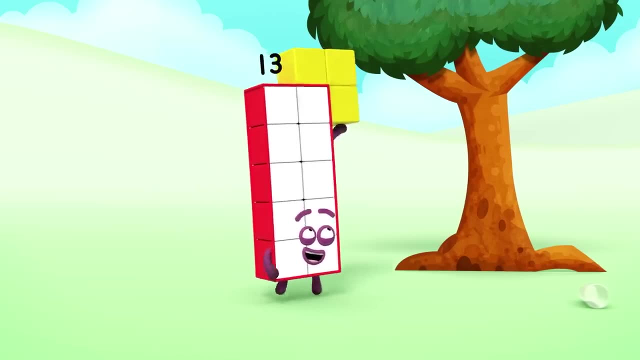 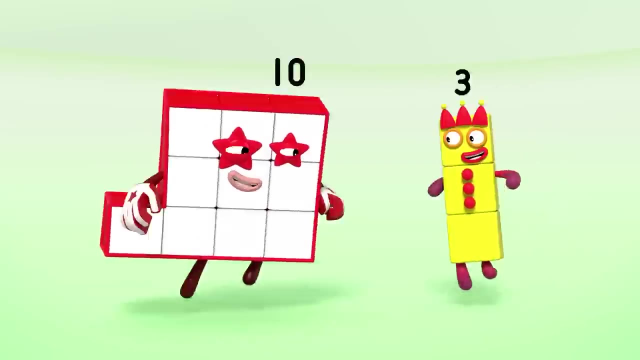 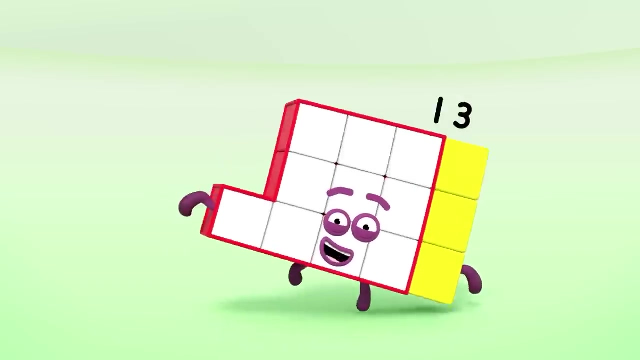 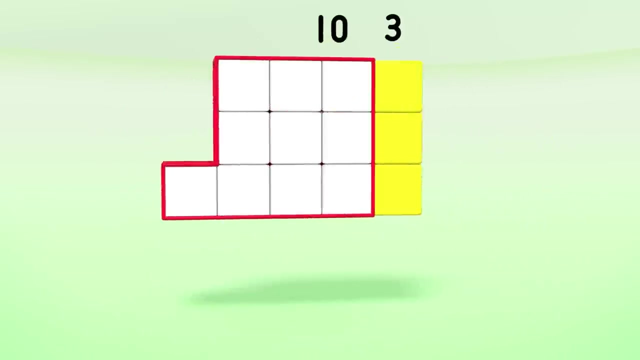 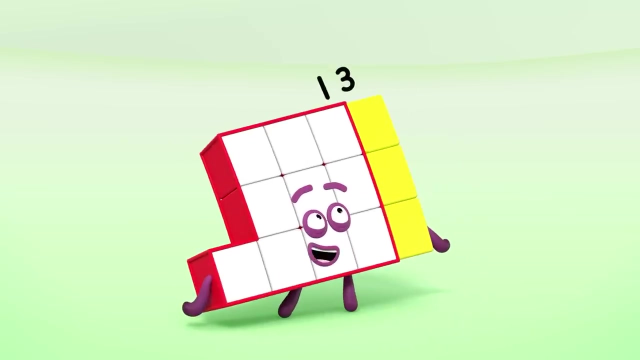 Whoa Wow, My three fell off. Never mind, I am thirteen. Oh, whoa Ha, Unlucky. Try again. I am thirteen, Hooray, And I think I might be a little bit unlucky. This is me. 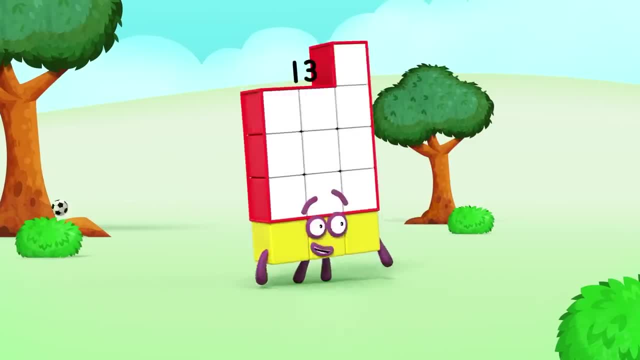 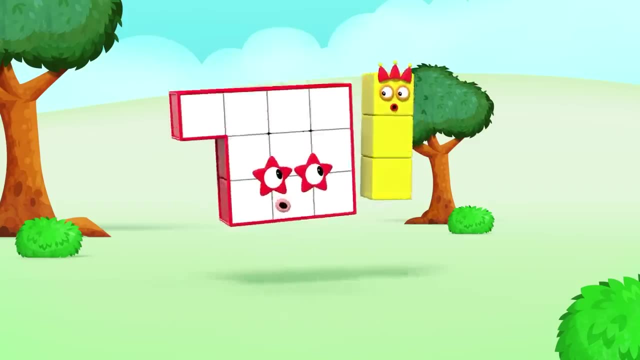 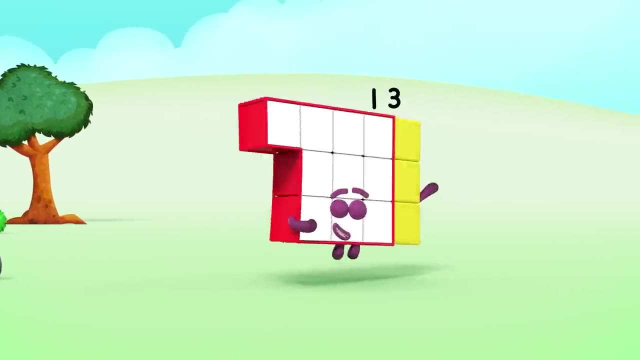 Ten and three Expecting to run out of luck. Sorry, It's all jolly japes. when I get into scrapes I'm always coming unstuck. Oh, I'm the clumsiest number you've ever seen. Unlucky. 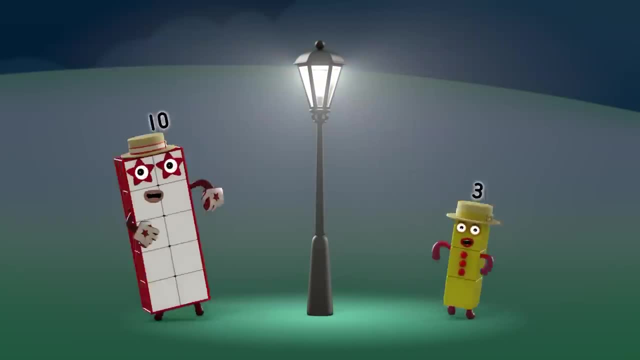 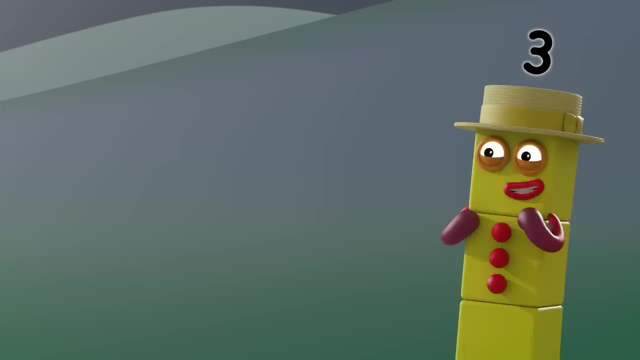 Number thirteen. Oh, A three and a ten. Somebody should tell him that it's happened again. I don't have the heart to be fussy or picky, But he's falling apart. He's a bit unsticky. It's happened again. 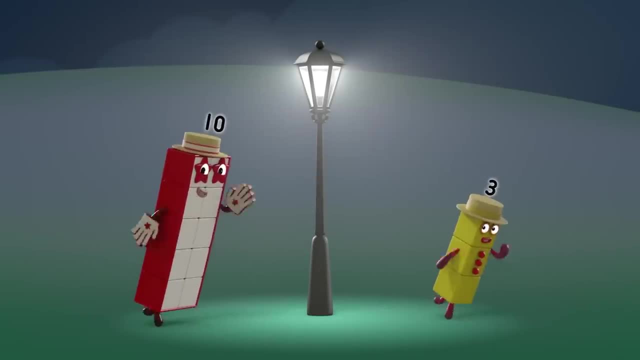 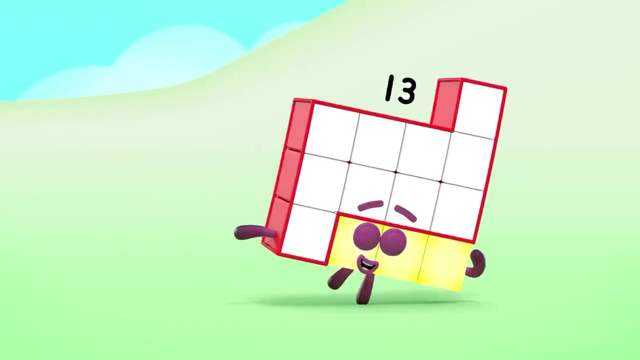 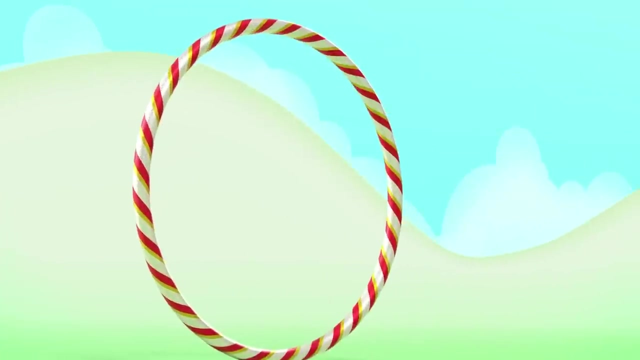 And no one knows when, Somebody should tell him that it's happened again. Me again. Three and ten Expecting to fall down a hole. Ha, I jump through a hoop And step in the puddle. That seems to sum up my role. 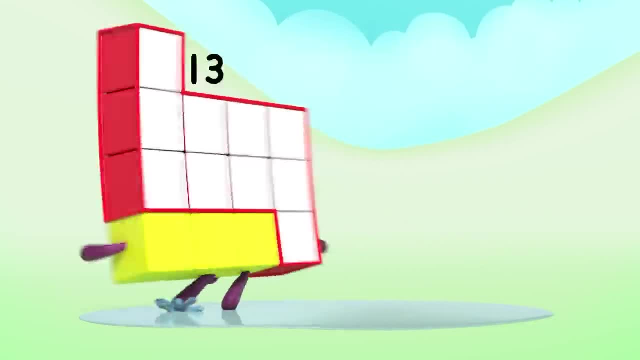 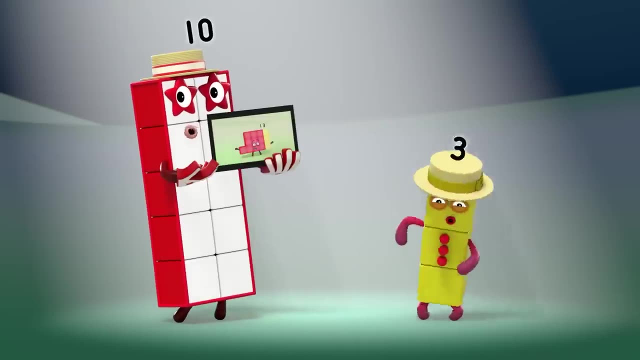 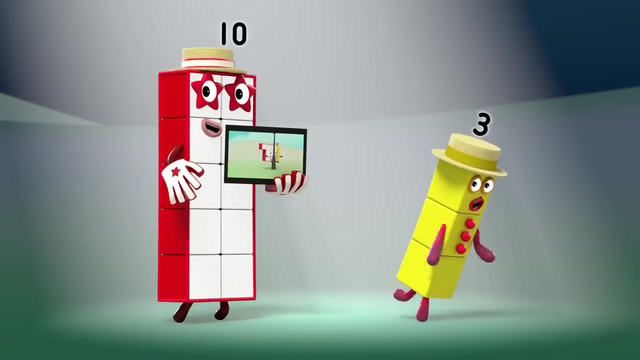 And wherever I end up, I might get slain. Unlucky Number thirteen. Oh, It's always the same when he says his name. Somebody should tell him that's the name of the game. It's happened before. A total disaster. 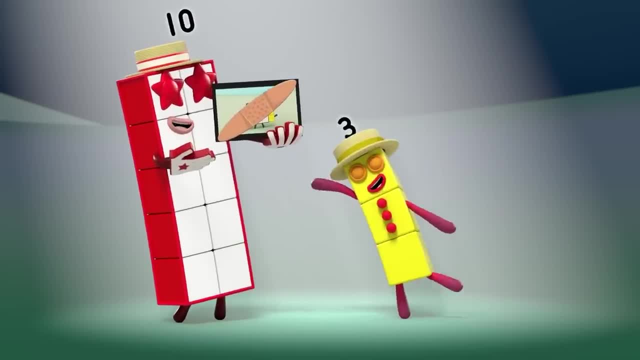 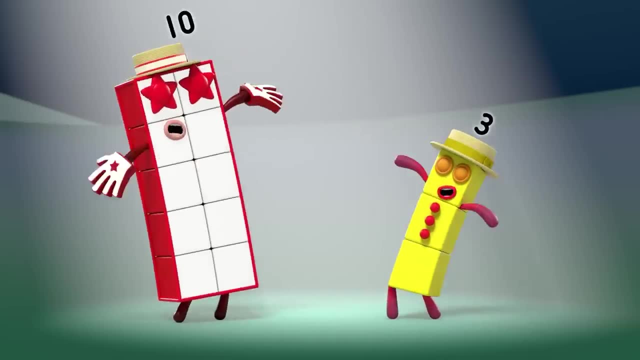 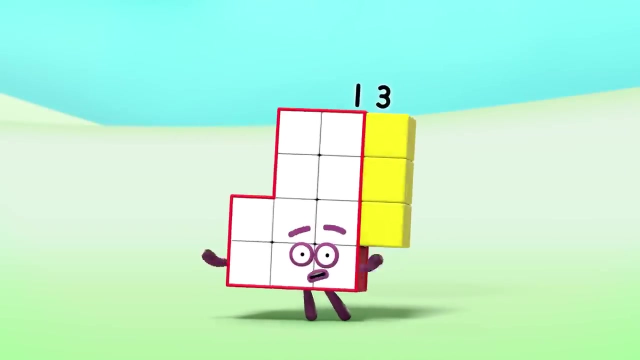 But he's going to need more than a sticking cluster. It's always the same. We know what to blame. Somebody should tell him not to mention his name. It's getting routine. I say: I'm thirteen, Keep it together. This is absurd.